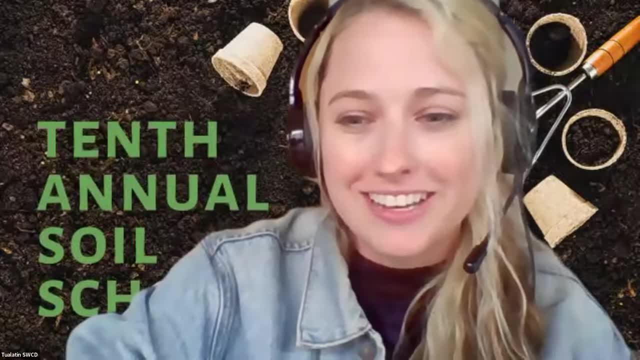 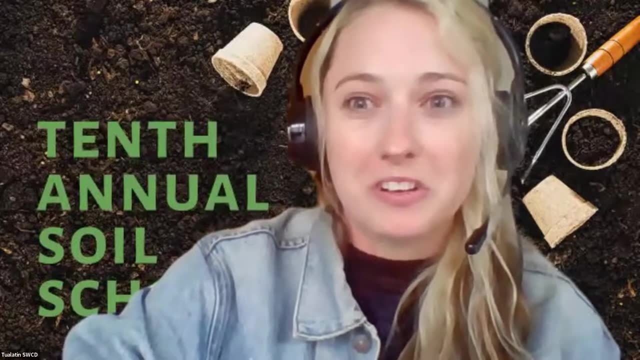 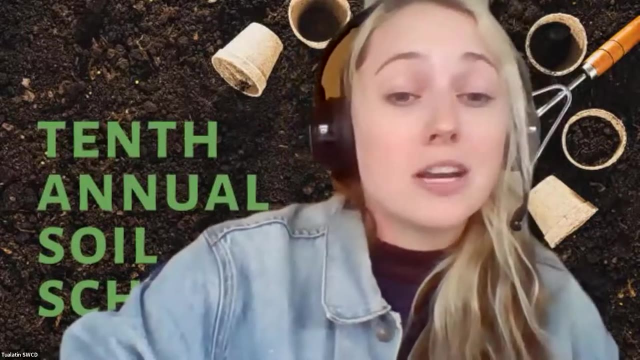 and I will be your host tonight for Soil School. We're about halfway through the series. I hope everyone has been enjoying the sessions. We really enjoy being here with you all tonight. So Tualatin Soil and Water Conservation District works to create a sustainable, productive and 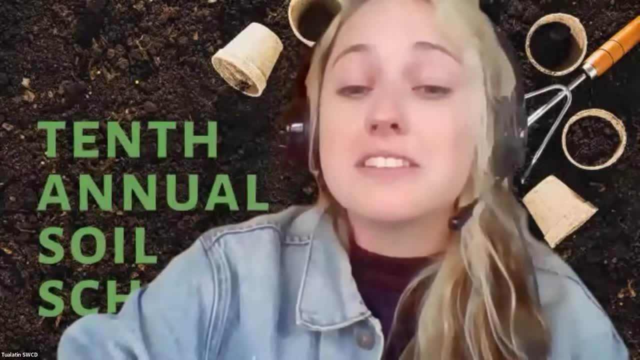 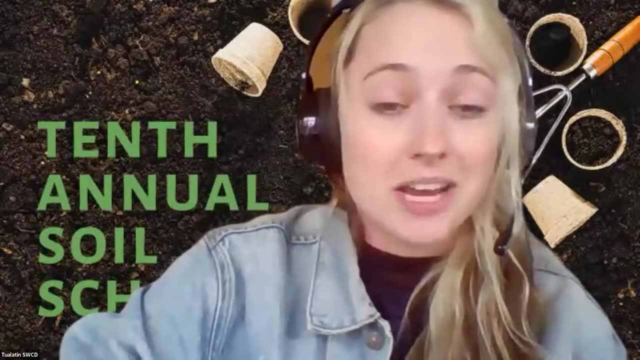 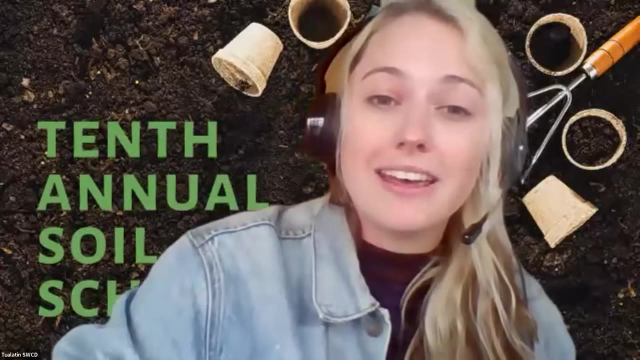 healthy environment for the Washington County community. We serve residents of the county by providing educational opportunities, advice about natural resource conservation and sometimes even financial assistance to help you get those projects on the ground. Tonight we're hosting this webinar. It's a series in partnership with West Multnomah Soil and Water Conservation District. 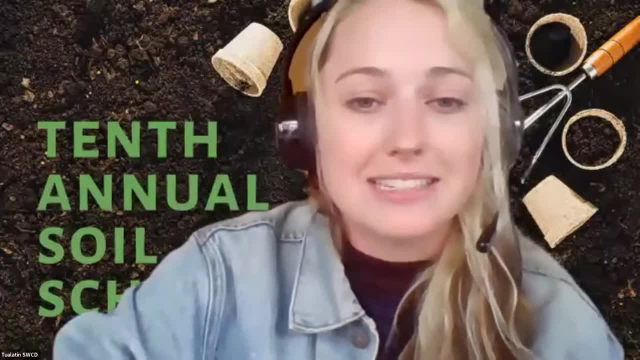 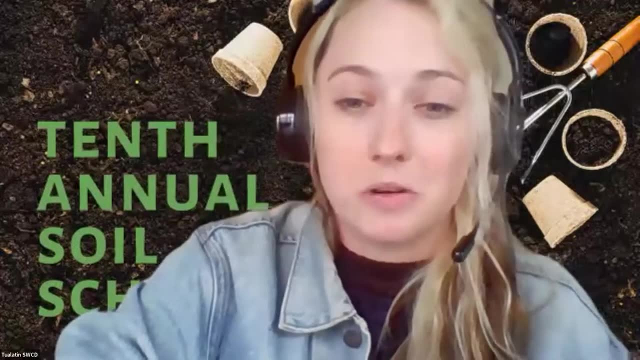 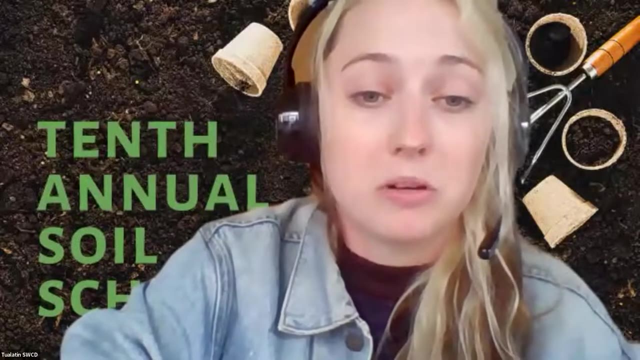 Their mission is to provide resources, information, expertise to inspire people to actively improve air and water quality, fish and wildlife habitat and soil health. They serve residents of Western Multnomah County, Salve Island and a portion of the Bonnie Slope neighborhood with conservation. 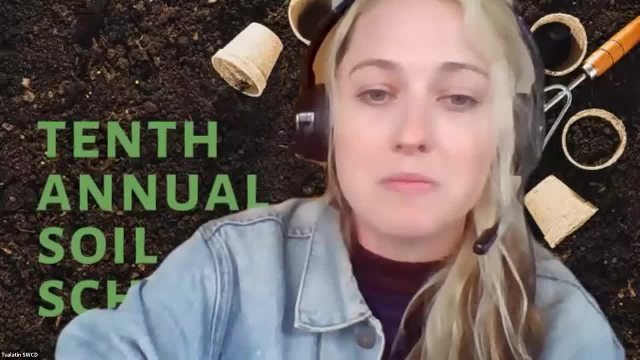 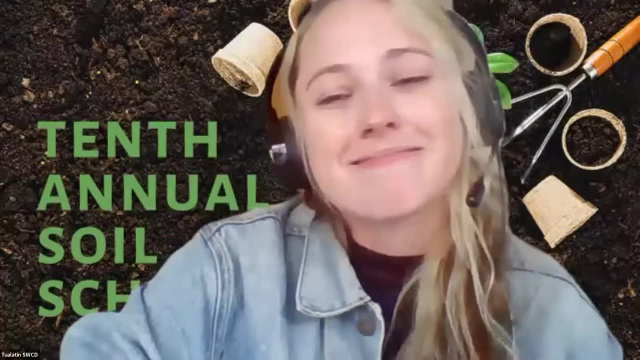 planning, weed management, native plants, wildlife, habitat restoration and a portion of the community gardens. So tonight we're here to talk about soil microbes. As we discuss this important topic, it's important for our district to acknowledge the original stewards, the indigenous. 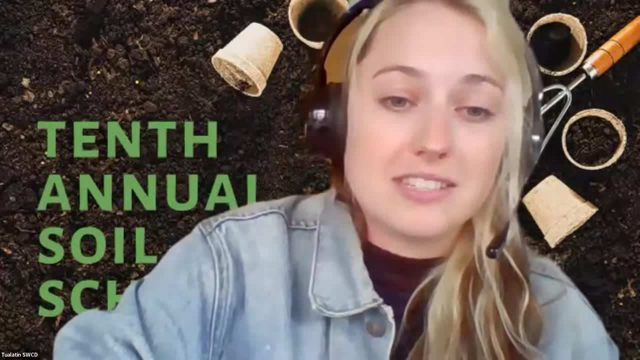 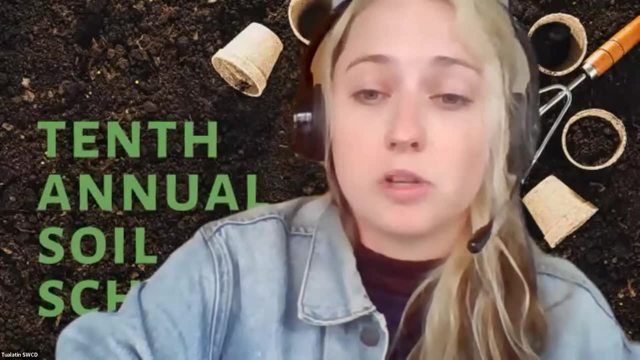 people of the land where we now provide conservation services and their deep and extensive knowledge of this land. We honor this land and its original inhabitants from time immemorable, the Tualatin Band of Kalakuya. They have lived and prospered by maintaining strong cultural ties to 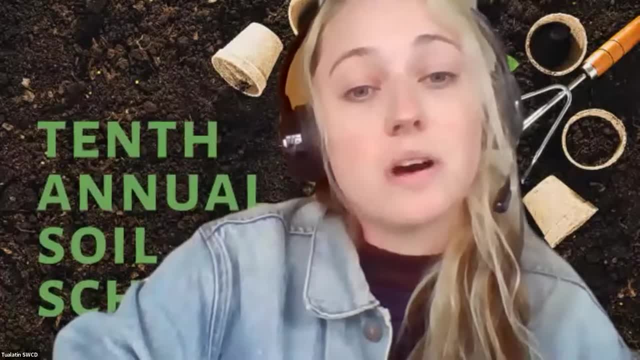 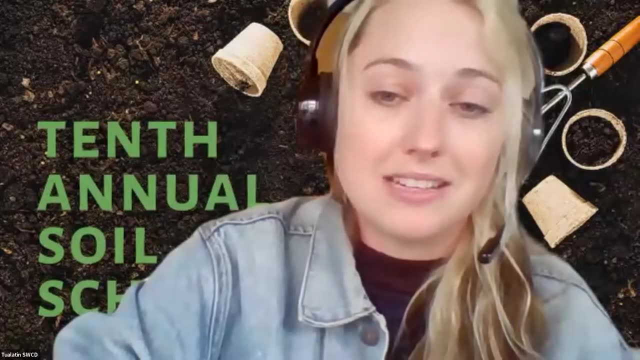 the land and through wise management of resources. The Tualatin Band of Kalakuya were signers of the Willamette Valley Treaty of 1855, which ceded their homelands to the United States in exchange for certain rights and benefits. 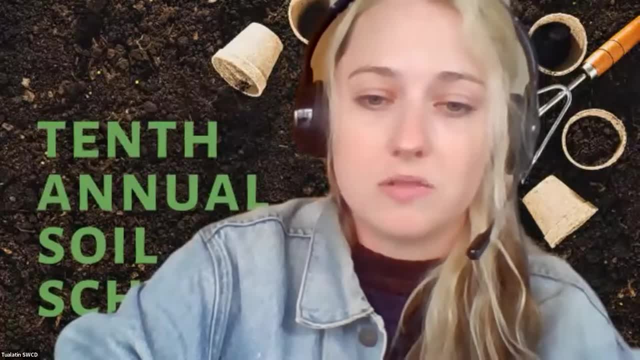 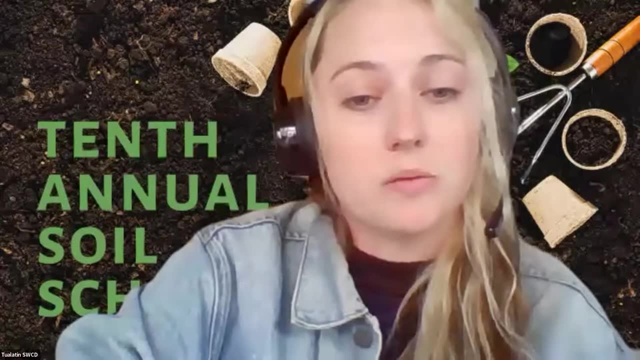 They were subsequently removed from their homelands to the Grand Ronde Indian Reservation, where they became members of the Confederated Tribes of Grand Ronde. Their descendants live on as tribal members today, carrying on the traditions and cultures of their ancestors, the original people of the land. 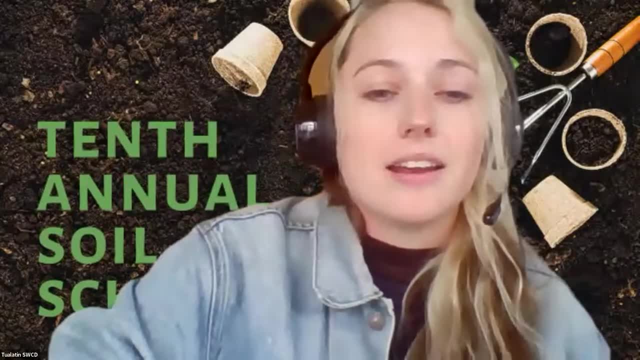 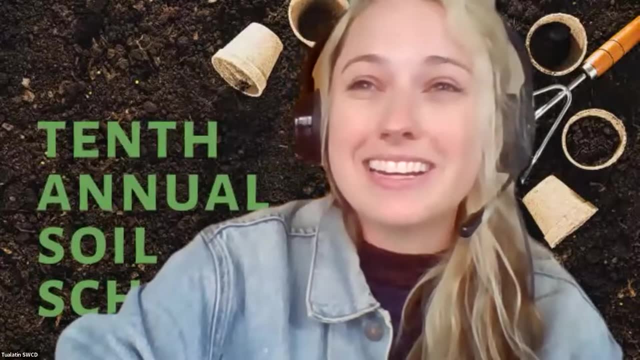 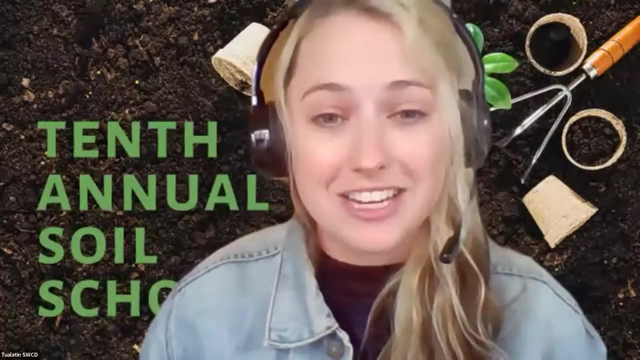 Now, before we get started with the presentation, of course we have to go over a few housekeeping tips. Tonight's recording, or tonight's webinar, is being recorded and it will be uploaded to our YouTube channel along with all of our presentations this month. by the end of the month, A couple will be up. 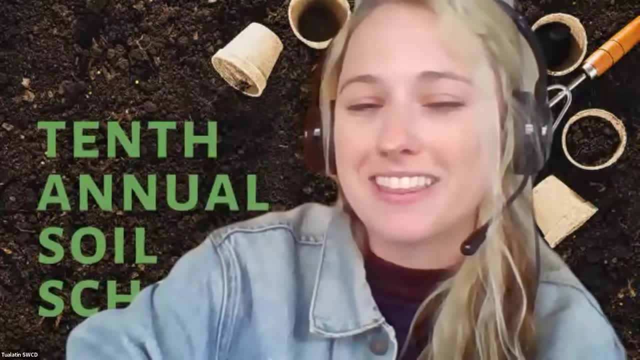 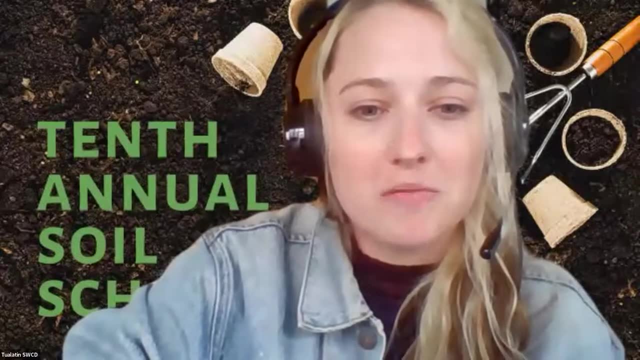 sooner than that, but they should all be there definitely by the end of the month. We're going to have at least 10 minutes for Q&A At the end of this session. if you're not familiar, there is a Q&A button down at the bottom of your. 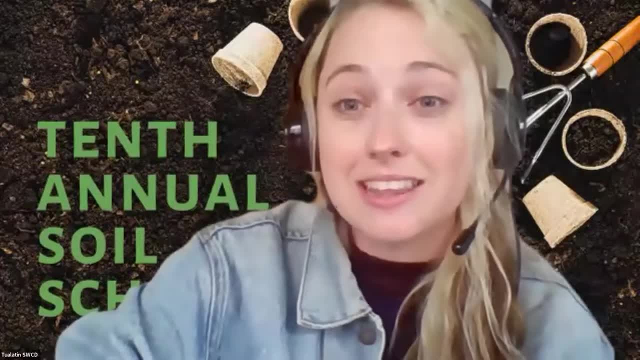 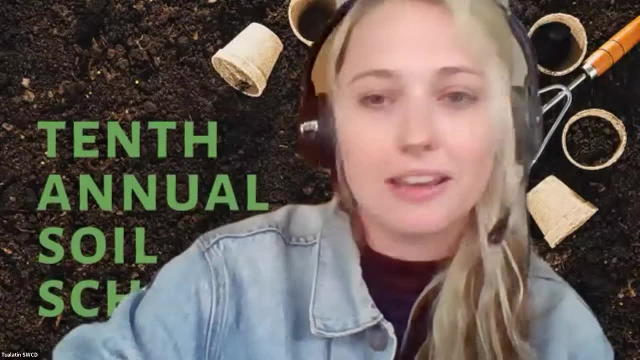 screen. That's where we'd like you to input your questions as they come to mind. That's a great place to put them, because you can actually upvote questions. If someone asks a question and you're like that's a great question, I want to hear the answer to that, just go ahead and give it. 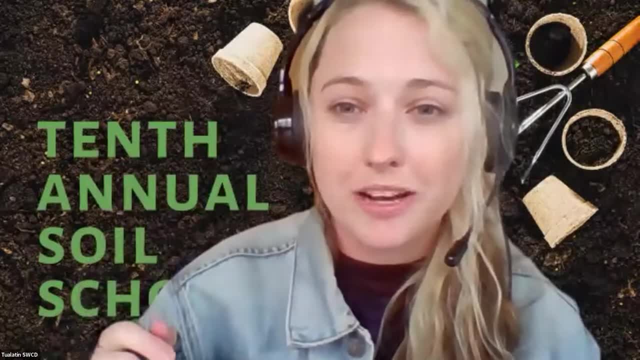 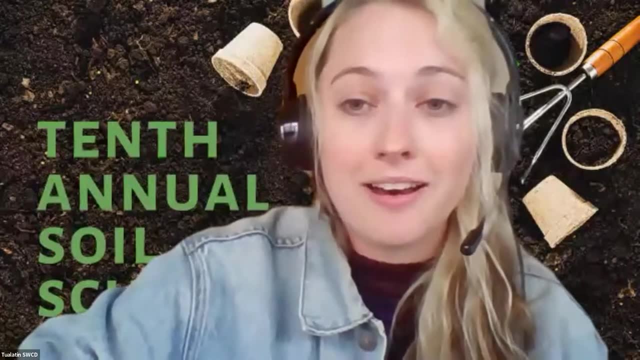 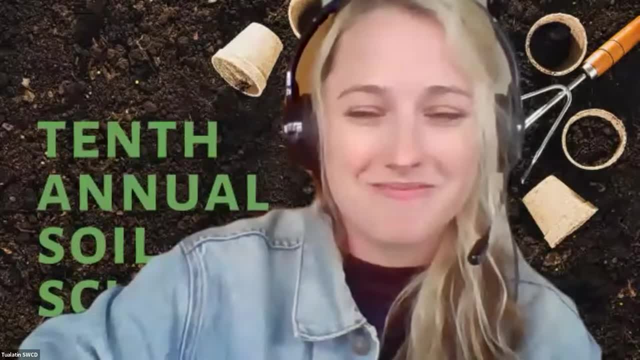 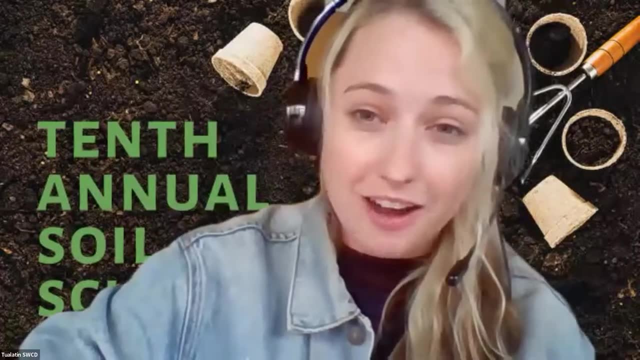 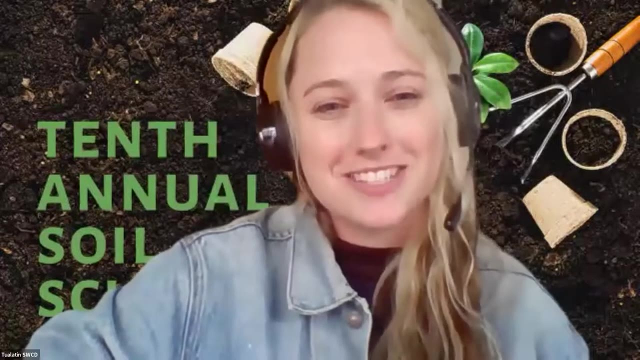 I will be monitoring that as well And, of course, we love to hear from you. Your feedback is very valuable to us. It helps us craft next year's presentations, So of course we have a feedback form for you and we would be so honored if you took a few minutes to complete that. I'm going 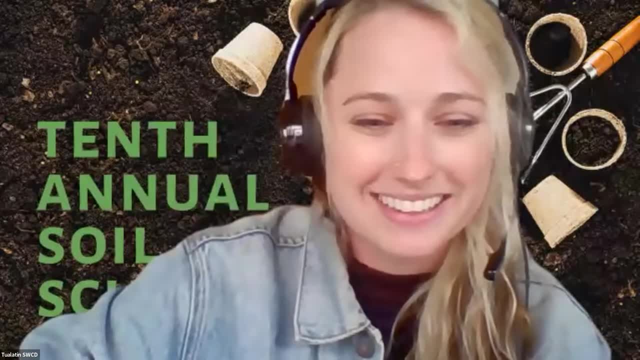 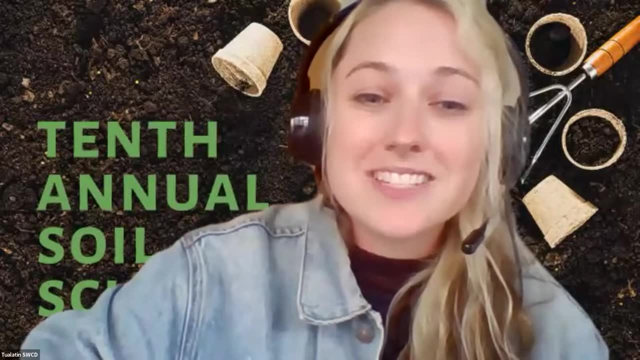 to hop. I'm going to drop that link in the chat box for you. So if you have any questions, if you have any questions, feel free to leave those in the chat box. And now I'm very happy to present to you Jennifer Moore. Last spring Jennifer joined the USDA Agricultural Research. 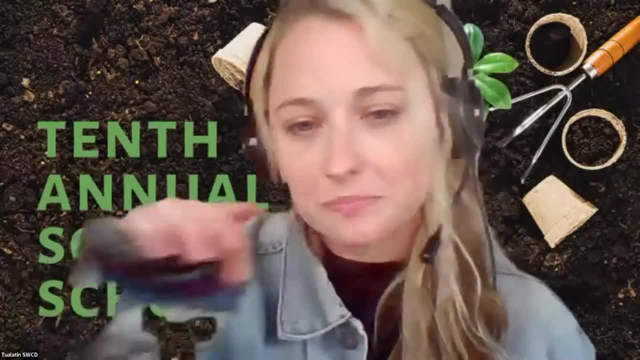 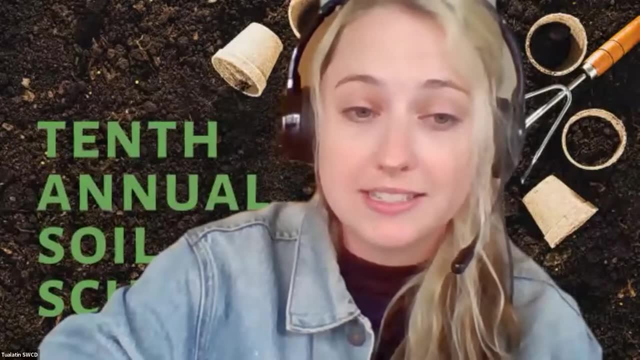 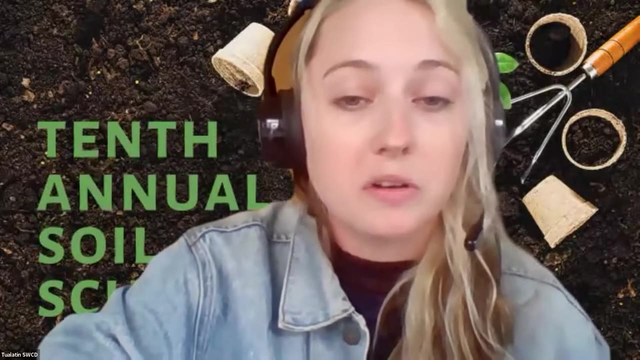 Service as a research soil scientist in Corvallis, Oregon. Her research will focus on soil health and soil carbon in forage grass and cover crops. seed production systems in the Willamette Valley. Jennifer has over 25 years experience in soil science research, including work in the third 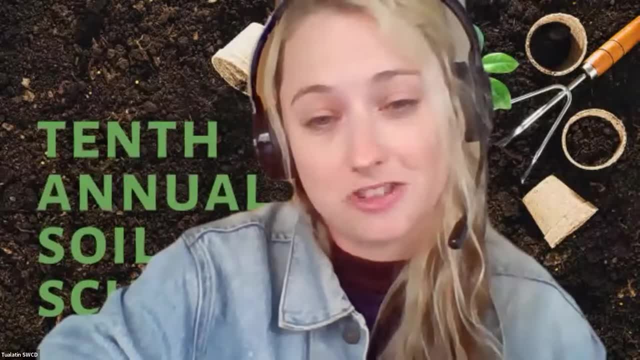 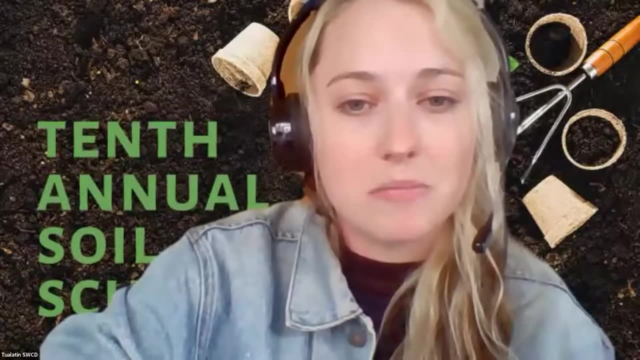 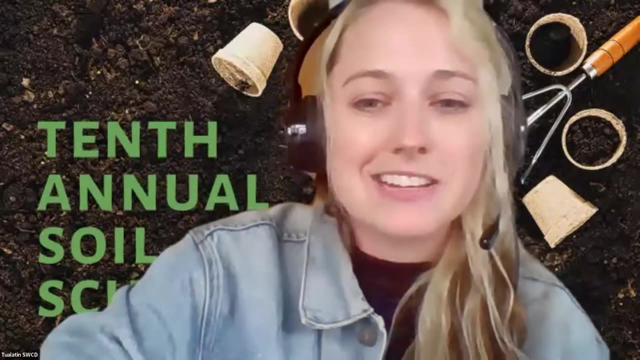 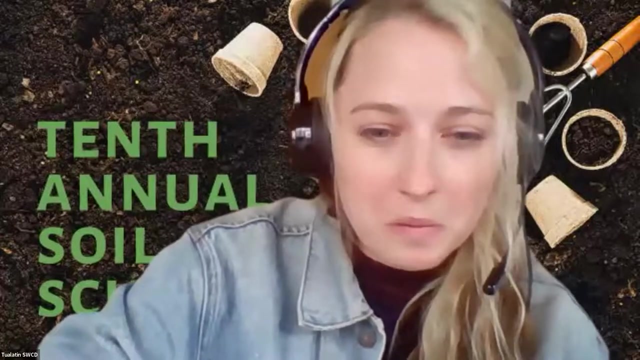 in multiple cropping systems and natural landscapes across the country. Before joining the Agricultural Research Service, Jennifer was the Climate Initiative Director at American Farmland Trust, the Western Soil Health Team Leader with NRCS and an Associate Professor of Soil and Environmental Microbiology at Texas Tech University. So now that our big introduction 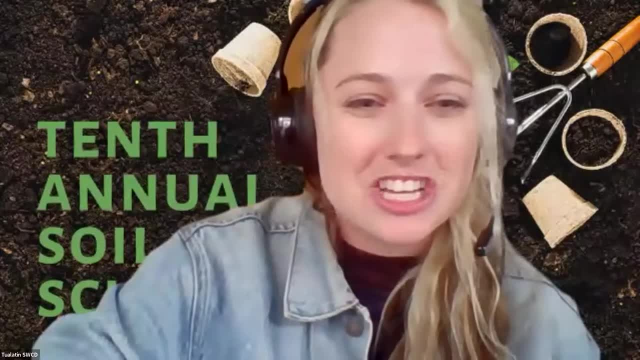 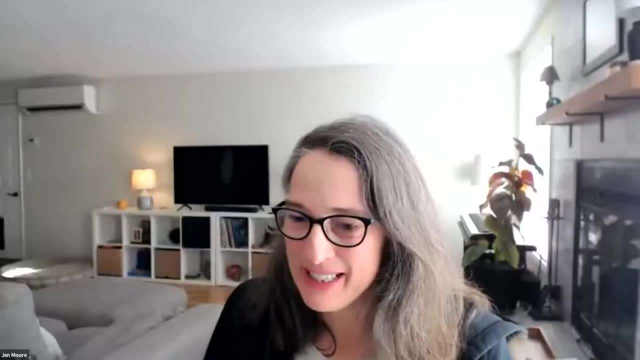 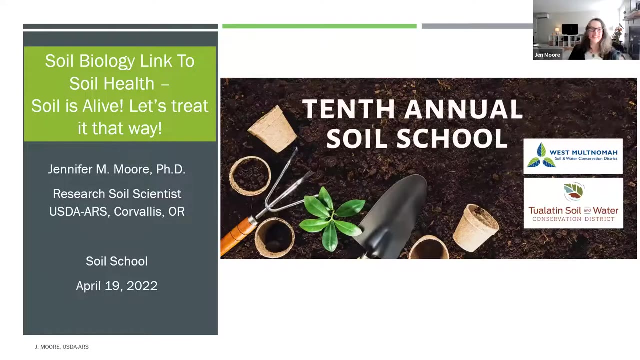 is done. it is time to get to it. Jen, tell us all about soil microbes. Great, Thank you. Thank you so much. Let me share my screen here. All right, Hopefully we're good to go. Great, All right, I wanted to thank you. 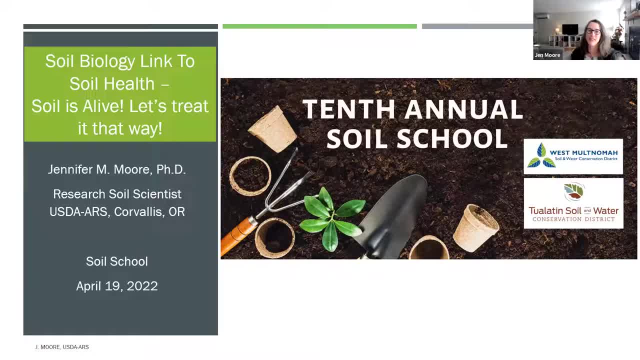 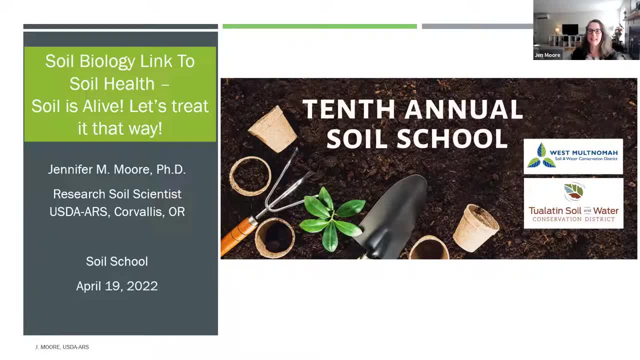 I also wanted to extend a special thanks to Renee and Annie for the invitation to speak today on linking soil biology with soil health, introducing some of the ways you can qualitatively evaluate soil health in your field or your gardens. I think this is the third. 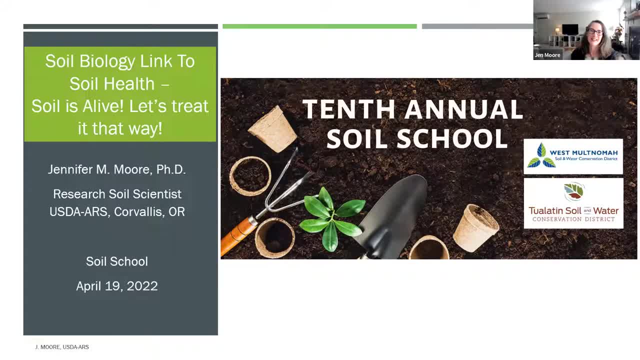 Soil School event I have participated in and hopefully next year we'll be back in person. That would be wonderful. So my goal today is to increase awareness and appreciation for the amazing living biological community below our feet. I'll start by defining soil health and 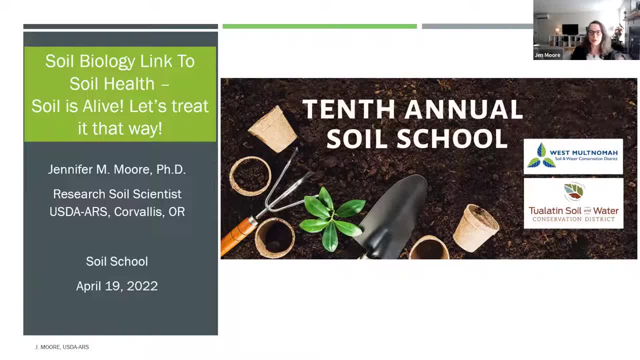 outline some key soil functions. We'll go over who's down there and what they're doing and discuss how we can monitor or assess soil health in your system. So hopefully in the end I'll inspire some more discussion and hopefully it'll help feedback on my end areas to research. 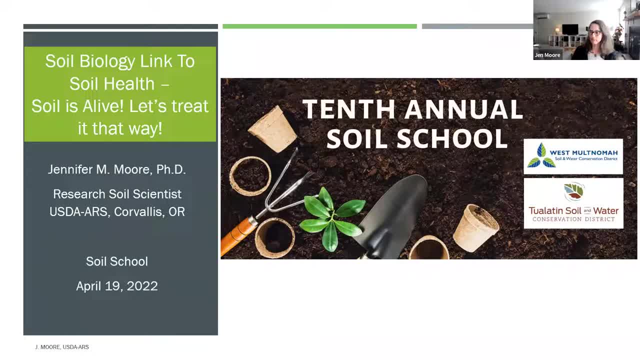 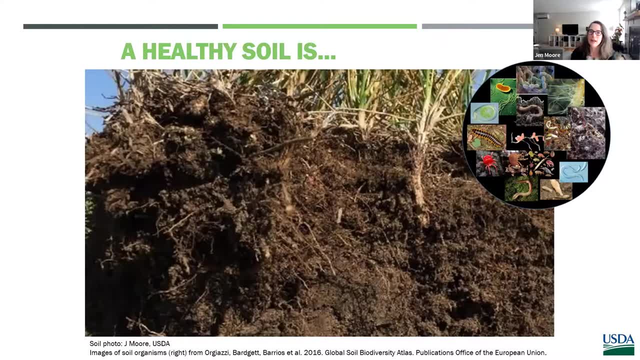 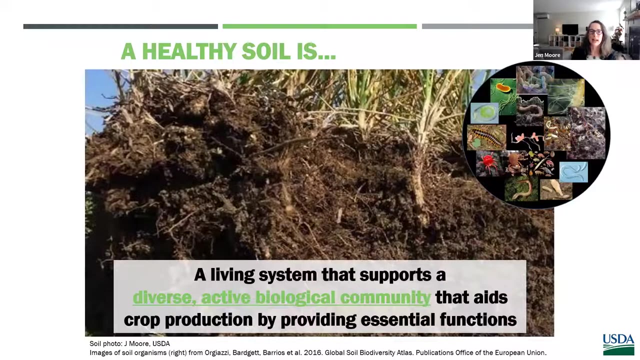 efforts on management impacts on soil health. Okay, so, building from the definitions that originated in the early 1990s, NRCS defined soil health as the continued capacity of soil to function as a vital living system, ecosystem that sustains plants, animals and humans. I also like to use health as an adjective, and thus we: 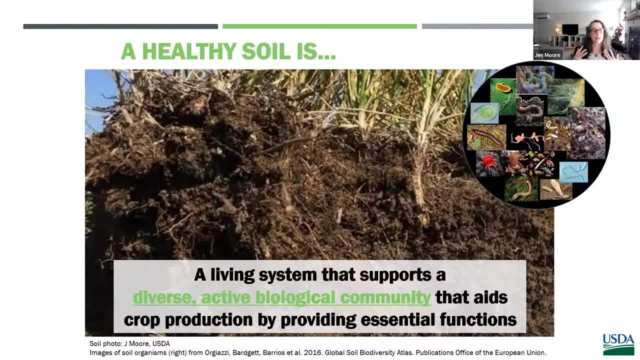 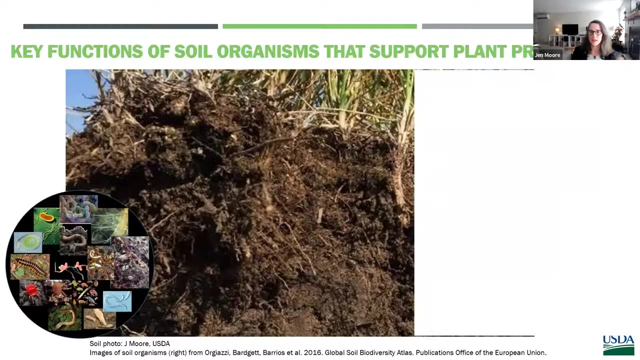 can describe a healthy soil as a living system that supports a diverse, active biological community, that aids crop production by providing essential functions, And so, zoning in on the term function, there are many that are critical for agricultural production systems and for the ecosystem and the environment overall, So there's a bunch that I'm listing here. 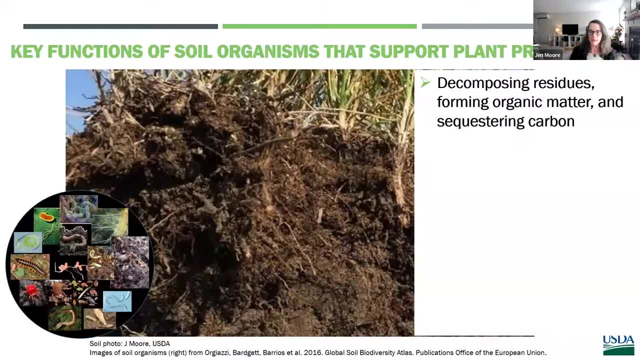 These include the decomposition of plant and animal residues, releasing and cycling plant available nutrients and enhancing plant growth. They also are involved in the formation of soil organically Matter through that decomposition process. Physically, the soil must also function to allow for adequate air and water flow, which is driven by the structure of the soil. 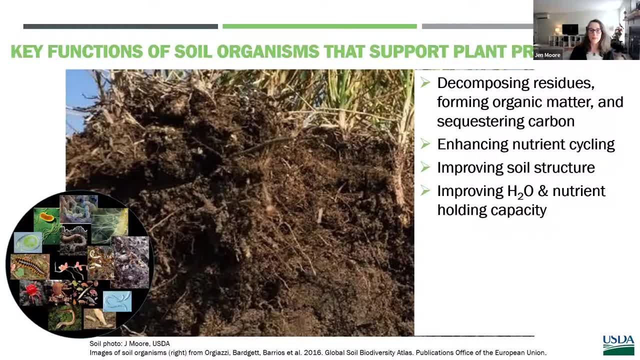 And a well-aggregated soil not only resists the erosive forces of wind and water, but it also helps water to infiltrate, filling the profile, filtering and storing for future uptake by plants. A healthy soil is full of abundant and diverse soil organisms which drive all of the functions. 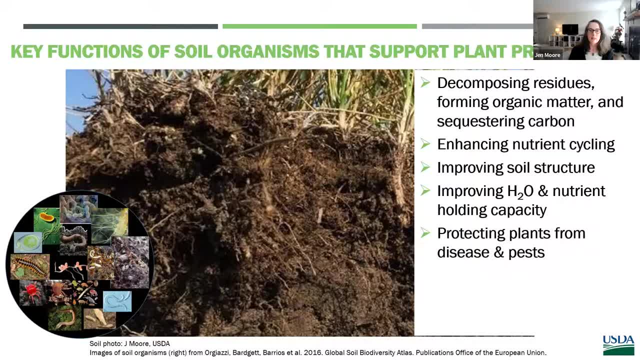 listed on this slide. This is an example of a healthy soil- And many more- And it includes unique functions such as forming symbiotic associations with plants like nitrogen fixers and mycorrhizal fungi that we'll talk about later. So microbes also help to detoxify pollutants and break down. 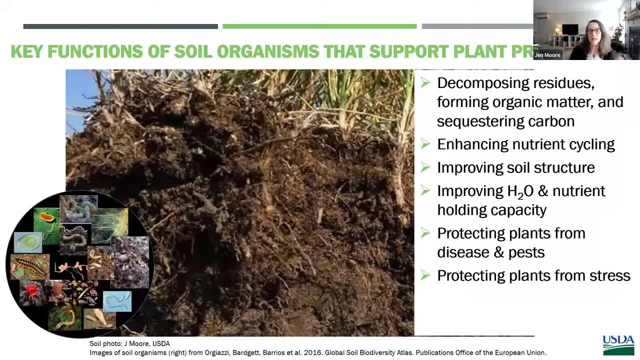 agrochemicals to help keep our soil and water systems clean, And the entire community in concert with plants, helps to suppress weeds and keep populations in check to minimize pests and pathogens pressures. So overall, a healthy system is both resistant to minor environmental disturbances like drought. 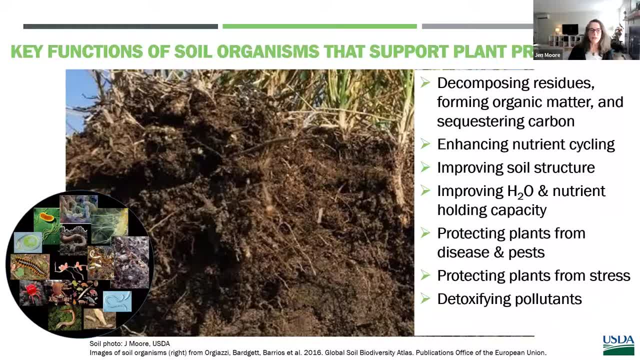 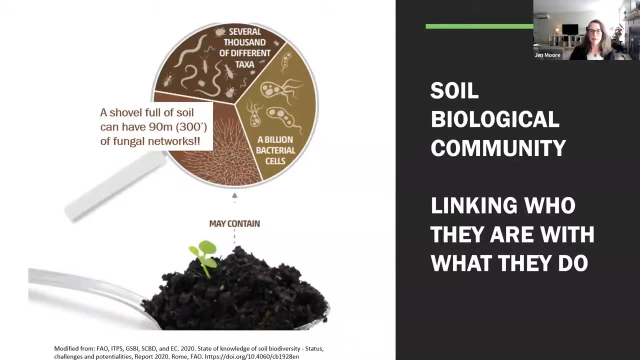 or flooding events, and it's resilient to more extreme events, like extreme drought, massive major flooding events- you know wildfire events, for example. So soils are amazing habitats for life. You probably have heard this already, but they're home to over 25 percent of all living species on earth. 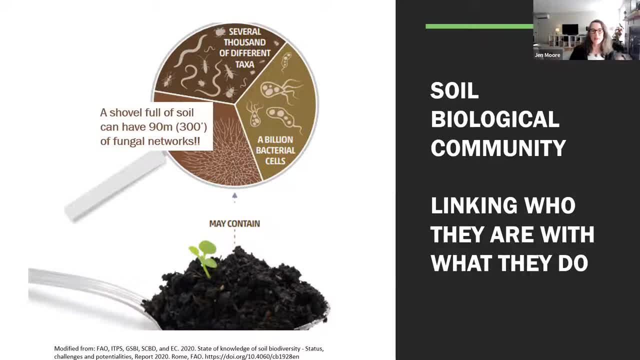 The vast numbers of organisms below ground is quite staggering. In just a teaspoon of really rich, healthy soil there can be millions to possibly a billion bacterial cells, many hundreds to thousands of different kinds of those bacteria, And in a shovelful you can contain hundreds of feet of fungal networks. 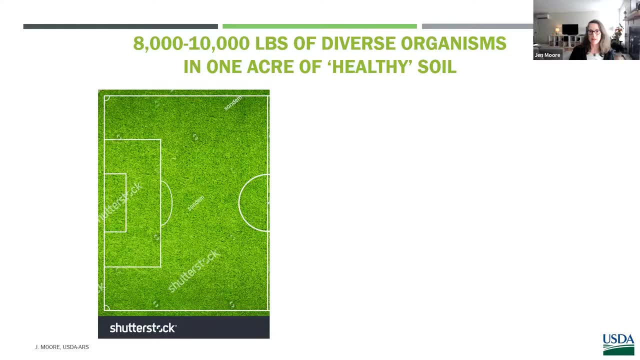 So healthy soils not only host vast biological abundance and diversity, but the living world and the environments. and the environments are all imbued with soil, And if you look closely at the soil, you can see that the mass below ground is equally impressive. 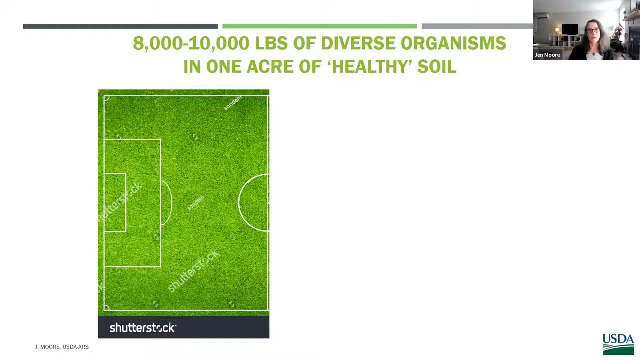 An acre of land is roughly half the size of a soccer pitch. So if we imagine an acre of healthy soil, there are between 8,000 and 10,000 pounds of soil organisms living below ground. That's equivalent to an African elephant on one acre of land. And so, keeping that sort of um analogy going, there is the equivalent mass of four to five cows' worth of manure annual population. And so, keeping that sort of analogy going, there is the equivalent mass of four to five cows' worth of manure in the ground. 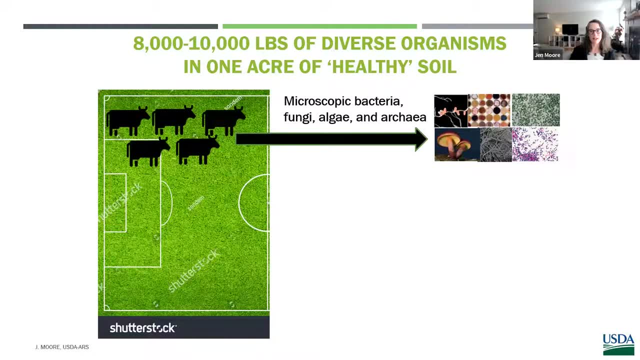 And so, if we look at science and the environment, if we look at soil, we can see our soil size and we can see the amount of soil that is low Boat, microscopic bacteria, fungi, algae and archaea- all things we can't see with the naked eye. 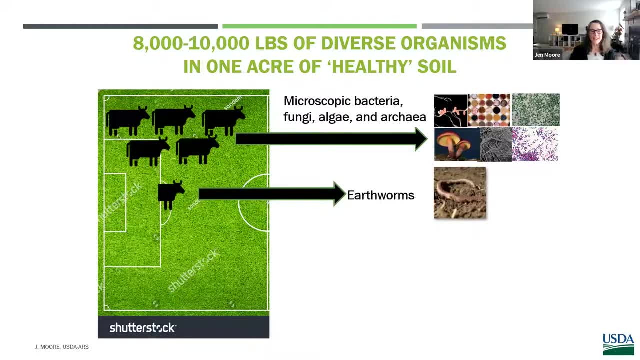 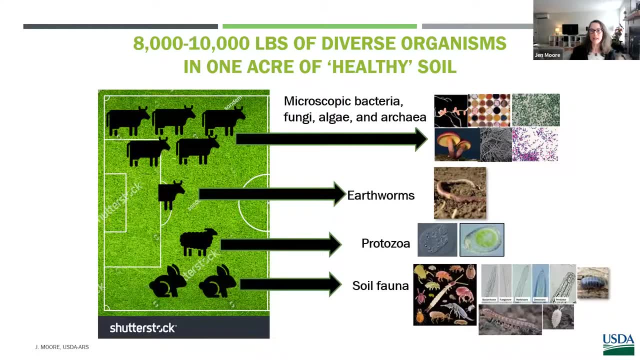 There's about a half to one cow weight of earthworms, There's about a sheep weight of protozoa, about two rabbits worth of soil, fauna or animals like beetles, mites, spring-tailed centipedes, nematodes, etc. And thus soil health and resilience depends on maintaining. 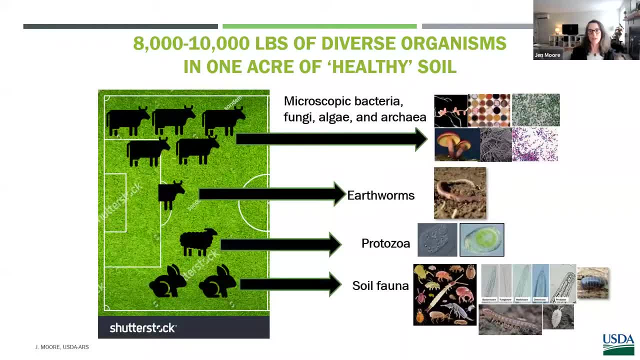 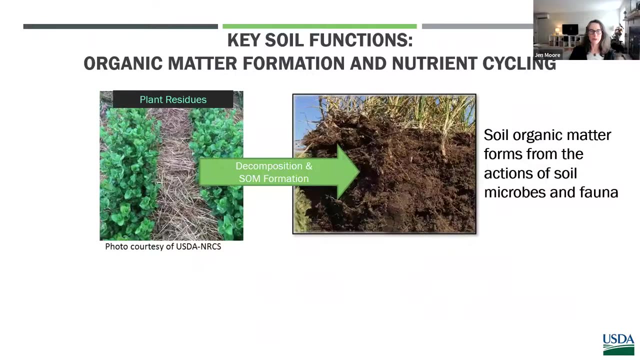 this diverse and robust biological community. that again, really can't emphasize it more. It's responsible for carrying out all of those important processes I described earlier. So let's look at a few specific examples linking soil biology with function. One of the most important functions is the formation of soil organic matter. 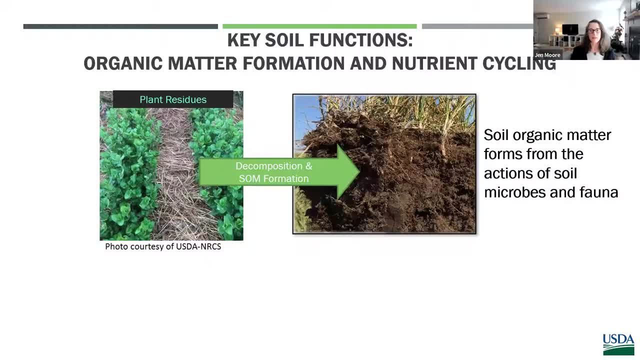 This important property of soil is important for functions like nutrient cycling, all of which are important for the development of soil, organic matter, All the way to combating climate change, and also storing and filtering our water. So it's critical for every environmental and ecological process we can think of. 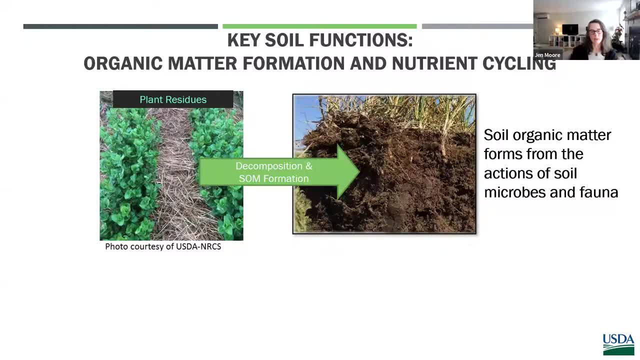 And it also helps to release nutrients over time through decomposition processes, And so traditionally, scientists thought that stable organic matter originates from the preservation of complex plant compounds that are resistant to decomposition, But we now know that forming stable organic matter is largely from dead microbial cells and their byproducts. 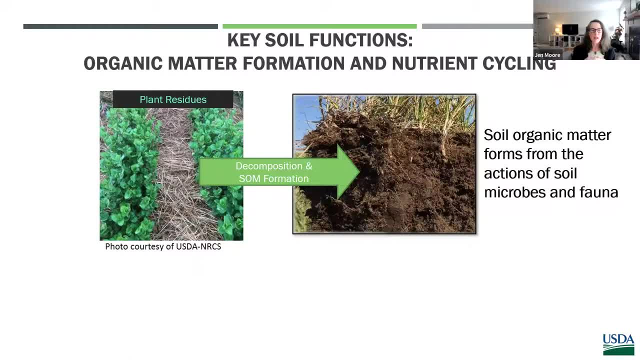 These are kind of absorbed to particle surfaces And so what's really important about that function is historically we kind of viewed the soil and organic matter as this chemical property and sequestration of carbon sequestration as a chemical property. But it's really how we 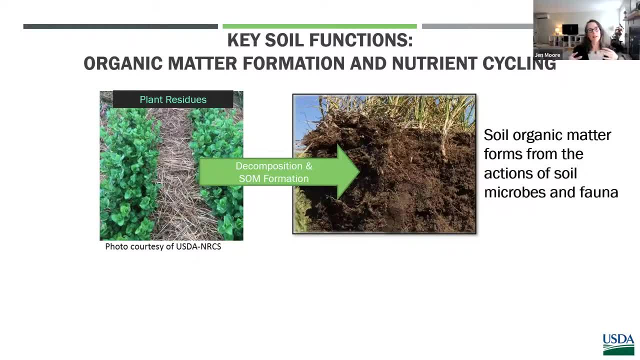 maintain, feed, fuel and cycle that biological community and their dead microbial cells In a taking on a lot of changes. So we need a lot of good. we need a lot of good that can contribute and help to combat some of the climate change that we're experiencing. 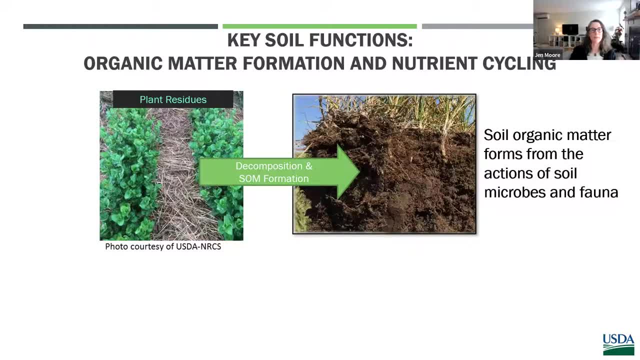 Of course, the food that microbes needs primarily comes from plant sources, But seeing soil organic matter formations stemming from the actions of soil microbes supports the concept that managing for healthy soil should equate to managing for optimal biological activity and microbial biomass. So during decomposition, plant and animal residues are converted to matter and there are going to be. 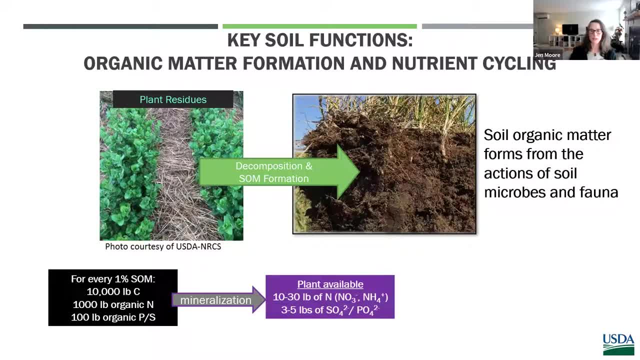 to plant available nutrients through a process called mineralization, So soil. I think I have a pointer here. So soil organisms take organic matter, they degrade it and break it down into parts, And so for every 1% of soil organic matter there's about 10,000 pounds of carbon. 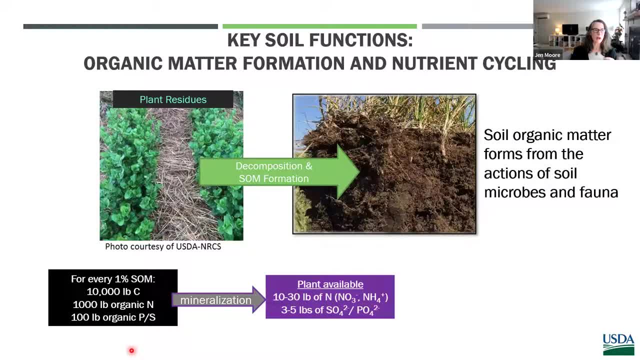 1,000 pounds of organic nitrogen and about 100 pounds of organic phosphorus and sulfur. That's sort of like this long-term pool that's just hanging out in the organic matter And over time about 2% to 3% of that each year gets converted into plant available forms And again that's 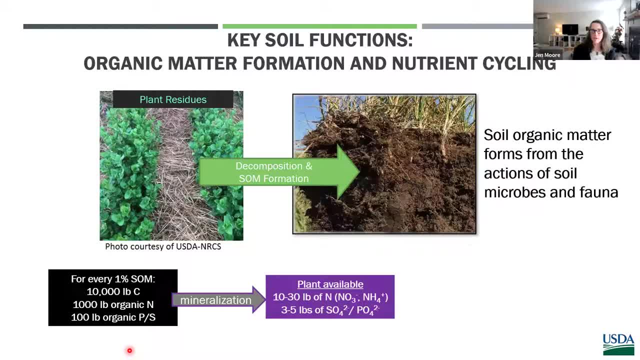 called mineralization And those forms are like nitrate and ammonium for nitrogen, phosphate, sulfate, those types of compounds. So in about a year you can release, just from the natural decomposition process, about 10 or 30 pounds of nitrogen and three to five. 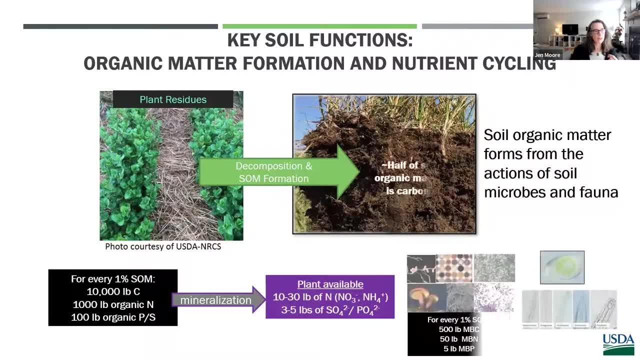 pounds of sulfur and phosphorus, And also it's important that that microbial biomass is also containing nutrients. So in that 1% organic matter there's about 500 pounds of microbial biomass carbon, 50 pounds of biomass nitrogen and five pounds of biomass phosphorus And, as 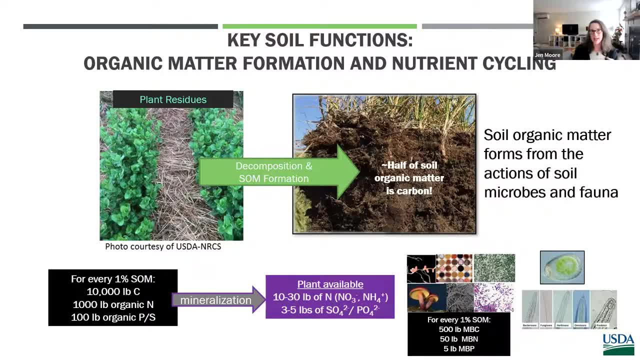 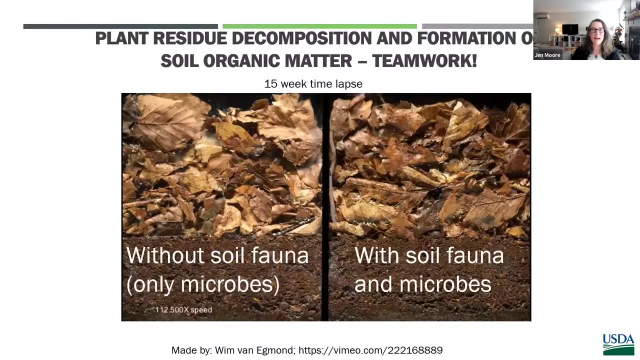 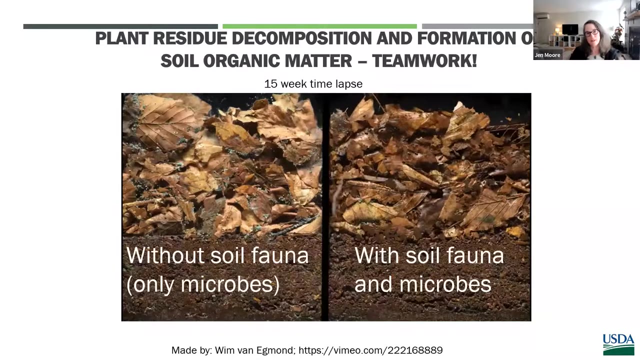 those organisms. they die and are decomposed. those cells also release some of that inorganic plant available. This is a slide, just I'll let it play a little bit. It's my reminder- I kind of joke- that I'm microbe-centric. I study soil microbiology and microbial ecology and biochemistry, And sometimes 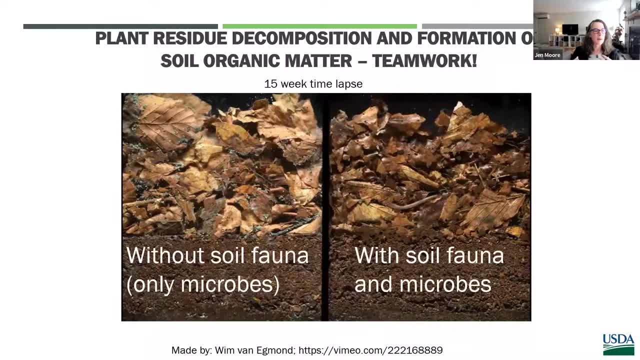 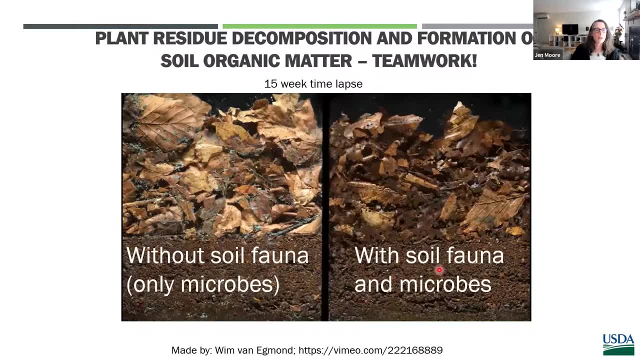 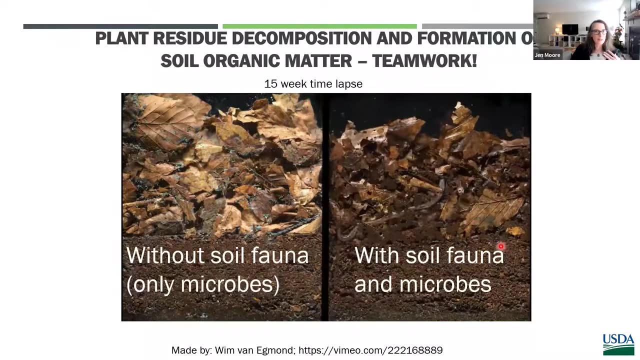 I forget about the larger organisms because I don't study them, But this is a really great video. It shows the decomposition of, in this case, leaf matter with soil fauna. So all of the larger organisms, including earthworms and centipedes and millipedes and beetles and all. 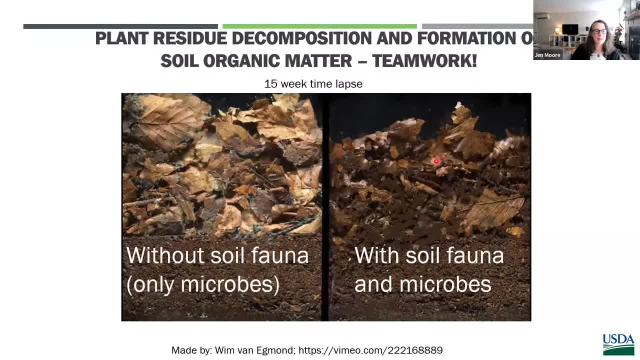 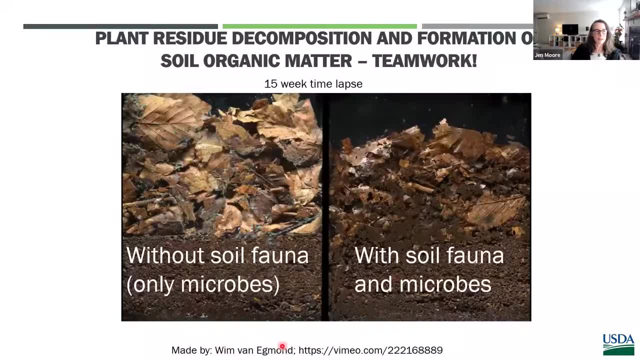 the- I call them the creepy crawlies right in the soil with soil fauna and without, So just soil microbes, And it's a 15-week time-lapse video and the source is listed here for you And you can. 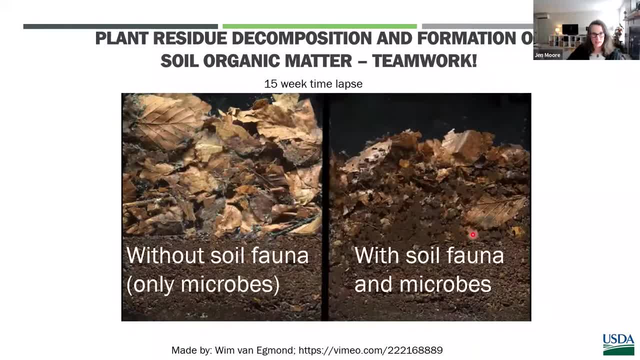 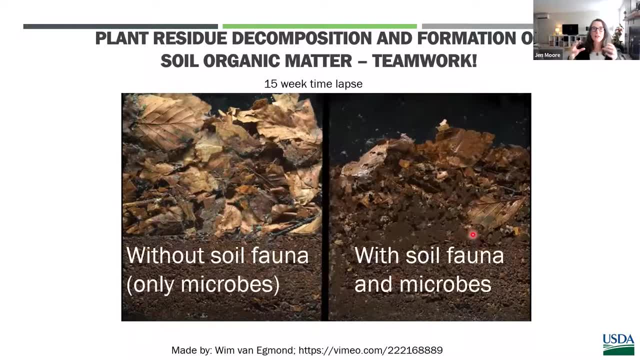 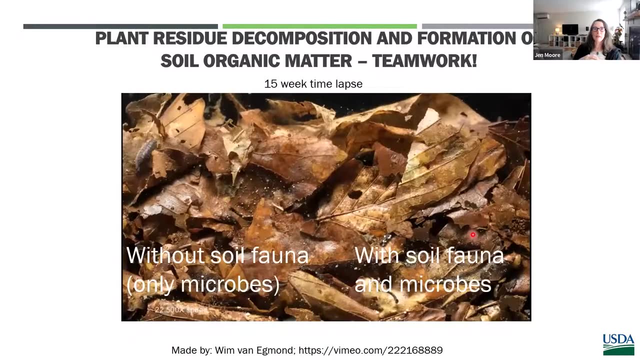 see how quickly the mixing and the translocation from the surface below ground through the actions of the soil fauna. They're also stimulating the microbial population because they're chewing up all those large fragments of organic matter And they're releasing. you know, they're cutting it up, they're chewing. 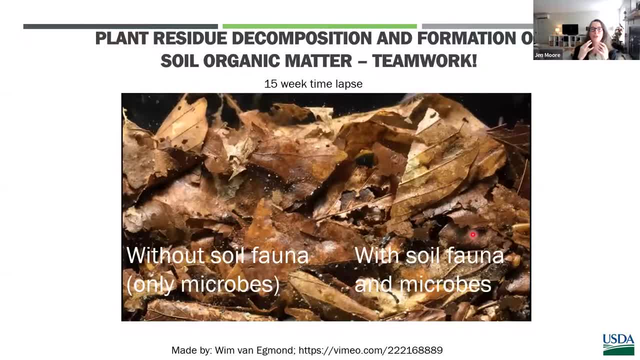 it up, And it's kind of like similar to what we do when we eat food: We chew it up, we create smaller pieces, A, so we don't choke but B, so the enzymes in our mouth and our gut can then go. 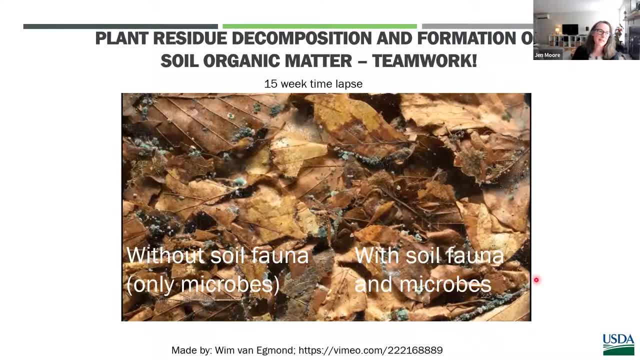 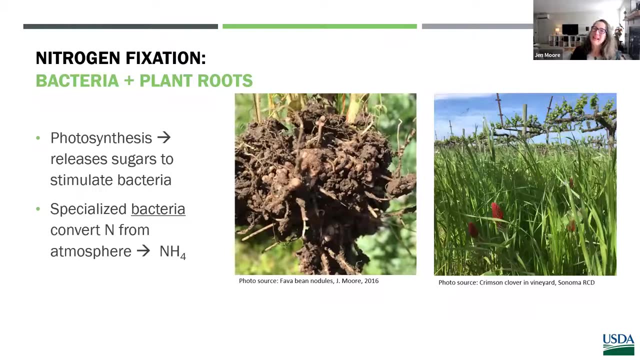 to work to release the nutrients that our food contains, And so that video is just my reminder, and now yours, That it's a whole community that's responsible for this, not just the microbes. Okay so, but microbes are really incredible organisms. Here's one example of bacteria that: 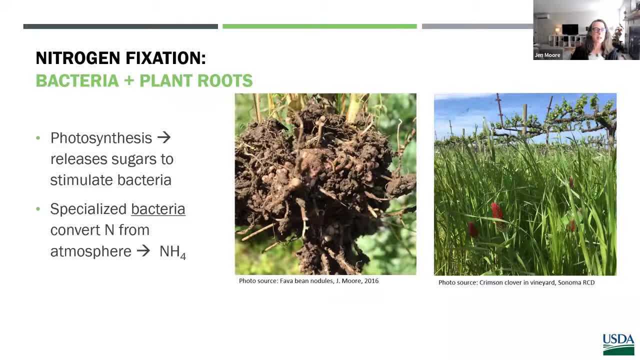 team up with certain plant roots. These bacteria are involved in nitrogen fixation. So what they do is they come in and with plants, like legumes, they form these little nodules, these little fibers on the roots, And inside of those nodules they're taking atmospheric nitrogen. So about 80%. 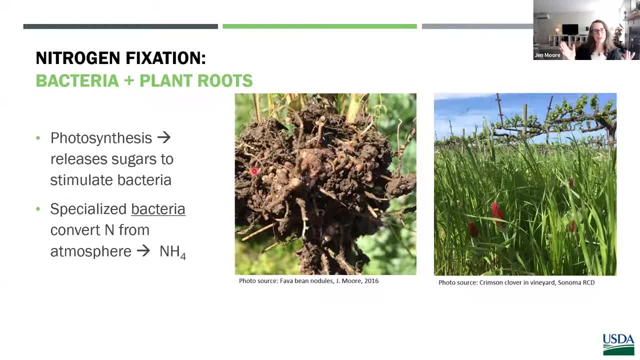 of our atmosphere is dinitrogen gas. Inert doesn't do anything. but they take that nitrogen inside of that little nodule and they break it apart and they create ammonium And in return they give that to the plant And in return the plant gives them sugar and a nice protected home to live in. in that 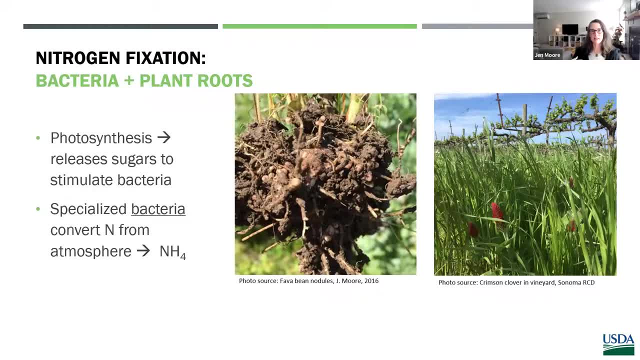 little nodule. So the process is the biological nitrogen fixation and it supplies a really incredible amount of nitrogen to our plants. So anytime you can incorporate a legume into your crop rotation as part of your cover crop mix, it's naturally going to take nitrogen out of the air and put it. 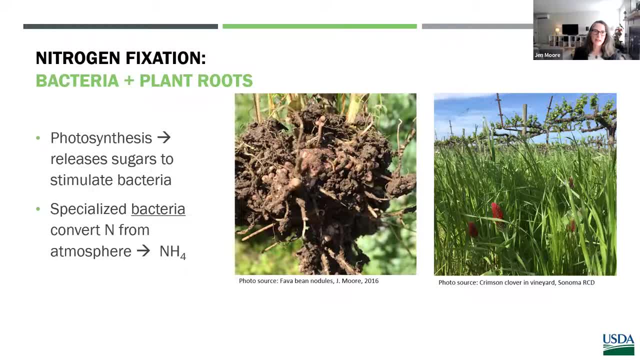 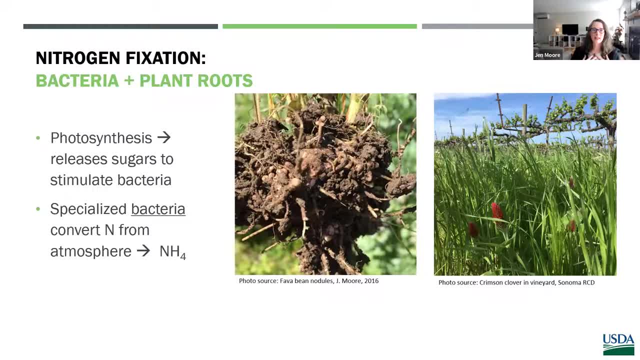 We can do the same thing. Humans are very crafty. We can take nitrogen out of the air and break it up and form fertilizers right. You can buy a bag of that at your local Home Depot But it takes us an enormous amount of heat pressure oil. It's a very energy-intensive process to do the same thing. 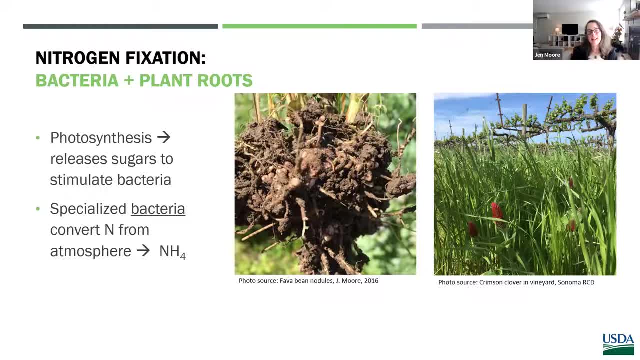 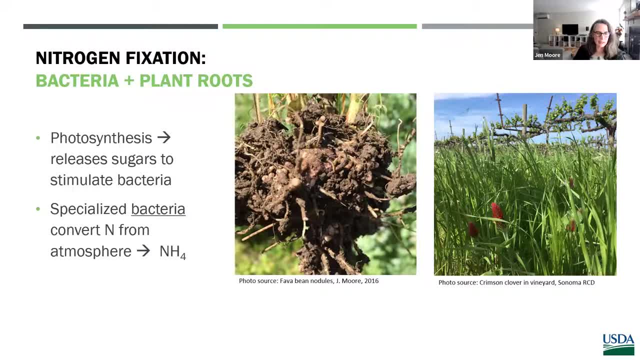 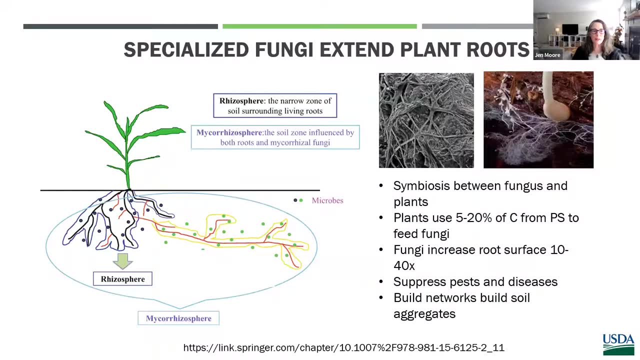 So really, really cool and a really important plant and symbiotic association to consider for your garden or your fields. Another really important symbiotic association is between plant roots and a fungus, So these are mycorrhizal fungi. Mycorrhizae is a Greek word meaning fungus root. 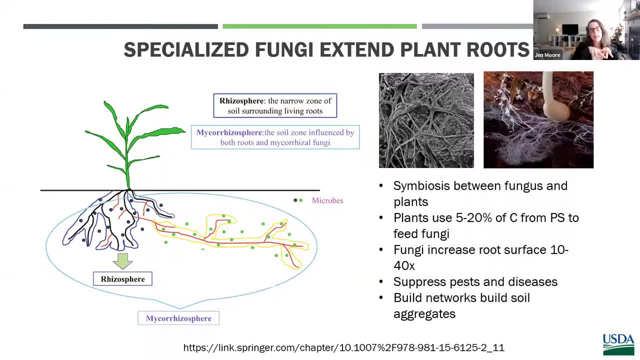 And the fungus basically attaches itself to the plant root and then it extends out into the soil, increasing the functional rooting surface 10 to 40 times. I kind of think of it as like hair extensions, right, Like you're extending the area of in this case. 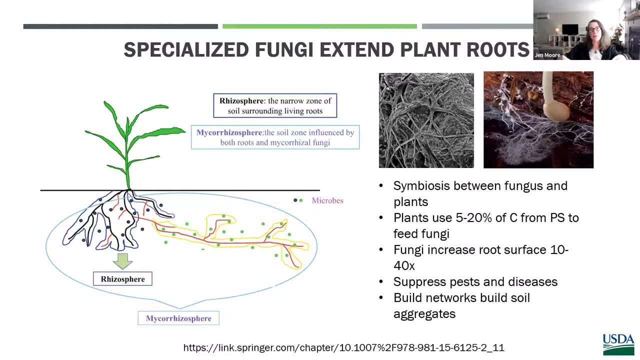 the plant root And when it can do that, it now has more soil volume to explore for things like nutrients and water, So it's really critical to help in that particular case And, similar to the bacteria with nitrogen- nitrogen fixation- the plants provide the microbe. 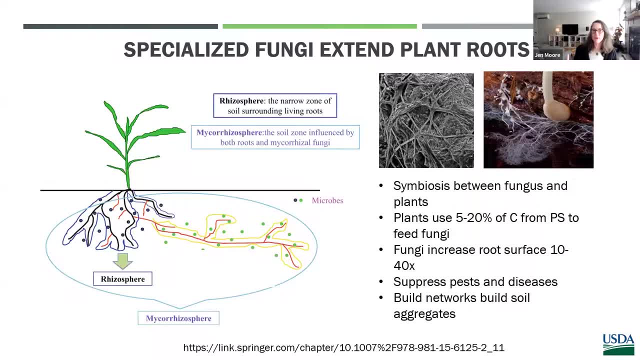 in this case the fungus sugars. About 5% to 20% of carbon, usually in the form of some type of sugar, is allocated to the fungus Again. in return, the fungus is now extending the rooting surface area. 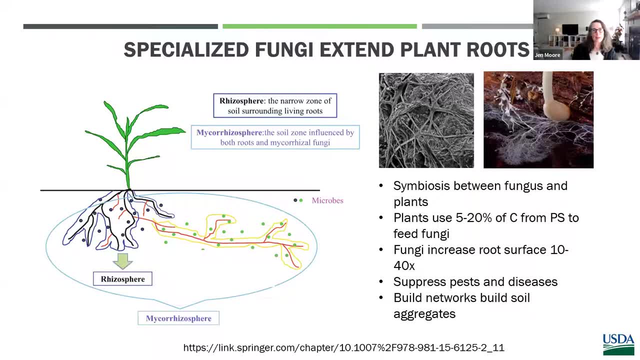 It helps bring phosphorus and nitrogen sulfur back to the plant, and also water, And there's also been some work done where these associations can help plants defend themselves against certain pests and diseases, And fungal hyphae are incredibly important for building. 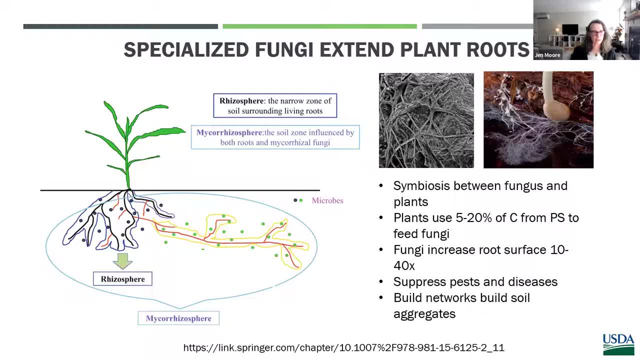 soil-stable aggregates, And we'll talk about those later on. So most plants are mycorrhizal. One exception would include the brassicas, which do not form these types of associations, So I wanted to point that out as well. 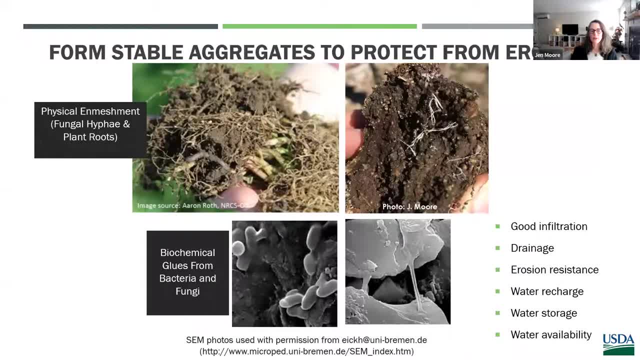 So here are those stable aggregates that I mentioned earlier. So these are important for numerous functions like resisting the erosion, resisting water and wind erosive forces and forming good structure for air and water flow. It's a physical property but in reality, aggregate formation. 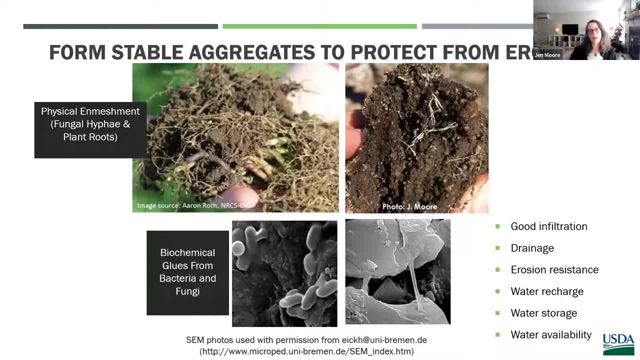 is largely a biological process. So there are two ways that soil organisms help form stable aggregates. The first is this physical enmeshment. So think of those fungal hyphae and plant roots Here. They're shown In this image. you can just see all of the roots. 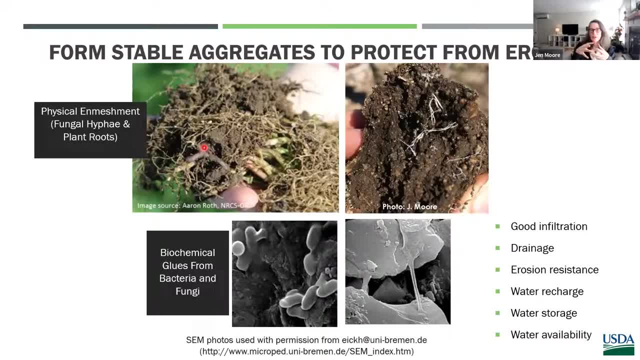 as well as some of the fungal hyphae. They're encapsulating the soils and they're holding it together kind of like a hairnet. Hold your hair in place. The fungal hyphae and the roots are holding that soil in place. 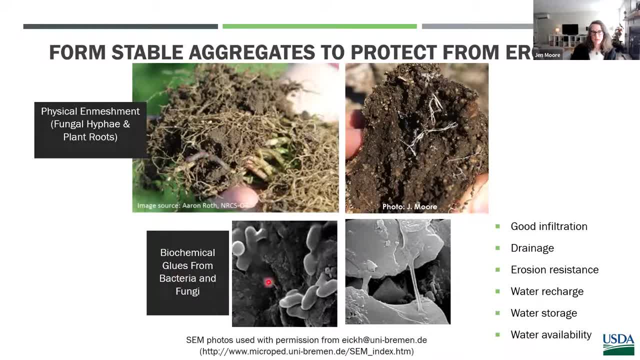 in an enmeshment There's also a biochemical process, So bacteria and fungi alike release sticky substances that help literally stick, Aggregates together and forms like a glue that helps hold these particles together, making them resistant to erosion, And so this is a really high powered microscope. 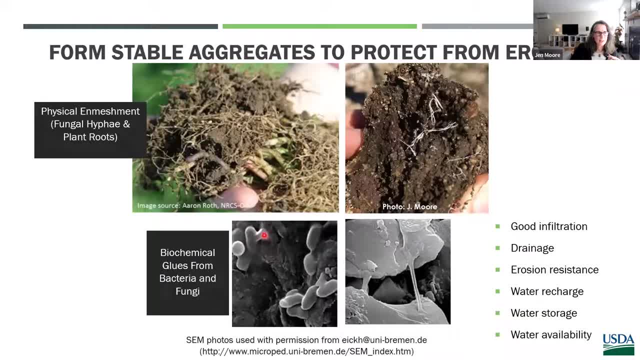 These are bacterial cells And right here you can see this is a soil mineral particle And this is a little ooze coming out of the bacteria that's sticking that bacterium onto the surface of the soil particle. So a whole bunch of these guys get together. 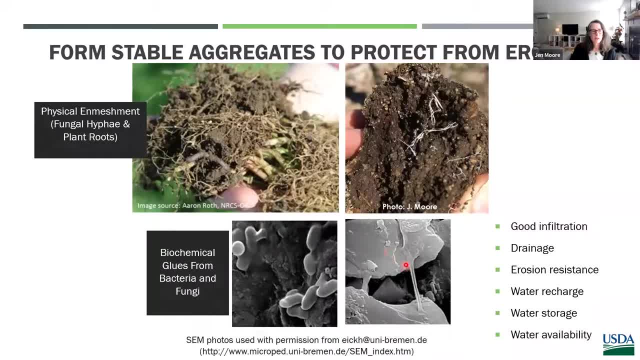 And they help glue the particles together. This is another really high powered image. Again two particles, And then there's this thread-like material. A certain bacteria called Actinobacteria also produced this sticky substance holding it together. And then finally up here, these are fungal hyphae. 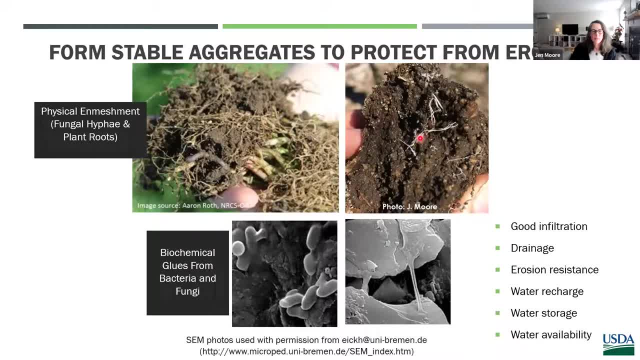 These are not mycorrhizal. These are involved in the breakdown of dead stuff, But they're also helping to enmesh and encase And they're also helping to hold the soil together And they're also helping to enmesh and encase. 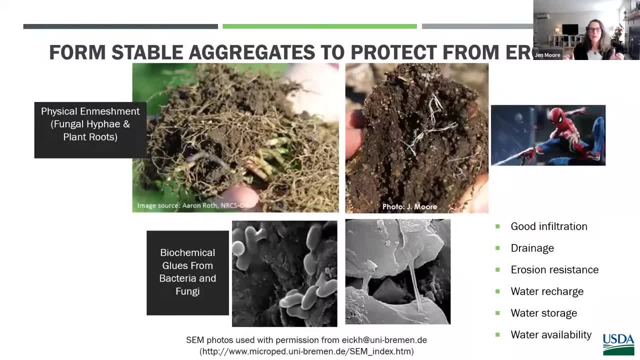 And they're also helping to enmesh and encase And hold those soil particles together. So I kind of think of it. they're superpowers, kind of similar to Superman, To- oh my god- Spider-Man. I was going to call him Batman for a second. 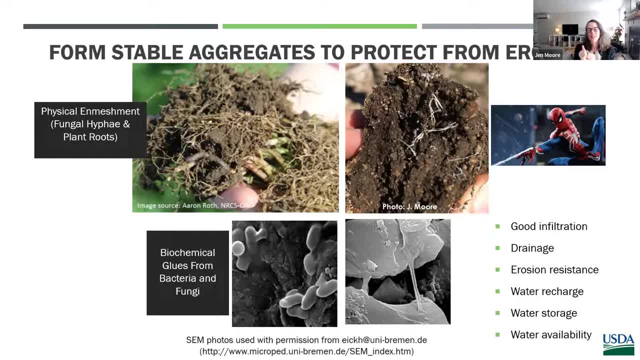 To Spider-Man right With its strong thread-like substances that's holding the bridge, or holding the bus that's almost falling off the bridge and saving all the school children. Similarly, the fungal hyphae, the bacterial glues, are holding those particles together. 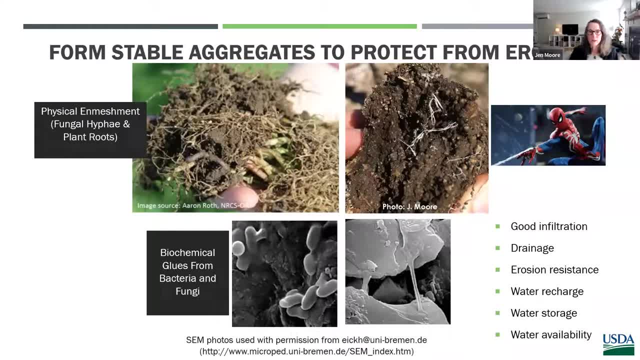 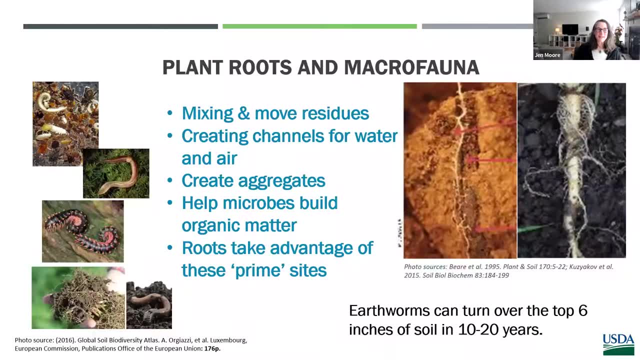 Saving that soil from blowing off in the air or running off the field in water erosion, OK, And so other plant roots and macrofauna again are really important. The larger organisms help to fragment, mix and move those residues, like I showed in that video. 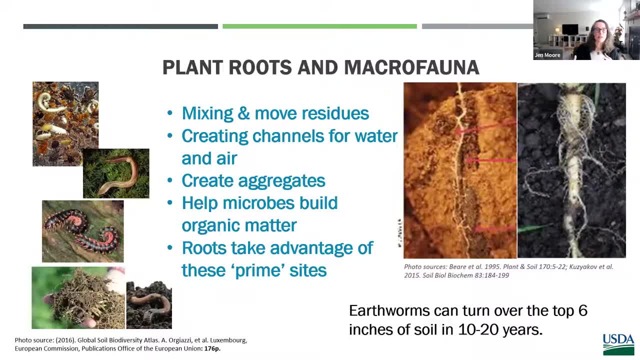 These organisms are sometimes called to the ecosystem engineers because they're like the movers and the shakers of the soil. They're really important for creating large, large channels for water and airflow. sometimes called biopores, They help also to create aggregates. 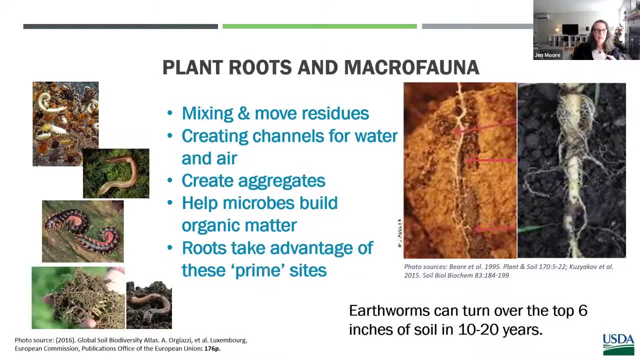 They help microbes build organic matter And in this particular case, I wanted to show that this is an earthworm channel. So earthworms, as they channel through the soil, release material out the other end. It's rich in organic matter nutrients. 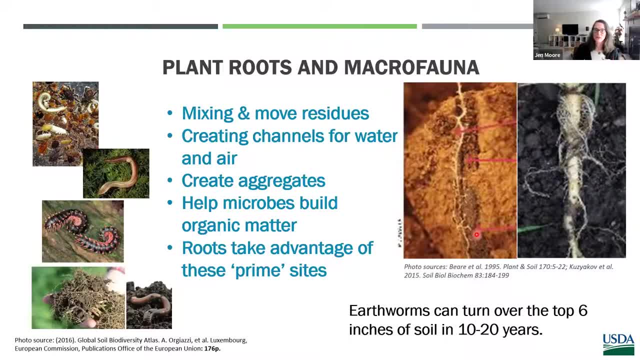 It's a neutral pH And it's very resistant to erosion, And so water can flow, Air can flow in these channels. It's loaded with bacteria, And so when these channels are there, the roots can then take advantage of them And they're kind of like in this primed environment. 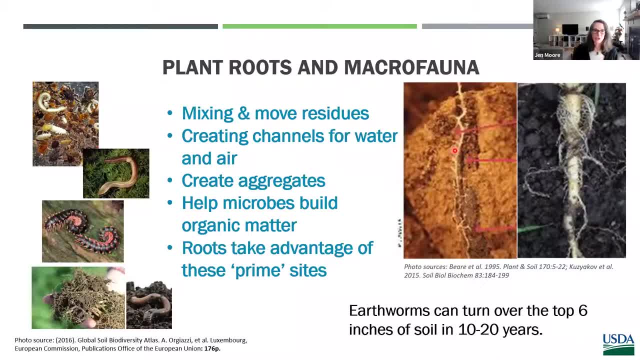 to be able to get off to a healthy, strong start. Similarly, root channels themselves. this is a radish or some sort of large rooted plant that, as it decomposes, it's going to leave a large gap in that soil for that airflow. 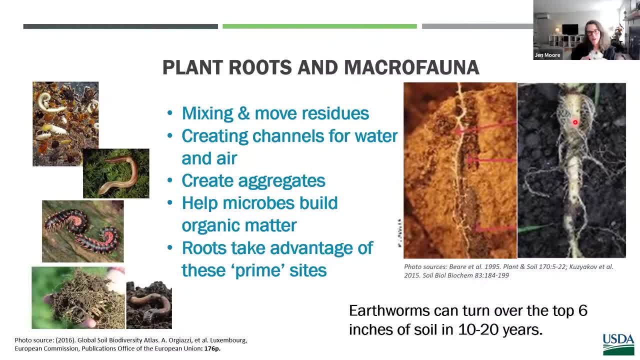 And as the material is degraded, it's also going to be a site of a hot spot of microbial activity. So leaving these channels in place are really important. When we till, we're disrupting these channels, And so we no longer have that kind of easy passage. 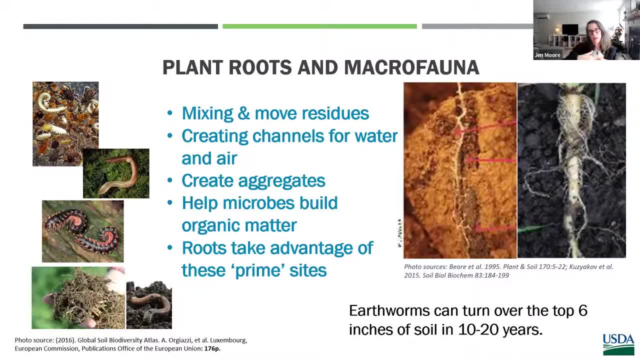 for the next root and the next crop to come in and take advantage of those channels for nutrients and water flow. So that's it. And then just another plug for earthworms, like how important they are. they can turn over the top six inches of soil in 10 to 20 years. 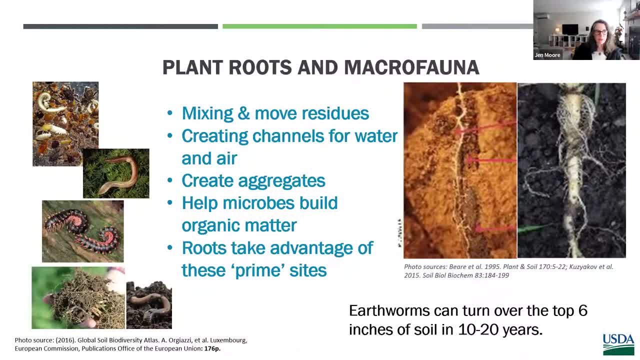 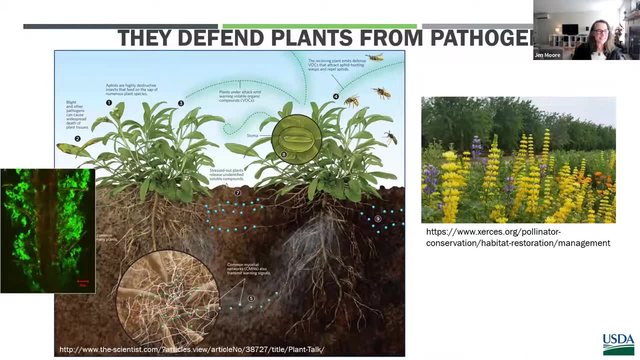 And so very, very important mixers and movers of organic materials. This is one of my favorite slides. Hopefully I can go through it here. So plants and microbes have this unique communication system that scientists are just beginning to decode. So, for example, on the left this: 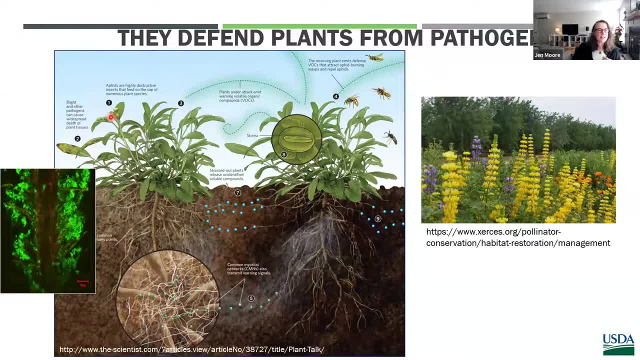 plant is being attacked by a pathogen that's entering the plant through the stomata. This sends a chemical signal below ground that causes beneficial soil bacteria to come to the rescue and swarming the root to first protect the below ground system from any further attack. 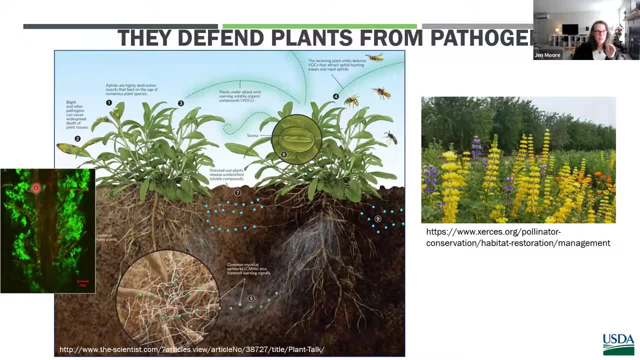 So that's kind of shown. this dark image is a root And these green fluorescently dyed substances are bacteria that are swarming the root. So they're good guys. They're beneficial organisms to help protect that plant below ground, while it's being stressed above ground. 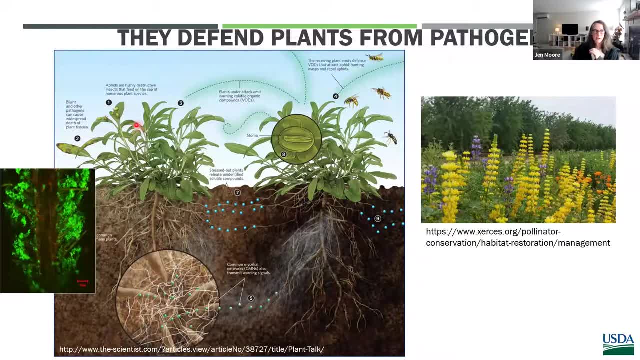 These bacteria also release a chemical that goes back up to the plant, tells the plant you're being attacked, close your stomata, batten down the hatches. There's bad guys in the area. You need to protect yourself. So that's one form of communication above and below. 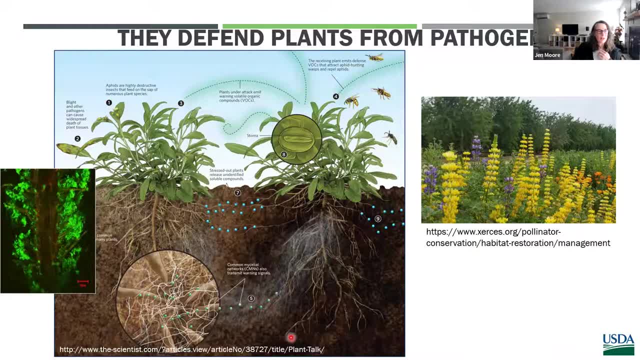 ground that plants and microbes use. There's also another. This is an instance- where the plant is being attacked, now through the stomata, with, I think it's- aphids, And in this case now the plant is sending a volatile organic chemical. 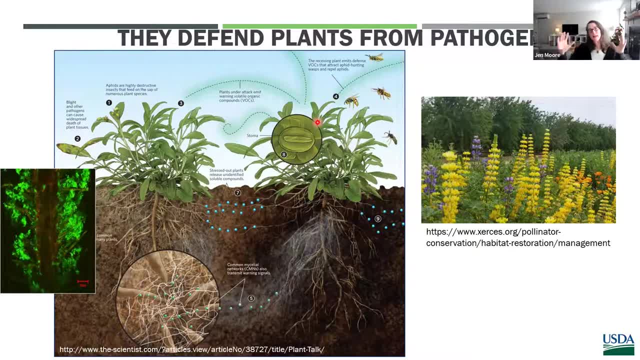 It's like a pheromone into the atmosphere. It's an SOS signal that if these wasps are nearby that can attack the aphids, they'll come in. they get the signal and they swarm in and then they can start to attack the aphids. 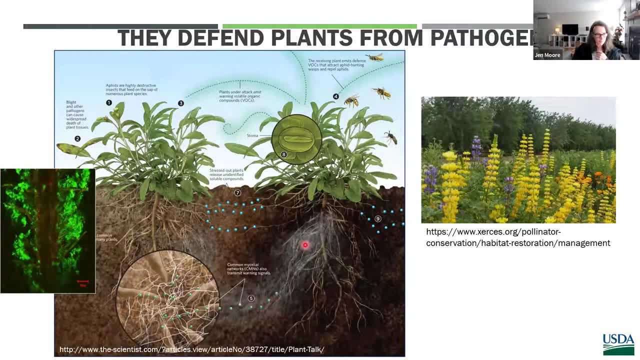 To reduce that pathogen or that pressure. Finally, there's another information signal below ground. through those mycorrhizal fungi, the fungi that can attach to plant roots, In this case, this plant is being attacked on the left. The signal comes down now: 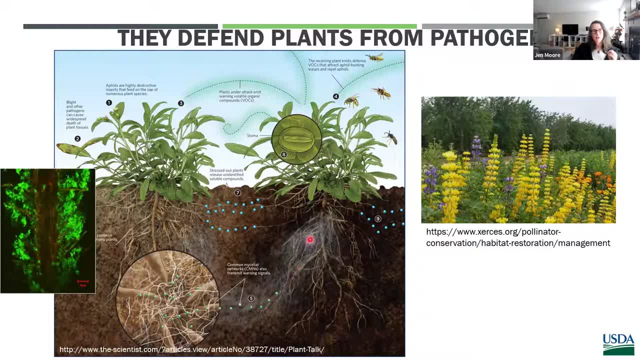 It goes through the soil, through the mycorrhizal hyphae. Over here this plant is not being attacked, But it's being told that its neighbor is being attacked. It will automatically then close its stomata to protect itself from the pathogen. 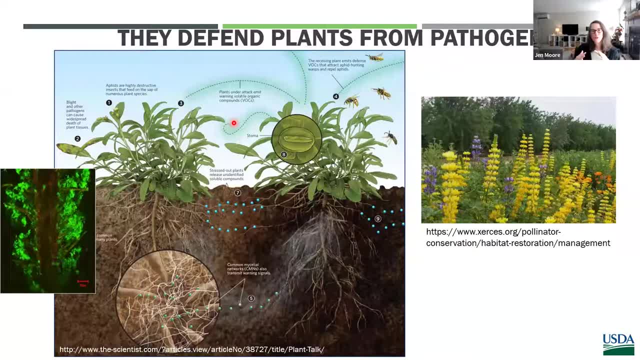 that is infecting through the stomata. So this is the whole communication that's going on, And this point over here with this diversified field border is: these organisms, like these wasps and other pollinators, are good guys. They need to be nearby to get these signals. 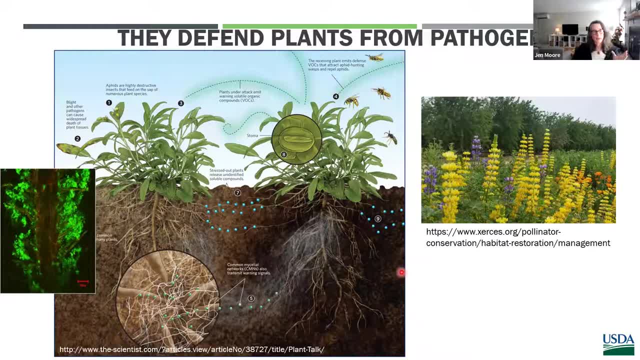 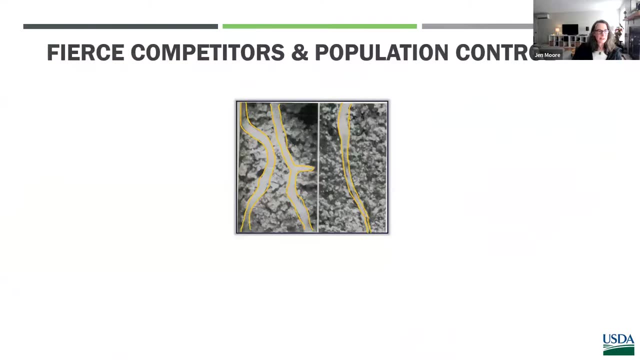 for the whole plan to work. So one way we can do that is to diversify plant pollinator habitats that will also attract these beneficial organisms that can help reduce pest and pathogen pressure. That's really super cool. These are just a reminder of the fierce competition. 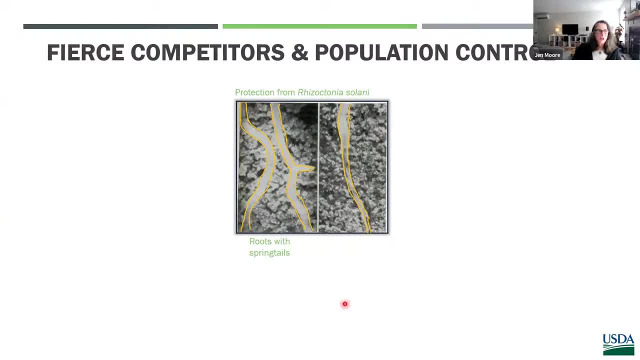 and population control. that naturally happens in soil. First, this is just an example of roots grown in the presence of a particular pathogen, Rhizoctonia solani. On the left-hand side, the roots are grown in the presence of these organisms. 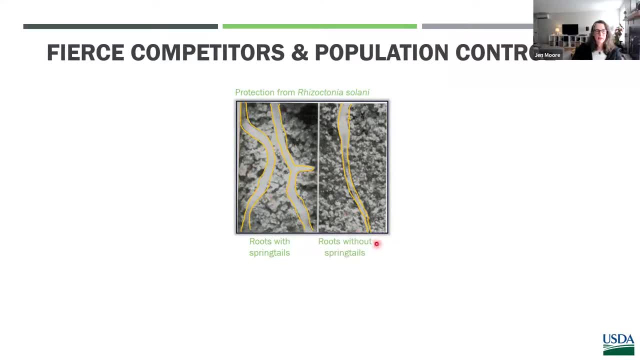 called springtails. On the right-hand side they're grown without springtails, And so another reminder that it takes a community And I'm not sure, the mechanism, but in the presence of these organisms the plant root is more healthy and able to resist and deal. 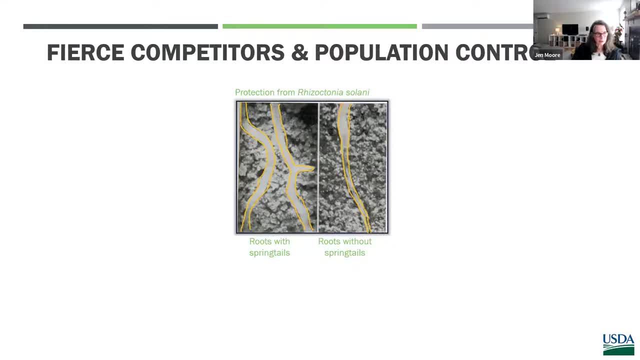 with the presence of this particular pathogen. That's one example. The nematode trapping fungi are so amazing, Right? So here we have this fungi, this little tiny thread-like substance. It creates a noose-like structure And in this case, the nematode's swimming through the soil water. 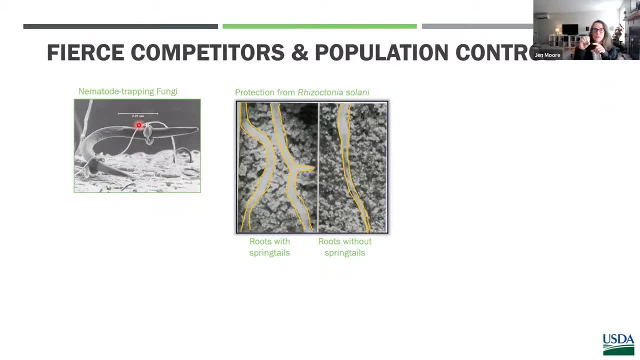 It's attracted for whatever reason, maybe a chemical signal that the fungi is releasing. It swims through the noose, Another chemical signal happens and it clamps down on that fungi and starts choking the life out of it. basically, So you can just get an appreciation. 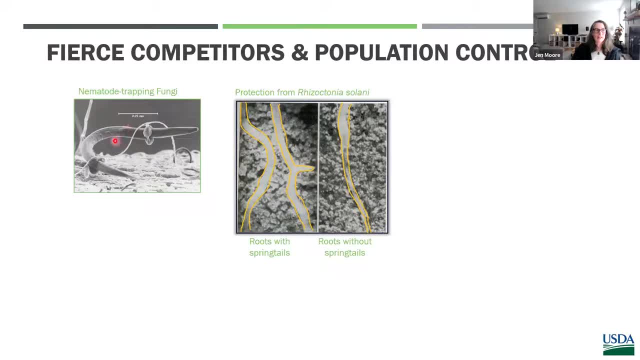 for the size of this tiny little fungi. Right, It's a fungus that is now attacking this huge nematode. in relation, There's another mite that's preying on a nematode. Nematodes are super important. They tend to get a really bad rap because they. 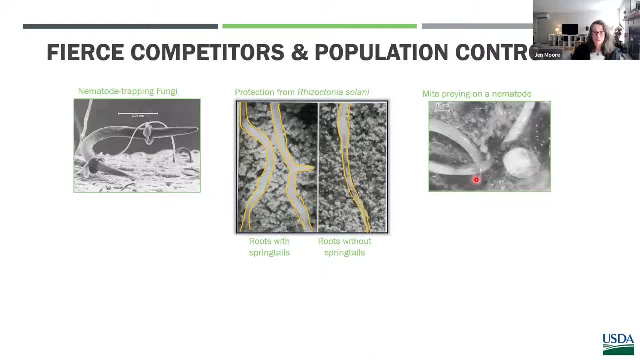 tend to induce a lot of crop damage, and rightfully so, because it causes millions of dollars of damage every year. However, the majority of nematodes are really important and really good for nutrient cycling And also they're involved- They eat everything. 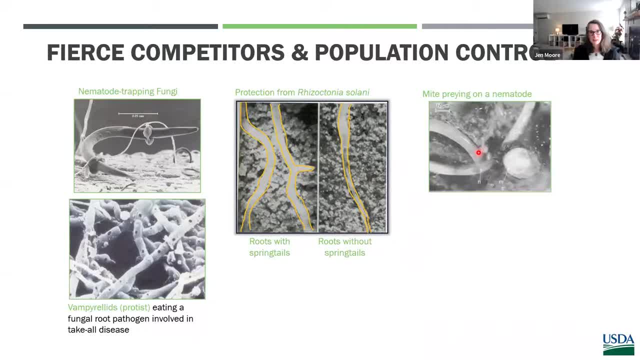 So they're also involved in population control. So keeping a nice, healthy balance of all of these organisms is really critical. I just like the name of these guys. These are a protozoa called vampiriliads, like vampires, And they puncture this particular fungus, that's. 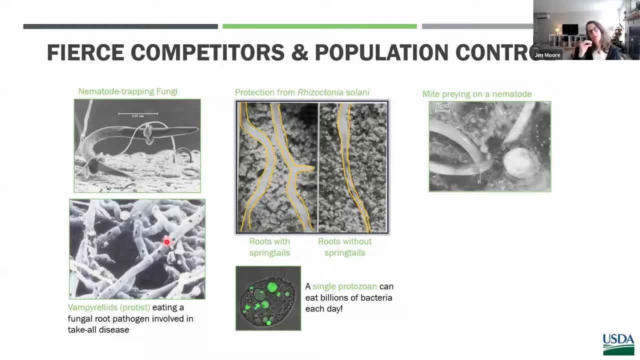 involved in take-all disease And they puncture it and start sucking the life out of that fungus, A single protozoan. they love to eat bacteria. So this is a single protozoan And again this green fluorescent dyed are bacteria. 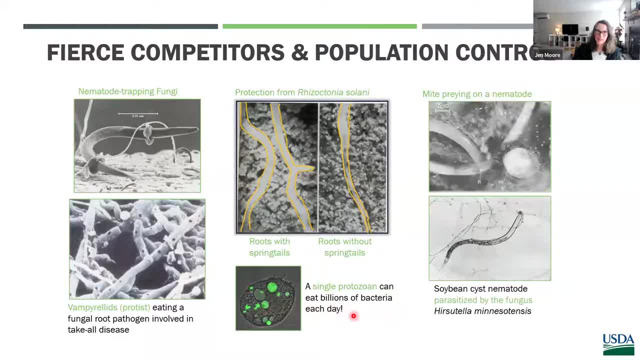 This individual can eat billions of bacteria in a given day, So very, very important for population control. And then this last example is a soybean cyst nematode, one of those bad guys causing major crop damage to soybeans, And it's being parasitized by this fungus that just 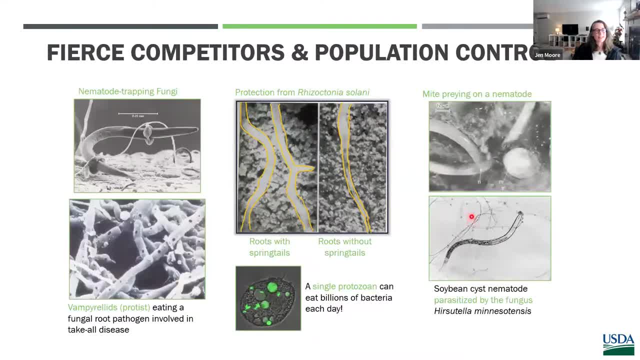 looks like some thread-like material in the soil, But it's killer. It's killing this particular nematode- So fierce competition. It really takes a whole community to keep everything in check. But when it's functioning well, there's a lot of population control. that happens naturally. 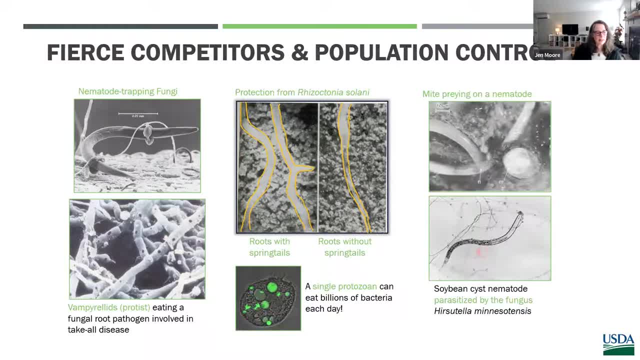 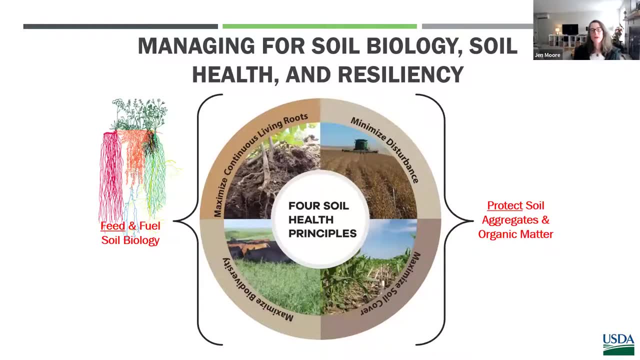 that we can rely less on certain pesticides to accomplish. So how do we do that? So hopefully I've just convinced you that this below-ground community, it's amazing, It's diverse, It's this active life force that's involved in every key soil function important. 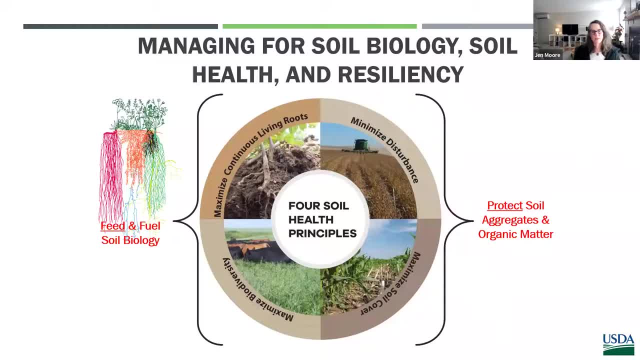 for agricultural productivity and numerous ecosystem services. So the next question is: how do we manage for soil biology, soil health and ecosystem resiliency? This was back from my days with NRCS. They have this great and really simple four principles of soil health- right. 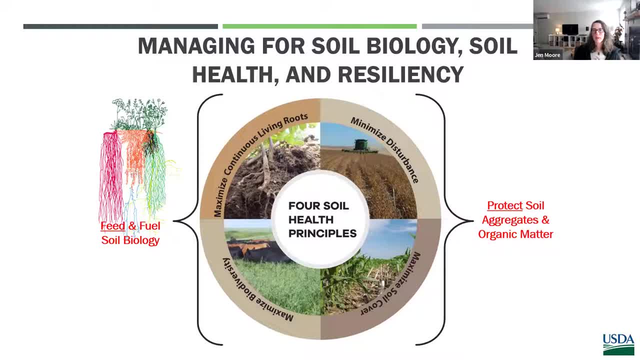 Minimize disturbance, minimize soil cover, maximize biodiversity. Sometimes people split it out. Right, They split it out with animals. I keep it in because animals are part of biodiversity And also maximize a continuous living root. I like to even simplify it a little bit further. 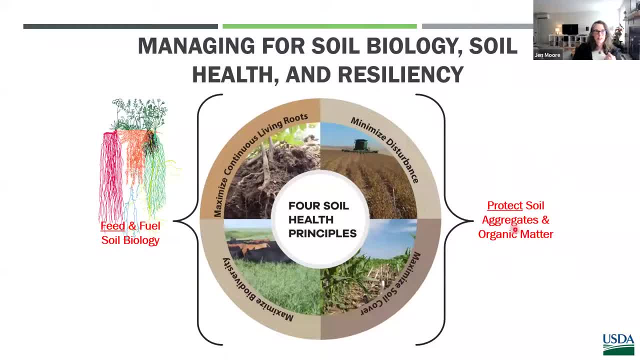 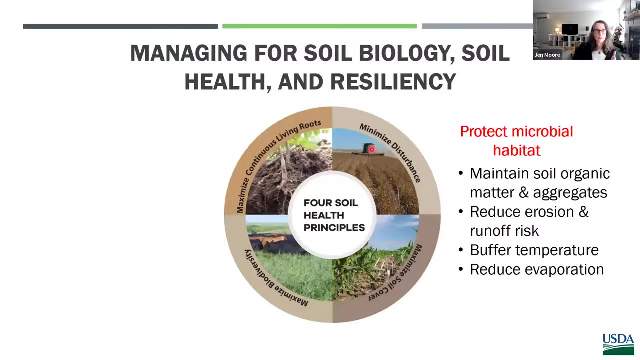 and talk about feeding and protecting. So the left-hand side is feeding and fueling that soil biology And the right-hand side protects soil organic matter and protects aggregates. A little bit more detail. So the first two principles: minimizing disturbance, maximizing cover. this is that armor of the soil. 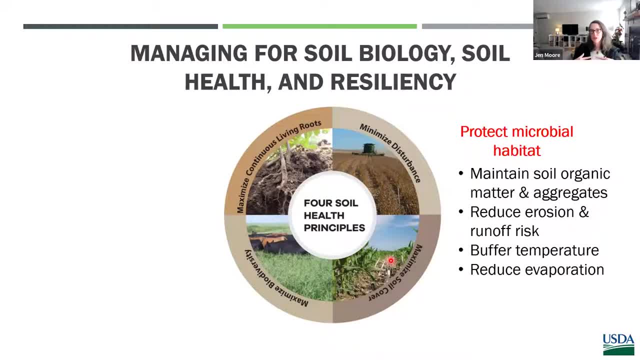 It's also not only protecting soil particles from erosion, It's also protecting that microbial habitat, those aggregates that Spider-Man helped to form, And the organic matter is not only habitat, but it's also fuel for the biological community, And so when we do this, these help to reduce erosion. 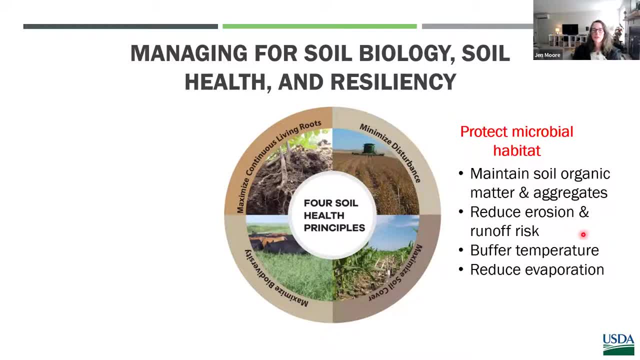 It reduces runoff risk. This keeps our soils, our fertilizers, our chemicals on site and out of waterways. Additional benefits include buffering soil temperatures, So we don't want major extreme temperature events to happen. Nature doesn't really like extremes. It doesn't do that well. 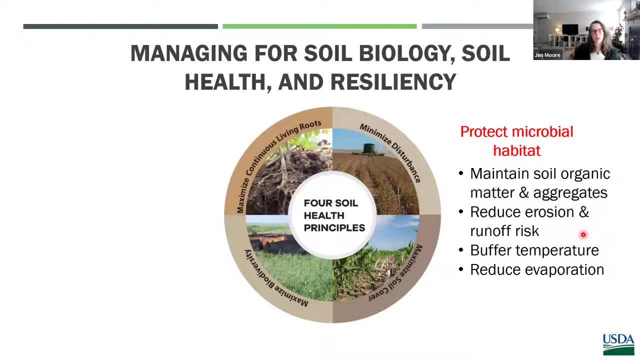 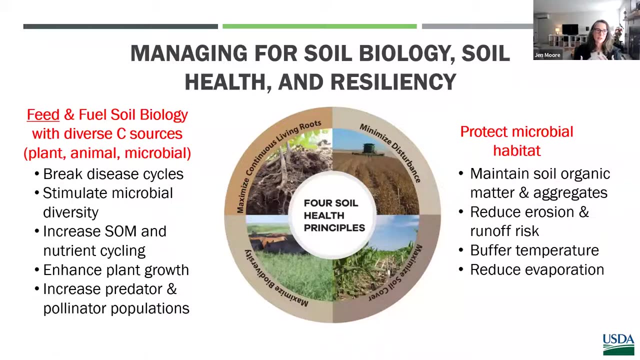 So it helps to buffer and insulate the soil from temperature extremes And it also reduces water loss from evaporation because we've covered the soil, Reducing that loss from the soil surface. The other two principles maximize continuous living root and maximize biodiversity. 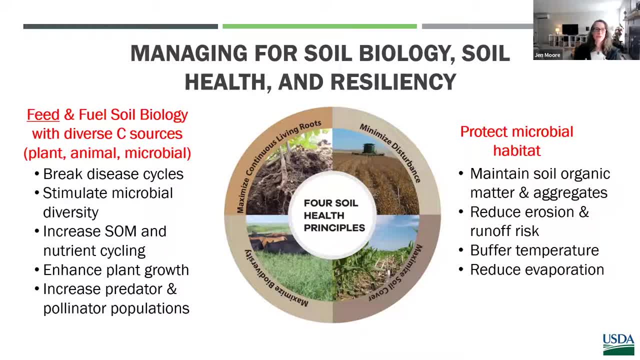 These principles aim to provide diverse carbon sources and biochemicals that fuel those soil organisms. So the other side doesn't really provide any new inputs. The left-hand side is where we need to provide those inputs to keep that system, that engine kind of running. 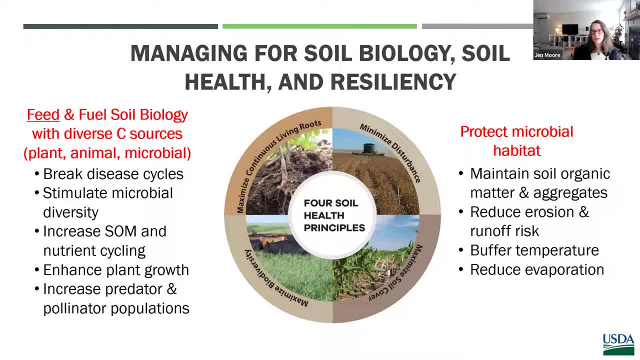 And so this stimulus, This stimulates the plant-microbe interactions that I talked about. It can help in resulting in breaking disease cycles, increasing- not just maintaining- soil organic matter, enhancing nutrient cycling and enhancing that predator and pollinator population I mentioned. 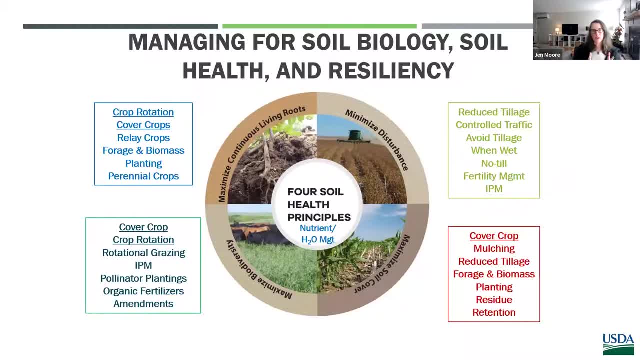 So it's important to develop soil health systems rather than target single issues. With a systems approach, the underlying cause of the problem can be identified and addressed rather than just addressing the system. So, although immediate action may be warranted to reverse concerns like erosion or salinity, not on the side of the mountains. 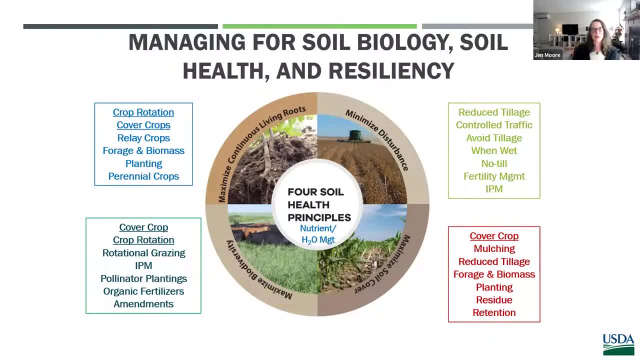 but long-term management strategies that can regenerate the system are needed. So listed here are some management practices that support the four soil health principles, And although adapting a single practice may be a benefit, the best approach is to couple as many as possible to develop a whole system that addresses 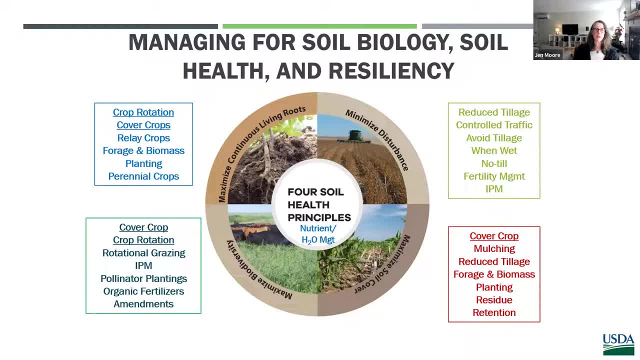 all four principles, So collectively. a soil health management system would stimulate below-ground changes to the soil microbiome. that translates into optimized system functioning and thus ecosystem resiliency. So this is especially, I think, important in the face of increasing weather extremes due to climate change. 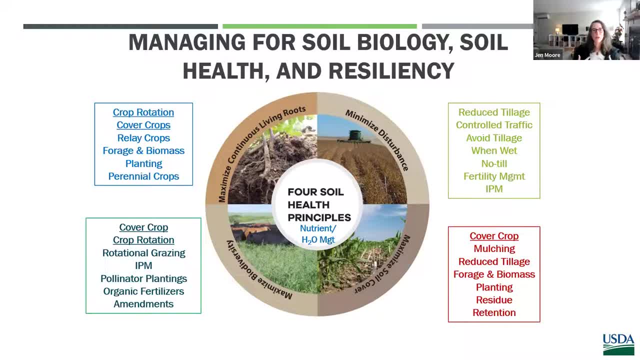 such as drought, intense storms, increasing temperatures, shifting those growing seasons, the reduced snowpack and spring melts that the Pacific Northwest is facing And, of course, more frequent and intense wildfires. So the more resilient our system, the better able we're both able to resist the impact of one of those threats. 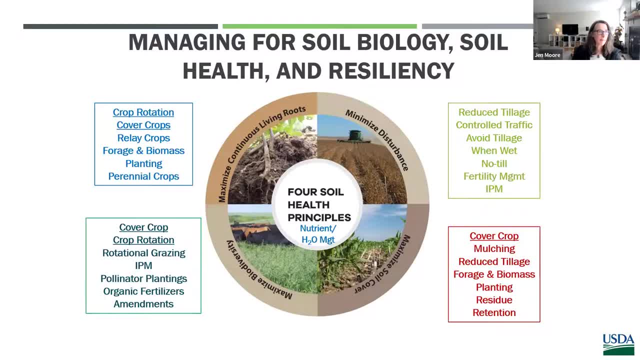 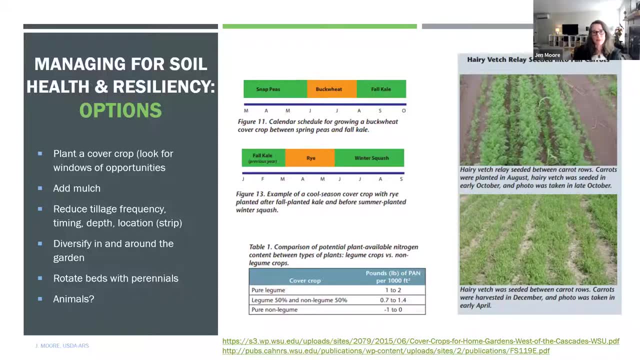 and, when it does happen, to bounce back more quickly. So what are some examples, what are some options for you? So planting a cover crop, that's one of the best. It's also one of the more common initial starting points that people like to do. 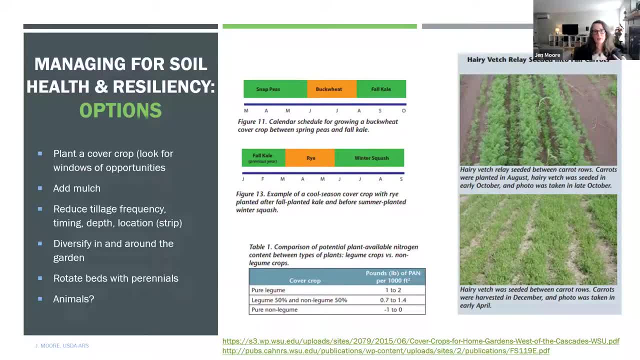 to use, And I would encourage you to look for windows of opportunities both in summer and winter, depending on what plants you're planting, And also windows of opportunity where in your landscape. So on the right hand side, here is a hairy vetch- that's relay, seeded between carrot rows, and that. 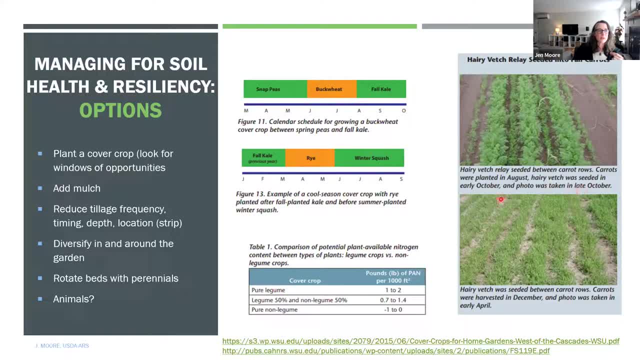 it's showing that the carrot were planted in August, Hairy vetch was seeded in early October and the photo was taken late October. And then here's the hairy vetch that again was seeded between the rows, and the carrots were harvested in December. And then this is just a reminder. 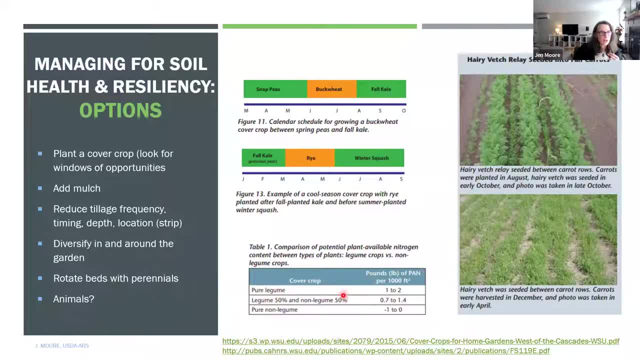 that when we plant some type of legume, like as a vetch, we do release some amount of nitrogen. This is plant available nitrogen in pounds per 1,000 square foot. There are two great references here. Cover crops from home gardens west of the cascades. it's a WSU publication. 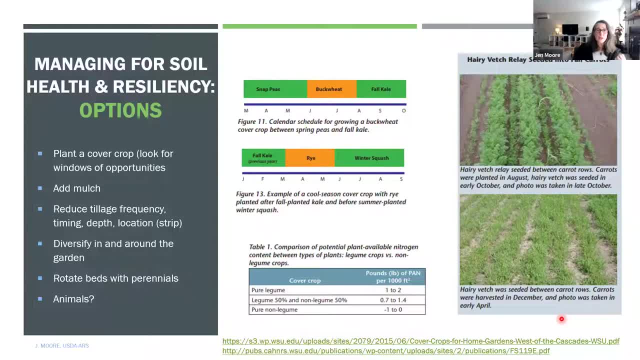 One of our OSU scientists, Nick Andrews, contributed to that from Oregon, And then another one that kind of talks about managing cover crops for the home gardens is listed here. Mulch is your friend if you're trying to reduce tillage, which again disturbs the aggregates. it breaks up things. 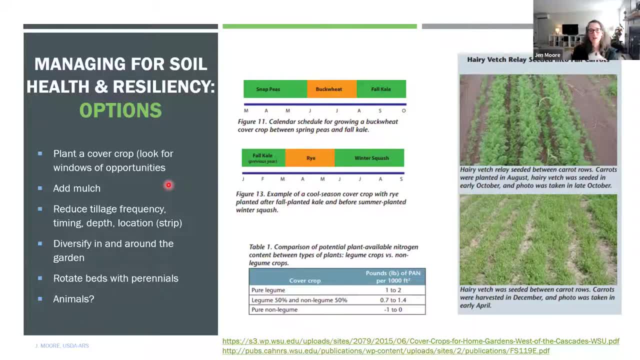 releases more carbon to the atmosphere and it destabilizes your soil, those big channels that we talked about earlier. Sometimes it might be necessary to do some form of tillage, but adding mulch can help you take steps to reducing tillage, maybe just tilling in little strips. 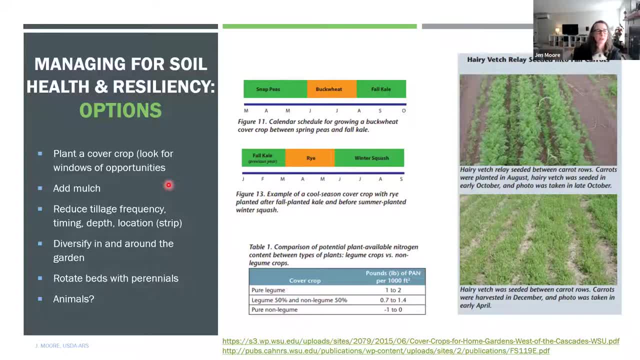 and working your way up to a full no-till system. Anything you can do to reduce the frequency, the timing don't till when it's too wet or too dry, how deep you go, and then the location- All of those things can be steps in the right direction towards a full soil health management. 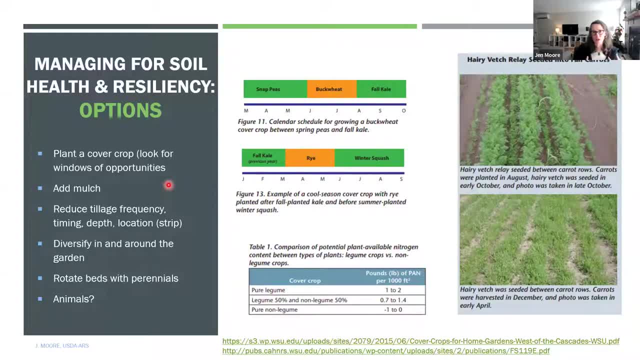 system. Diversify in and around your garden or your field. Don't forget about borders. Those can be really valuable areas to look at. Consider rotating beds with perennial crops, as you can rotate out different disease cycles, for example, and then you just 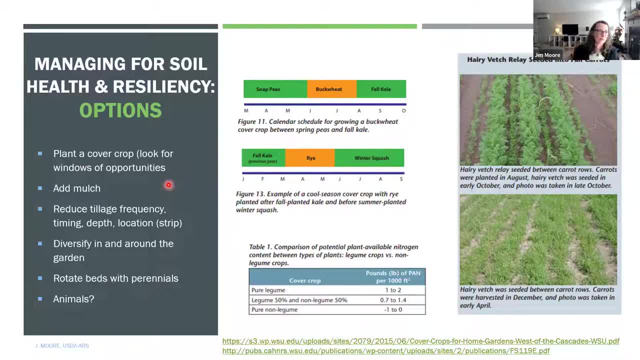 help to re-set the stage, if that's something that you can do. Animals are a great integrative tool. Of course, if we're talking about vegetable production, you need to think about human safety with that and timing, and I'm not an expert in that, but there are lots of good extension. 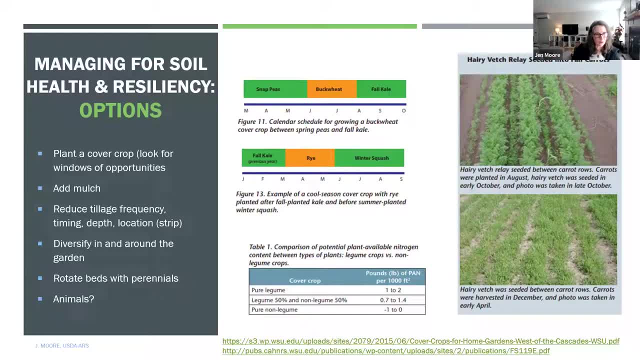 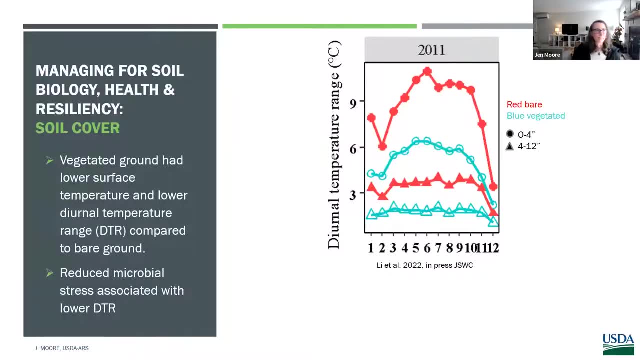 publications on that to help you with that, But they're a really great tool in the garden as well. You're doing great, Jen. I think we only have about three questions, so I think going all the way to 350 is fine. Okay, so this is just some examples of what happens in. 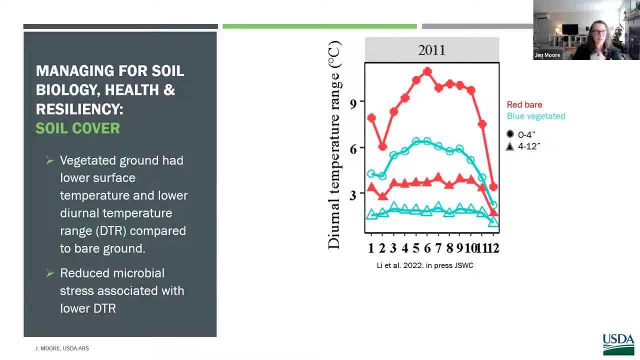 managing for soil health and soil cover. I just wanted to emphasize there's soil temperature and then remember those extremes in temperature. So diurnal temperature range is the difference between the max and the min on each day And what we discovered in Texas in a lot of the work that 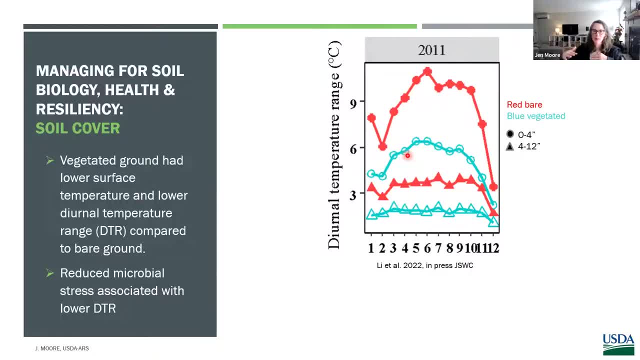 we were doing there is that it wasn't so much the average soil temperature that mattered for plant stress, it was that big range in temperature swings. So in our bare ground this is you know how much of a difference between min and max we had versus the vegetated ground. So this is the 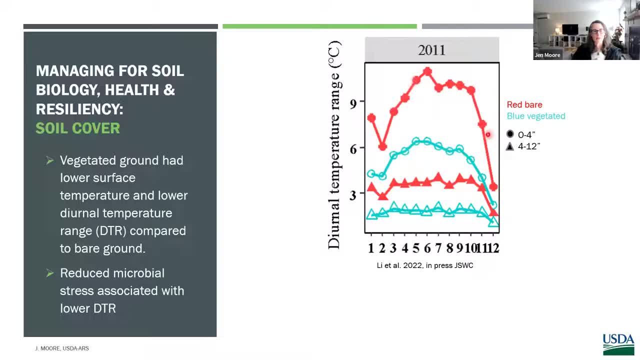 surface top four inches and you can see the bare ground in red was much higher than the ground in the soil. It's much higher, this diurnal temperature range, than the vegetated surface. and then that persisted down about a foot into the soil And what we found was that it was the lower the DTR. 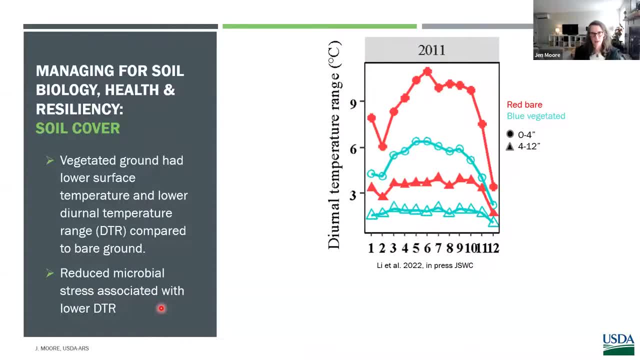 the lower the microbial stress and the lower the plant stress, So the more vigorous and healthy plants were as well. So just another layer of information that we were finding really interesting. And then in I gave this talk to some viticulturalists and they recognized that cool soils may be an advantage in warm climates because they can slightly delay ripeness and that could enhance certain flavors. 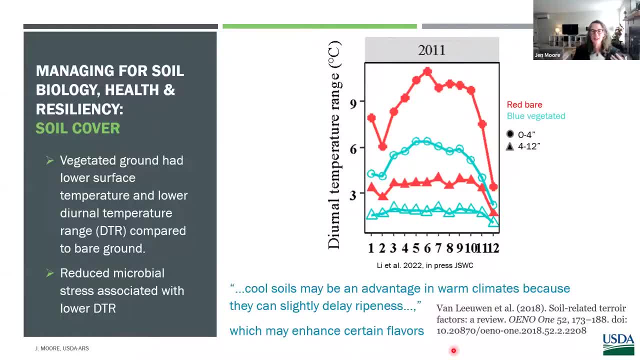 So the terroir of soil is related to all of these things: the microbes, the temperature interactions, the moisture, etc. And so how we manage for that can have an impact not only on our yield but on the quality of the fruits that we're generating. 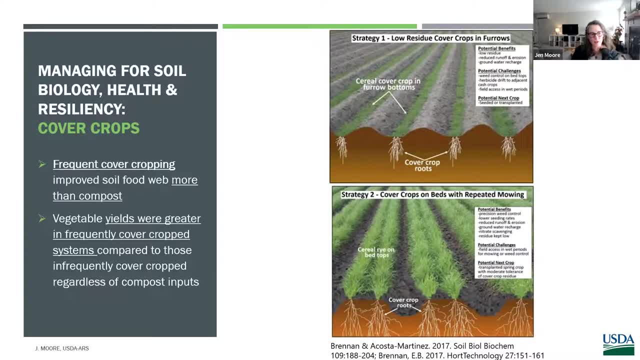 This is a great publication by USDA ARS scientists. This is work out of California again, where they're looking for unique ways to incorporate cover crops into vegetable systems. And so you know you can plant cereal rye in the furrow bottoms in this particular case. 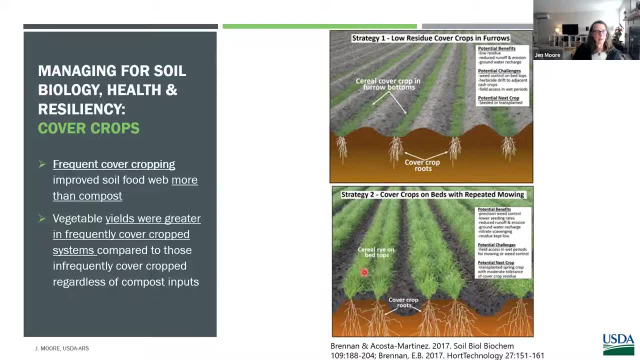 Or these were cereal rye in the bedtops and just different ways to incorporate. look for unique ways to get cover to protect those areas. One thing that was interesting is that they found that the vegetable yields were greater in the areas that had more cover crop, more frequency of cover crop. 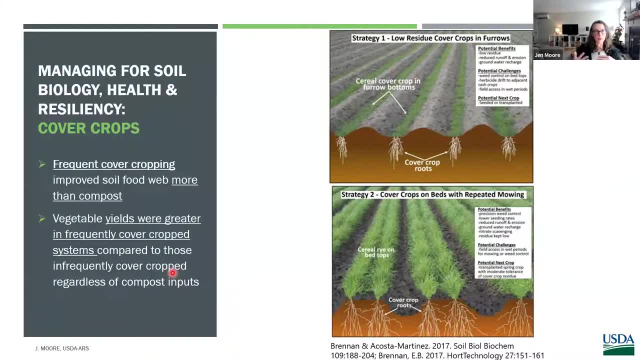 than those that were just that were less frequently cover cropped And that they were also greater And that they were also greater yields than compared to just mulching with like compost or something. So that living root was really important to help again make that vegetable system more resilient and more productive. 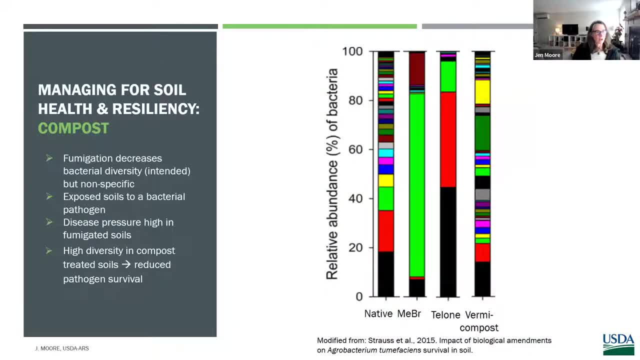 So that's an example of that. This one comes up just about fumigation, Probably not really relevant to home gardeners, but the takeaway message is that each bar is a different type of bacteria. So the more bars, the more diverse the system. 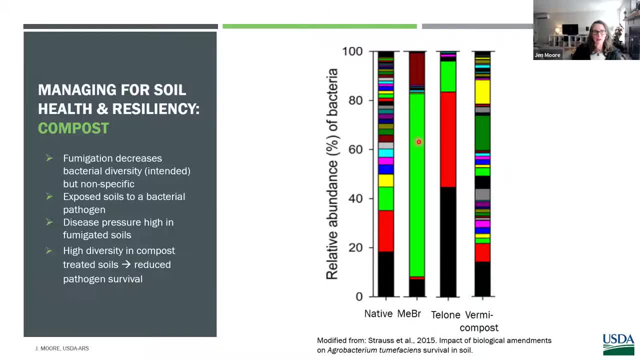 So this one's a native system And this is what the population looks like. These two bars are two different types of chemical fumigants to combat one of the pathogens. So you can really see that you know it knocked down the diversity of the soil. 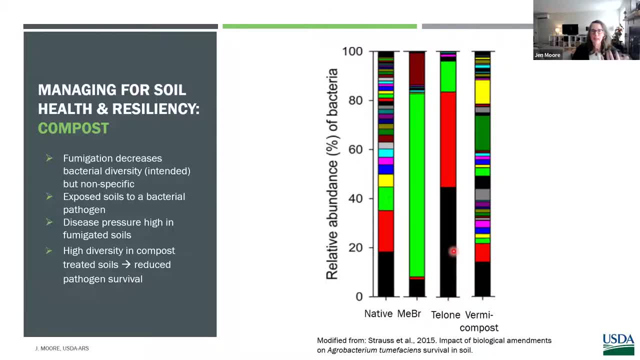 It temporarily knocked down the pest, But what they found was that that pest then just bounced back. What they found even more compelling was vermicompost, So that's composting with worm castings, And when they added this to the soil they were able to keep and maintain that diverse population. 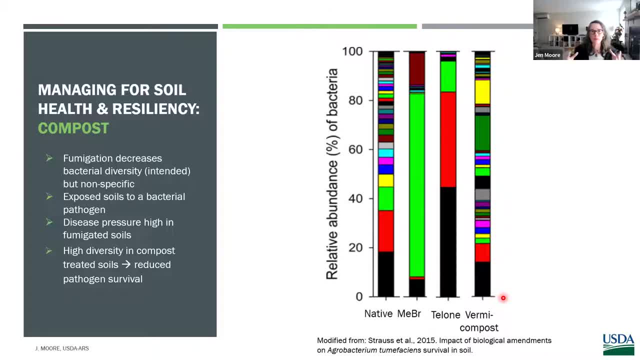 And one of the organisms, or a whole group of organisms, was able to then combat and minimize the impact of that pathogen in the soil. So the point is is that sometimes there's really cool organic amendments, such as vermicomposting, that can achieve the same thing. 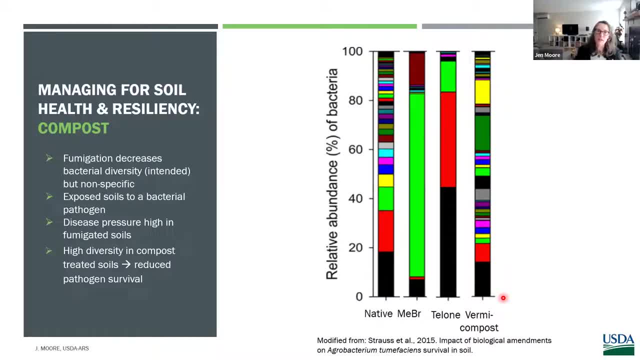 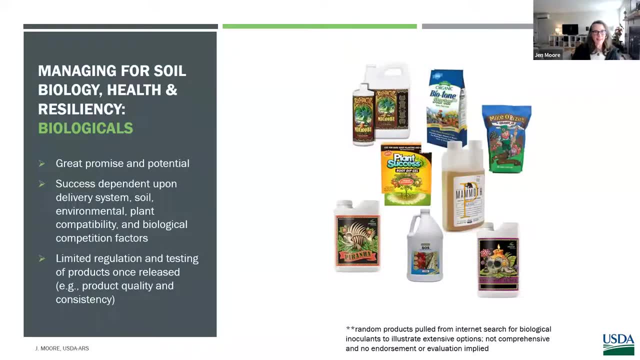 Without the environmental negativity of, in this case, chemical fumigants. So I just found that to be very interesting. And then that always leads to questions about: well, what about adding biologicals to the soil? You know there's like bugs in a jug. or you know different amendments that have been promoted. 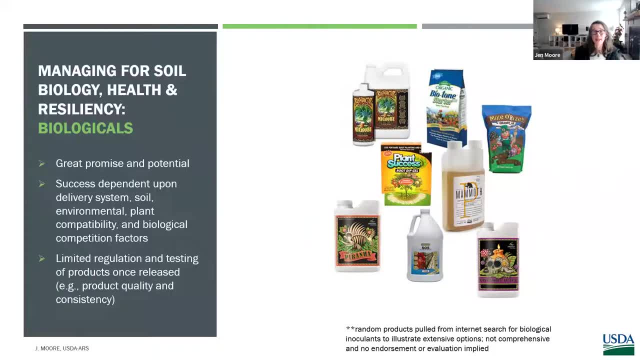 And some of them work and some of them don't, And part of the issue is that they're not very well regulated And there's not a consistent standard that people can rely on. I think that there's great promise and potential in these products. 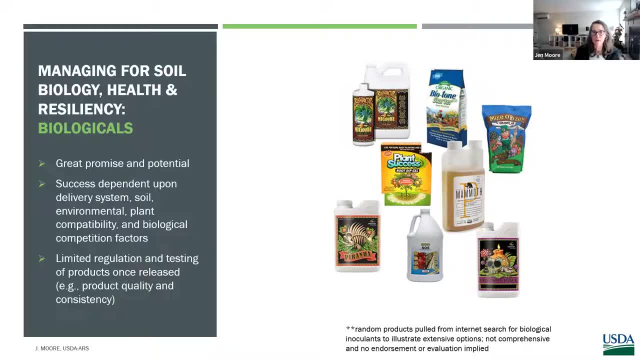 And so if you try them, I would maybe not go all in on them, but try them in a portion of your field. Set up a nice trial with the control and see if they're worth the money, because they're often quite expensive. 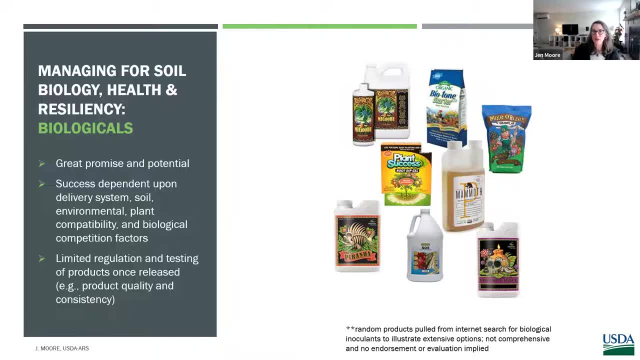 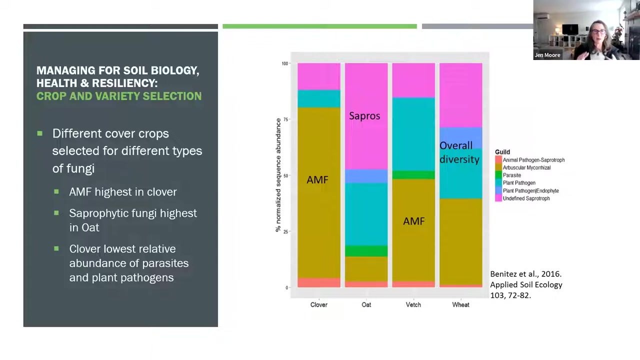 Hopefully, you know, with more research and more effort in this area, we'll be able to identify certain pathogens, Sorry, certain populations of beneficial bacteria and fungi that can help stimulate plant growth and knock down the bad guys. And then- this is just a reminder- that, depending what we plant, 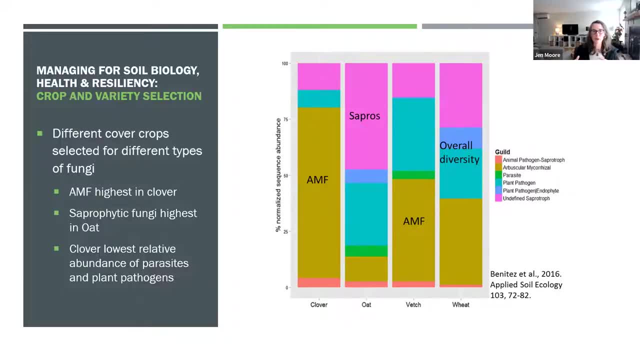 we can change the composition of the microbial community just by changing the plants we grow, And so these are different cover crops: clover, oat, vetch and wheat. Again, the different bars are different types of fungi in this case, And so the clovers really stimulated our muscular mycorrhizal fungi. 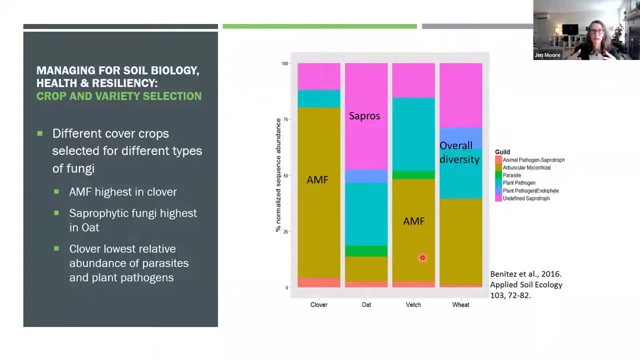 Same with the vetch. So these legumes really stimulated that symbiotic mycorrhizal fungi association I mentioned earlier. Other crops like wheat just kind of had greater diversity And the oats kind of stimulated the saprophytic fungi. So these are different types of microorganisms that break down dead stuff. 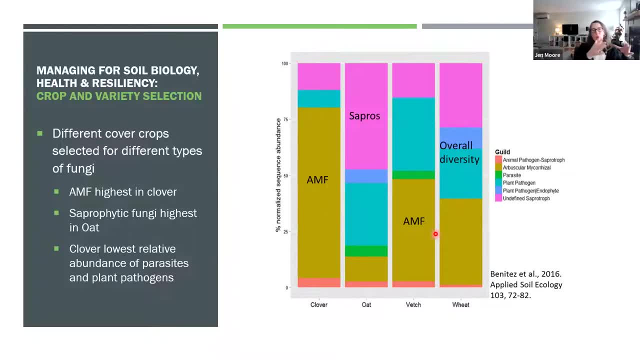 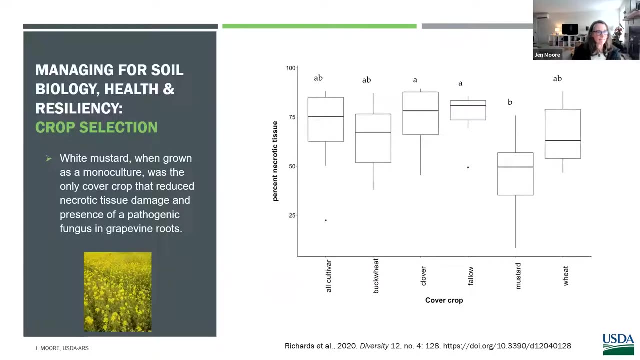 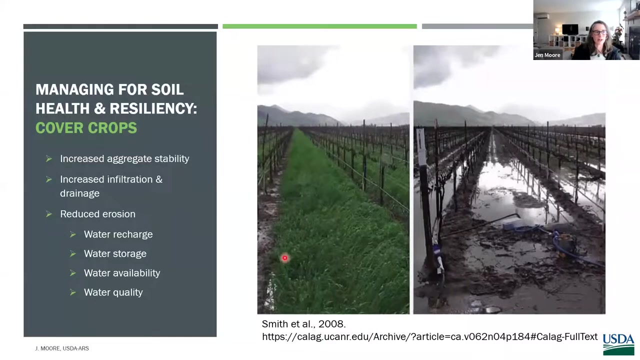 But the point is: is that by mixing and introducing new crops into your rotations, in your rows, in your cover crop mixes, we can help stimulate and change and diversify the population for the better? I'll skip that one, Okay. And then this one is just a reminder again. 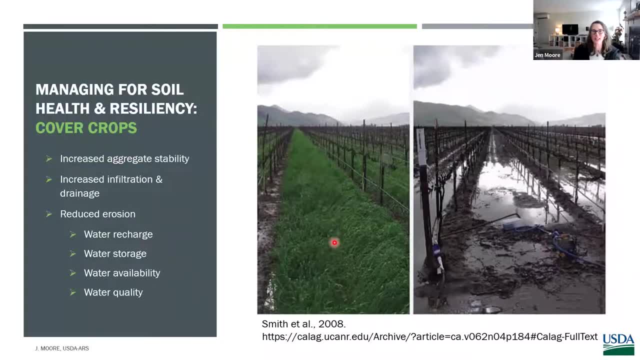 of the benefits of soil sustainability: Cover protecting the soil. I think a picture says a million words, in this case, right. So on the left-hand side, this is a vineyard with a cover crop. The right-hand side, no cover crop following a winter rain. 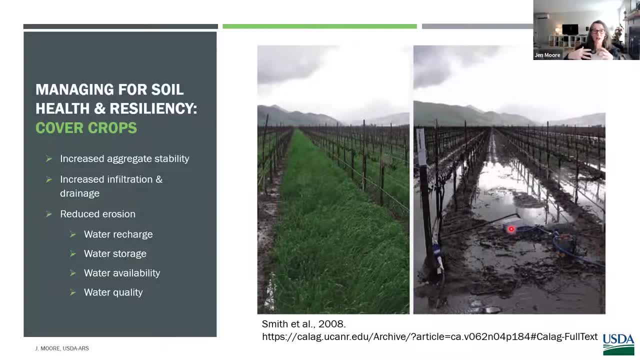 So you can see this soil is not well aggregated because the water is not going in, It's ponding on the surface, It is running off, It's evaporating off, It's not getting in the ground where the plants need it later on. 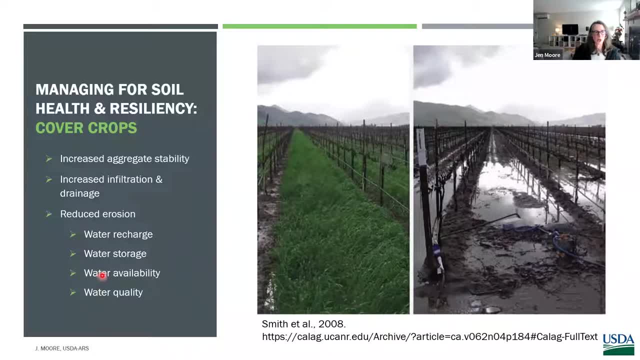 And so really important for water recharge, water storage, water availability and water quality. So anytime we can avoid this is a good thing for lots of reasons. Even fish populations right, we can talk about Really important stuff. And then there's that Spider-Man helping to aggregate the soil to help resist that erosion. 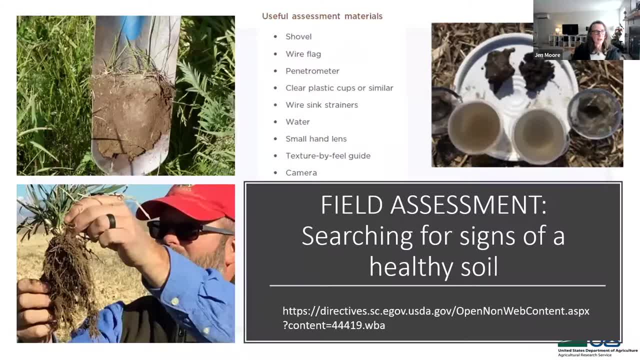 and get the water in. Okay, And then I'll just end with this and a couple of slides. There's a whole guide put out by NRCS. I helped to develop it before I left. It's a field assessment. The website is listed here. 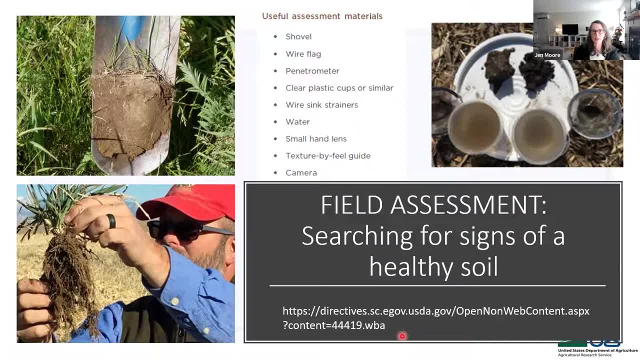 It requires no fancy equipment. It requires no expensive equipment, just your hand, a shovel and some things you can pick up at the dollar store if you don't already have them in your house. And it's a great guide. It kind of goes through. 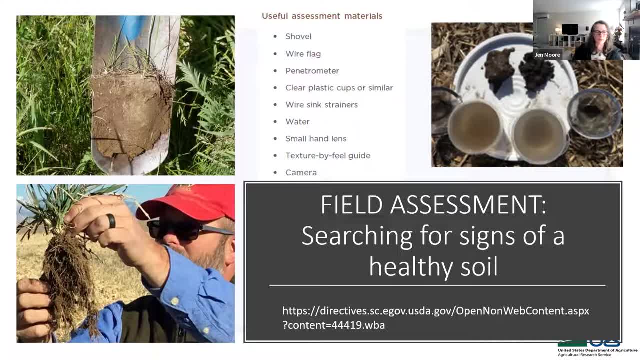 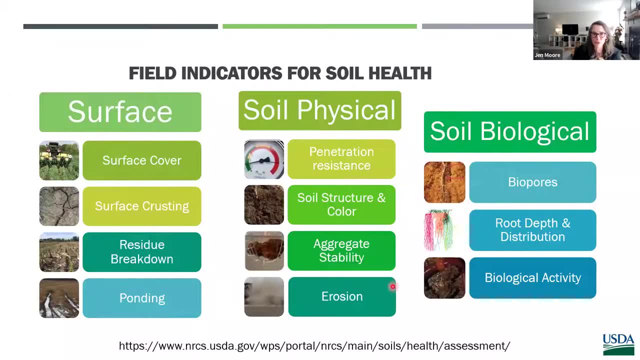 And it tells you if you have a soil health resource concern or not. I'll just kind of preview it that there are different indicators. You don't have to go through all of them. The guide will walk you through it, telling you what time of year to sample, how to do it. 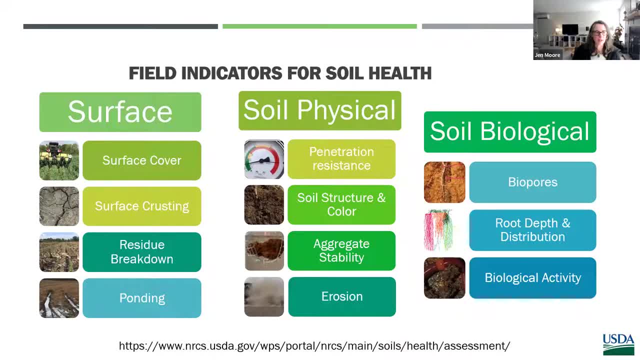 and what the implications of the results are. So surface things are: looking at cover, looking at surface crusting or cracking, looking at how quickly your residue breaks down or whether you're ponding water on the surface. Physical is this penetration resistance? 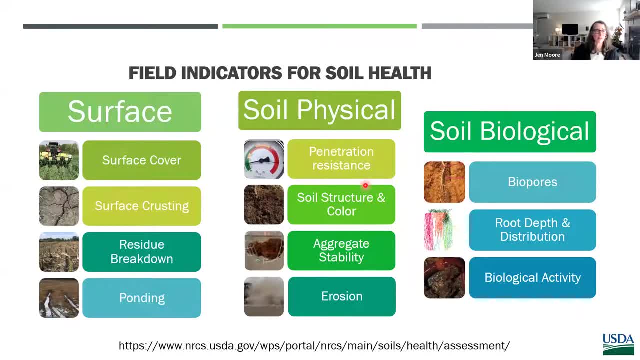 You can use a fancy tool or you can use a wire flag. The guide talks about that: Looking at the structure of your soil, the color can tell you a lot. There's a really fun way to do aggregate stability that the guide goes through. 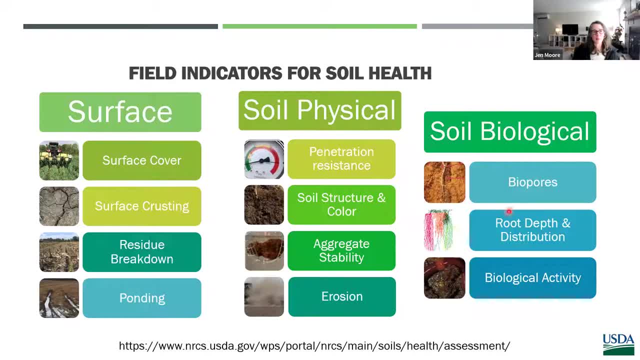 It's super inexpensive and easy. And then a couple of ways to look at the biological properties, those biopores, the big ones from the root channel, Or earthworms, what your roots look like And, if you're lucky, biological activity, although that's a little bit harder to see with the eye. 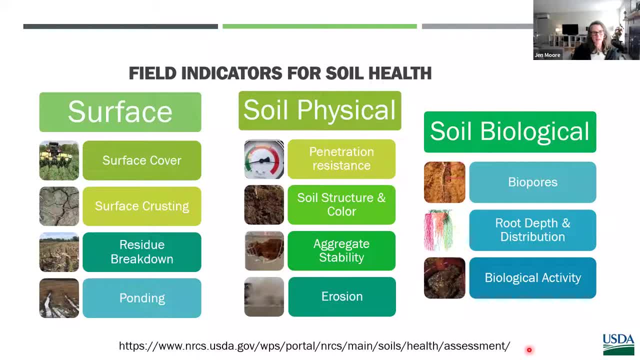 So this website is another link to it and it goes through it And I would be happy to help anybody. You can contact me and we could go over that later on. So I think I can end and ask and wait for questions. Is that a good stopping point? 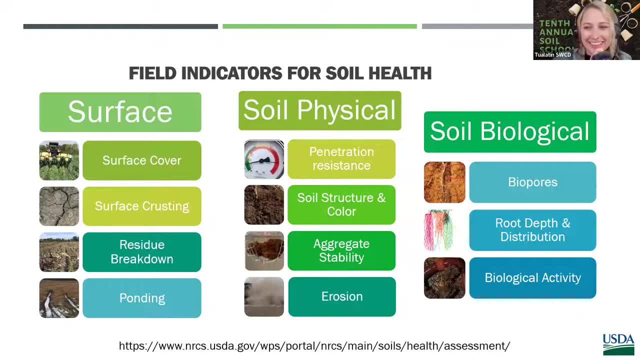 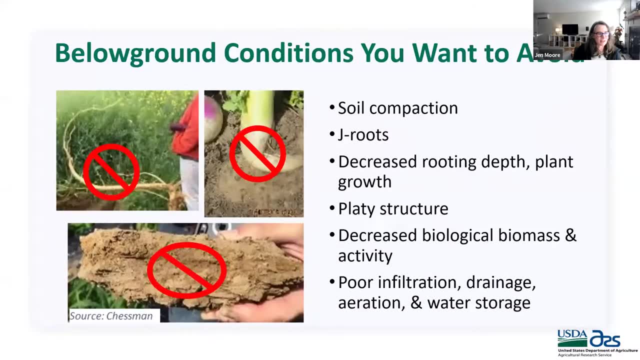 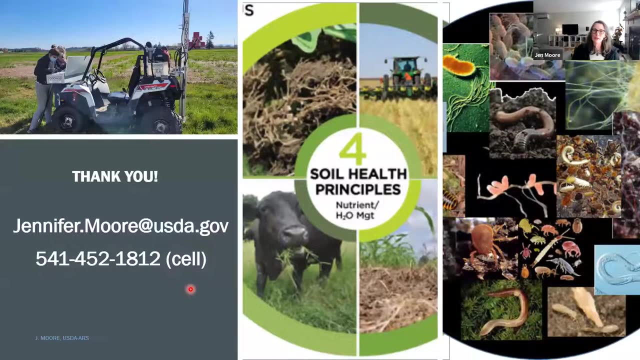 I think that sounds great. Okay, Yeah, I'm going to pull up my last slide here, So I'm just going to skip through these. This just kind of goes through a little bit more closely. But here's my email and also my work cell phone number. 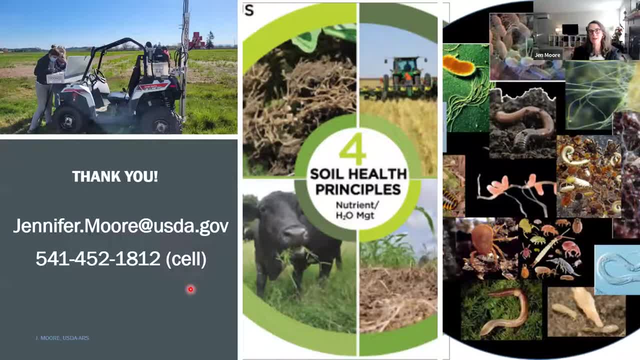 So if anybody has follow-up questions, I'd be happy to talk with anybody about designing a little study on your garden or your field at any point. Thank you, Very cool stuff, Jen. That predation slide was really neat, Oh man. 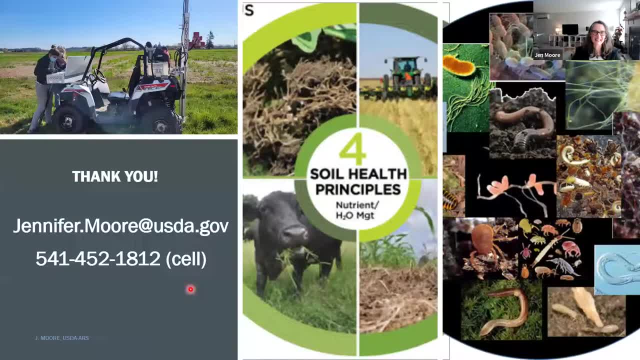 It's a cutthroat world down there, isn't it? Yeah, Yeah, If you believe in reincarnation, you don't want to come back a soil microbe, Oh man. Okay, So we have a couple questions. One of them, I think, I can answer easily by saying that these slides will be available. 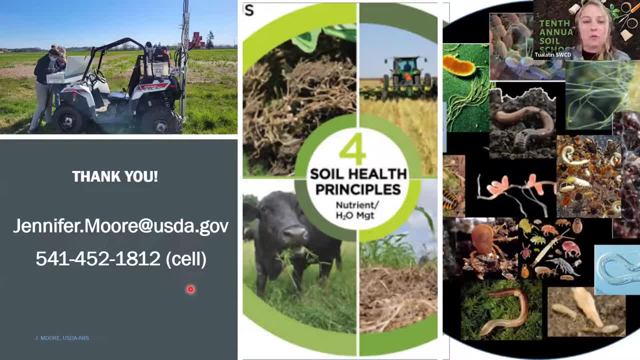 We'll be shared with folks. So I will follow up with an email to everybody. And so the key functions page, all these reports that she's referenced, these great resources, everything that's in this presentation, I will get into your inbox. 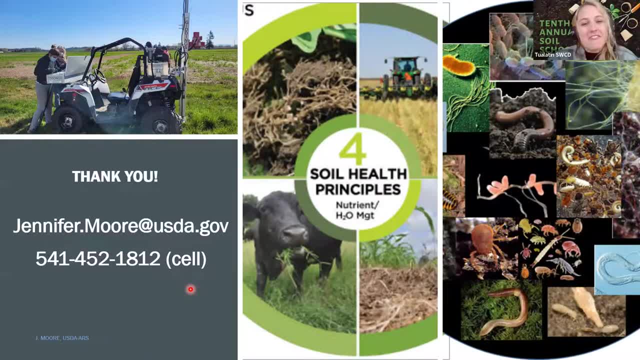 So, all right, this is a fun one. Jen, What is your favorite soil microorganism and why I have to pick just one? That's like asking me, like what's my favorite kid? I like actinobacteria. 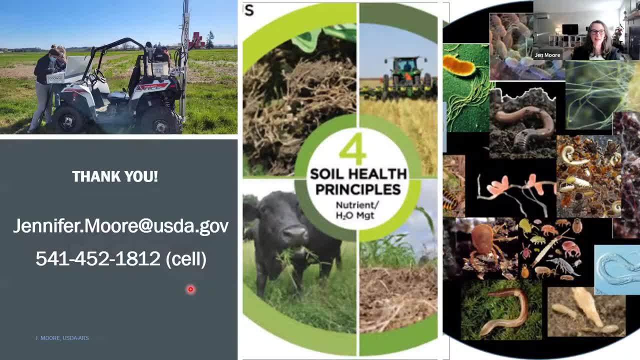 And one of the reasons is that they were sort of misclassified back when I was in school. They were kind of bacteria, kind of fungi, And then they discovered through DNA that they're actually bacteria And they're really important for breaking down. 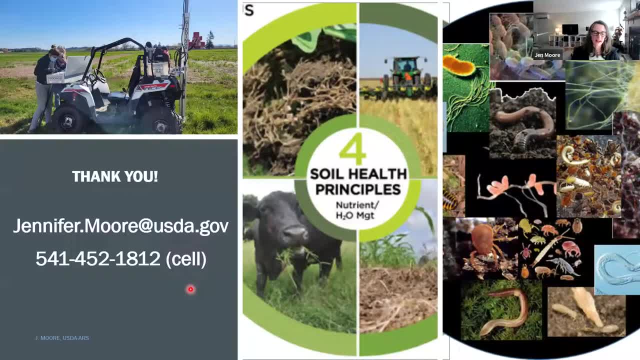 They're hard to degrade. materials Like woody material They're often common in. they're found everywhere. They can be in really high pH or arid environments. They're in our gardens And one of the cool things they also release is geosmin, which is a? is that earthy smell? 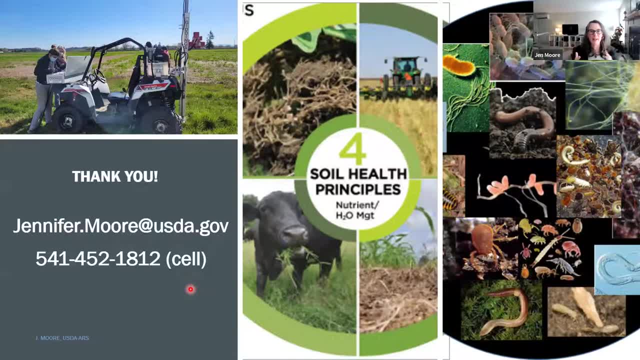 So you know, when you're working in your garden and you kind of get that earthy smell, The smell is from actinobacteria that are actively breaking down organic matter And they're releasing this volatile organic chemical called geosmin, And so it I think it's stimulating and it's a rich smell. 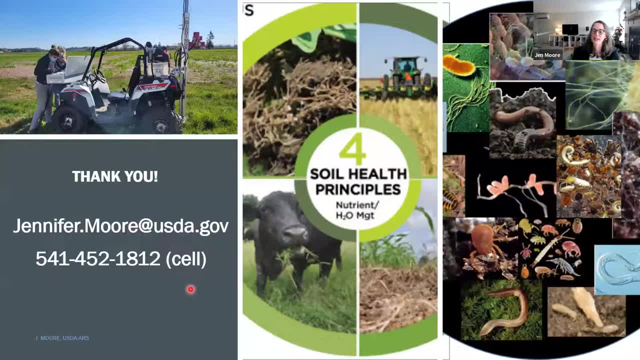 And I just think that they're super cool, So that's my favorite organism. I love that, And that actually gives me an idea for a question That makes me think of petrichor, Which is the smell that you get when it rains. 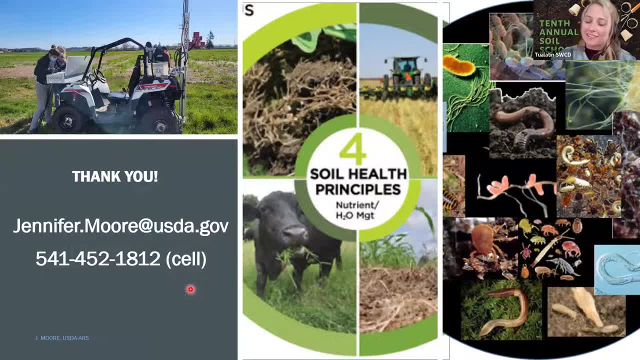 After it recently rains, And I was wondering if that is that related to anything happening in the soil. I don't know that term But I would, I would argue. I would guess that it's a stimulation in the flesh of a chemical, you know a biochemical that's released by organisms that are stimulated by that rain event. 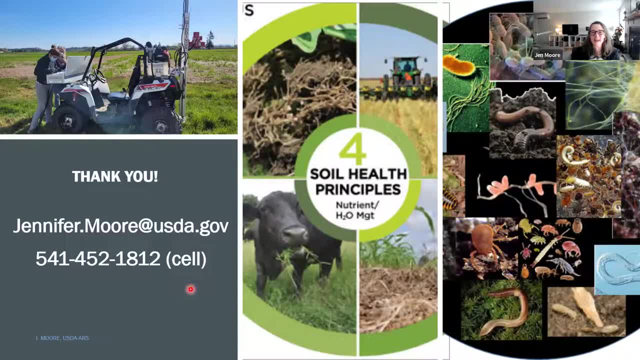 Yeah, I don't know. I know also, just on the smell thing, that there's a lot of work in gardening and how it's. there is like a true biochemical signal in our brains that it makes us happy right to dig in the soil. 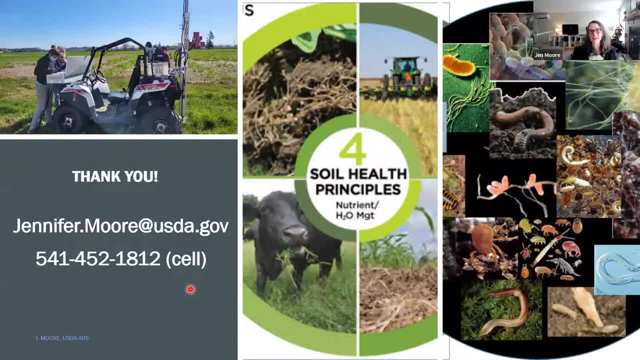 And so they use it for therapy and all sorts of great things. So it's it's not only good for, you know, feeding us, but it's also good for the mind, So I wanted to point that out too. Absolutely. 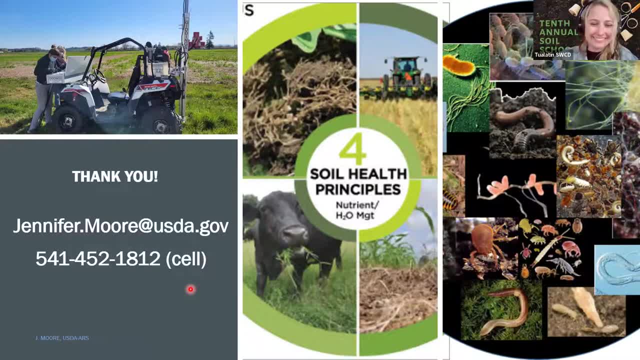 Grow your own food. It's good for the planet and good for you. Okay, And I'll say one more thing: that smell. we used to include it. It's in one of the former soil health field assessments. but the smell of your soil can also tell you something, especially if you're adding a lot of compost and organic materials. 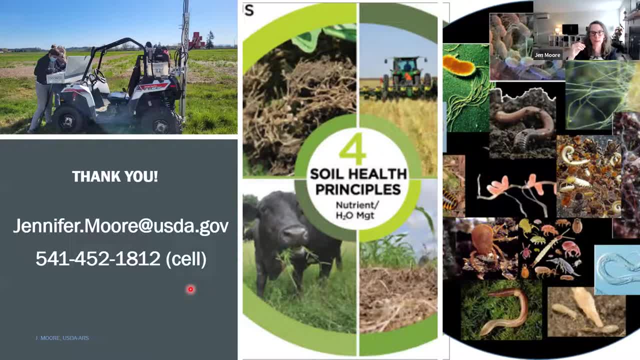 It can go anaerobic on you and you don't really want that to happen. so you need to aerate it a little bit or add more coarse material. So if your, if your soils are smelling kind of acid or you know, like yucky smelling, 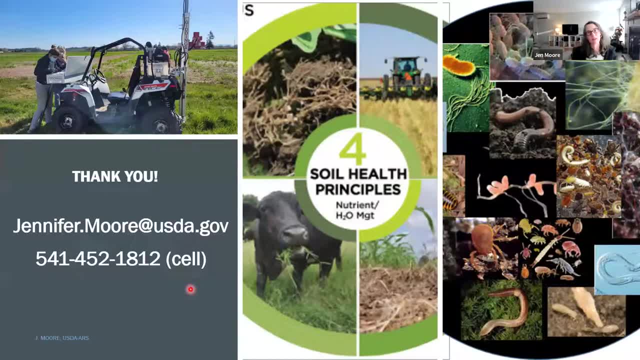 That's a bad sign, but that nice earthy smell is a good sign of a nice, healthy, active population. Okay, we've gotten several more questions that just popped up. So let's see: If you plant cover crops in the fall, winter, What do you do with them in the fall? 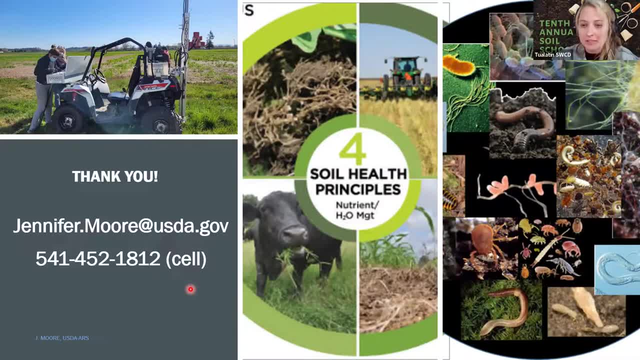 What do you do with them in the spring when you want to plant your vegetables? Yeah, so that guide I showed talks about that specifically. each cover crop and each crop you're planting has different timings, So there's different ways that you can go about killing the cover crop. 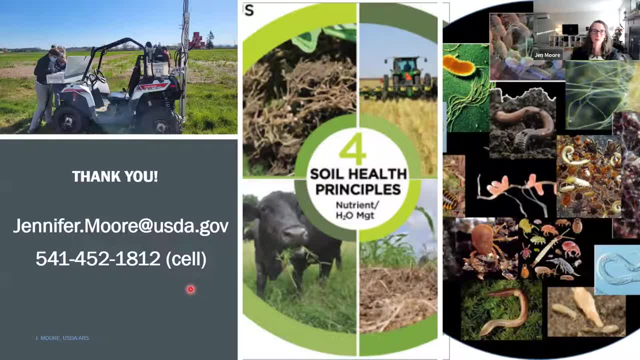 Obviously you could chemically kill it, like with Roundup or whatnot, Depending on the size. some people like to roller, crimper it, So you can get like a big barrel of what you know something full of water and and roll it over. it depends on the size. I'm assuming this is a small garden. 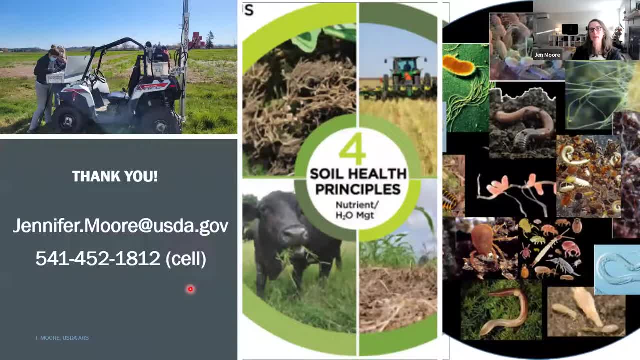 You know you could mow it. You could have some animal eat it. There's lots of ways that you want to kind of knock it down right before you plant into plant your veggies, And in that case again, you can do strips instead of tilling the whole thing under. that would be another option. 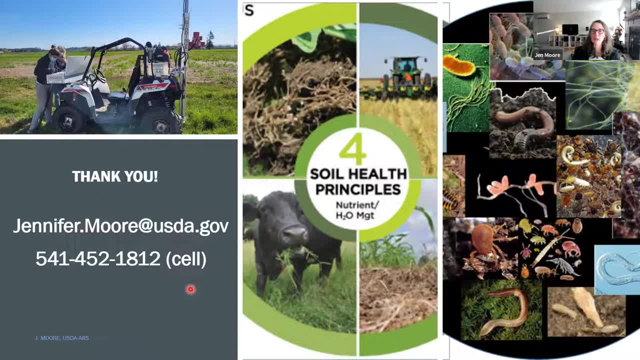 And in that case again, you can do strips instead of tilling the whole thing under. that would be another option. But if we can avoid tillage It's better. But you know, might take some some practice there. so there's lots of different tips and tricks in the man at the second reference on that one slide talks about managing cover cops for home gardens and I would highly recommend that one on a similar subject. 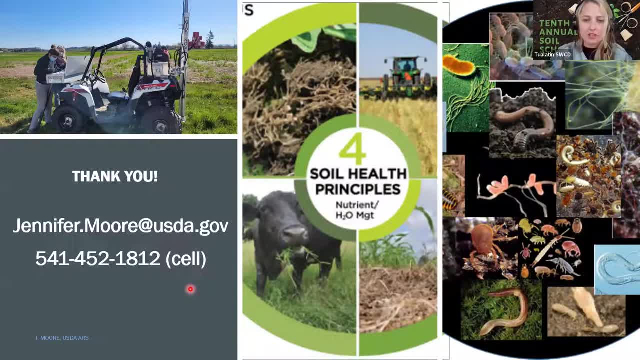 On a similar subject: do you have any suggestions for what cover crops are well suited to home gardens? On a similar subject: do you have any suggestions for what cover crops are well suited to home gardens? The first one talks about that one. Yeah, Yeah, And there's also. I can send it in an email and 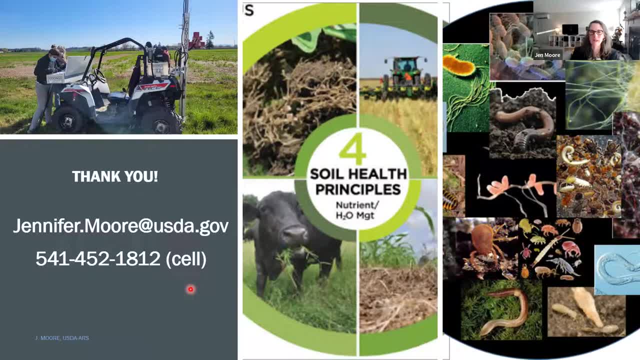 you can, or I'll try to add it to the slide before I send you the slides. The NRCS at the Plant Materials Center here in Corvallis, Oregon, has a cover crop selection tool And it's really easy to use And you kind of put in your criteria whether you want it for biomass or for weeds or 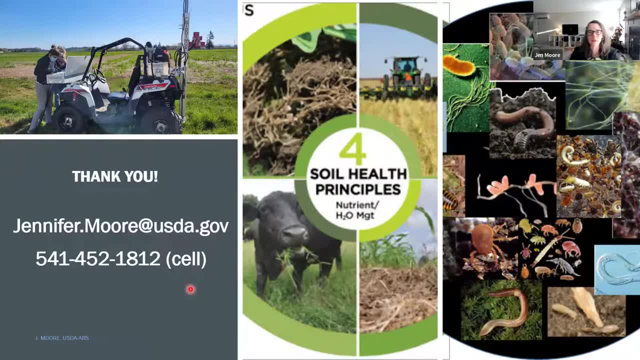 for nitrogen And it tells you which crops you can choose. And then another great resource is available through SARE- Sustainable Agriculture, Research and Education- managing cover crops for profitability- And that's a free resource And I can provide a link to that when I send the slides. 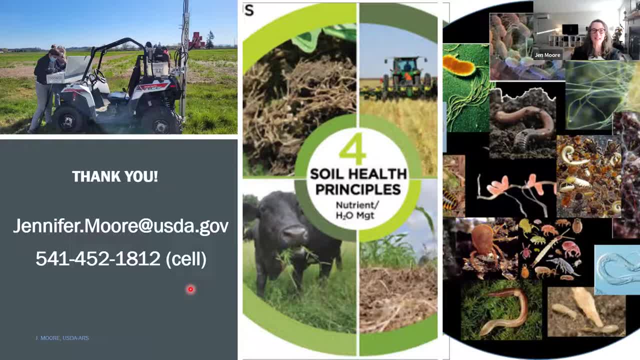 in. So it really depends. The cover crops are amazing and they're frustrating because there's so many functions And unfortunately it's the cop-out answer of well, it depends. It depends on what your goal is. There's different camps of whether you go all in on a really complex. 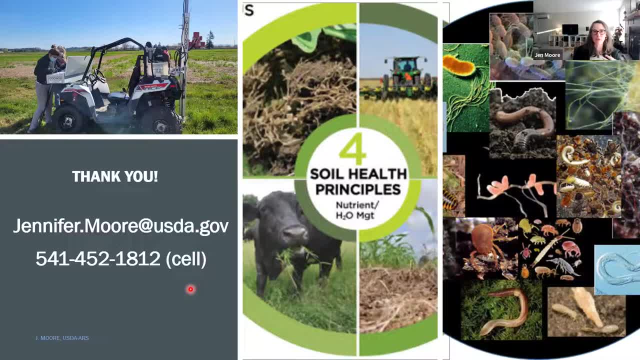 mix, or you try to gain a little bit of successful operation with one or two species. The more complex, the harder it is to kill non-chemically, Because they all kind of mature at different times, And so you kind of have to ask yourself: 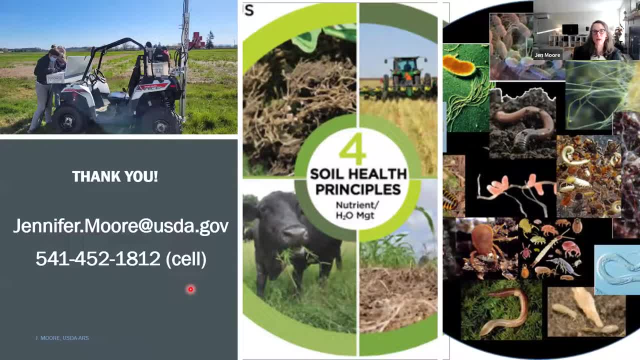 what do you want to do, What's your main goal And then what grows best in the region that you're at? Yeah, Yeah, we've got quite a bit of questions that are a little bit specific, So I think including those resources in the slides will be really helpful to folks Specifically, if you 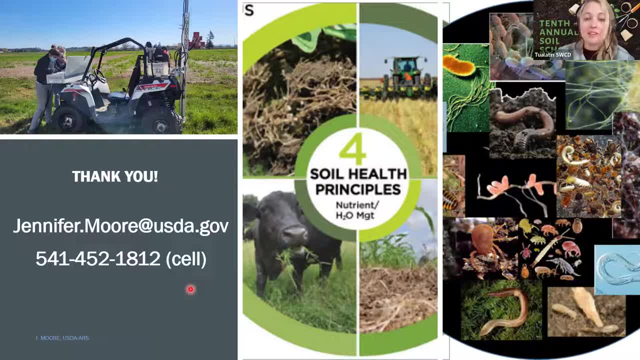 could provide a resource that would be really helpful to folks that are interested in the field, For folks that are not gardeners and not farmers. a lot of people here are telling people about how important living soils are, especially for sequestering carbon, And so, if you can provide, 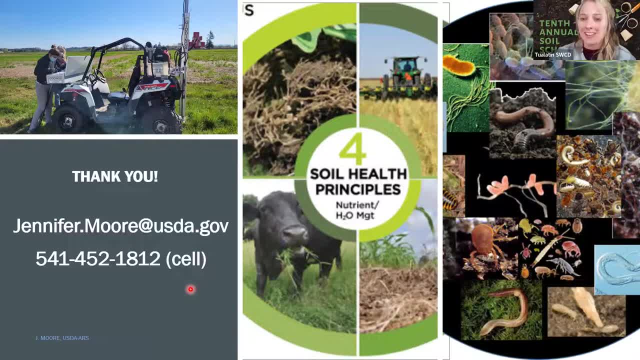 suggestions in the slides about where non-gardeners can learn about this subject and kind of just get a taste for the magic of soil that we're all into. Yeah for sure If it's about carbon sequestration and climate mitigation, that kind of thing. 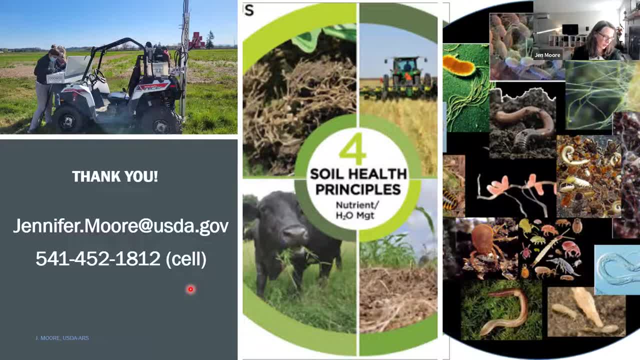 what I was with NRCS- myself a scientist from NRCS- and, oh my gosh, the climate hubs. I'm sorry. We put together a really nice four-page document that links soil health to climate mitigation in the Pacific Northwest, So if you please help me, remember to send you. 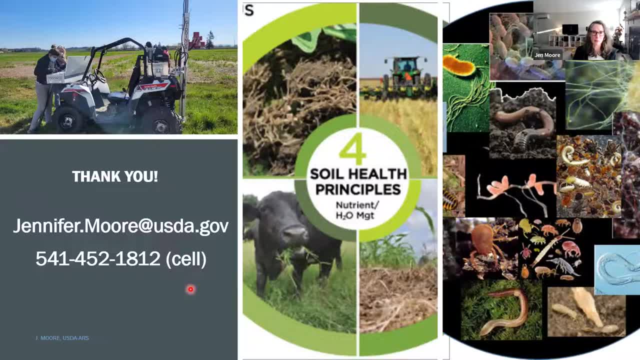 that link. I can definitely do that. I think it talks a lot about the impact of climate mitigation, about it pretty high level, and talks about the implications and why we want to employ these. Pretty much anything we do that builds organic matter in the soil. half of organic matter is 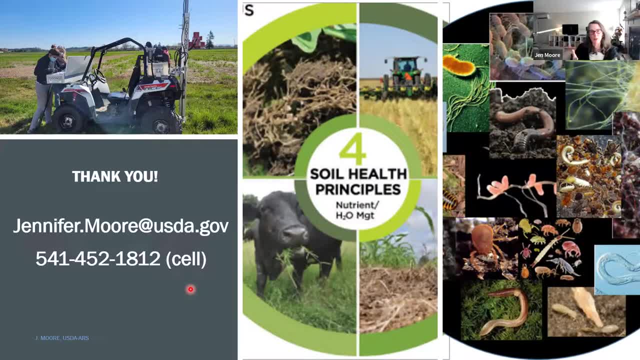 carbon, And so if we're making more organic matter, we are storing more carbon in our soils. The trick is to keeping it stored, And then I'll just say that it's not only storage, because if all of the carbon was stored in soil, then none of it would be available for microbes. 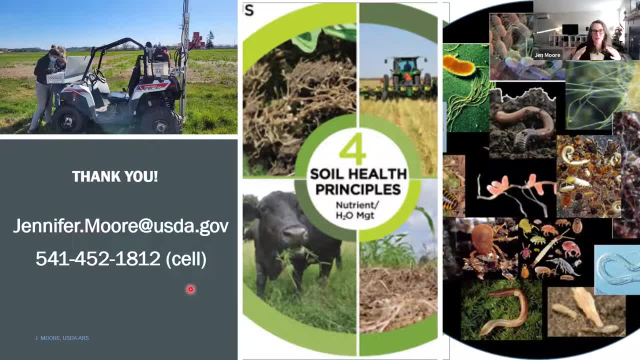 And so the holy grail is to manage carbon, the flow of carbon, while increasing that long-term stable pool. So we want to kind of balance it between the two. We don't want to hoard it all, because then otherwise the whole food system would collapse, But we want to increase it just enough. 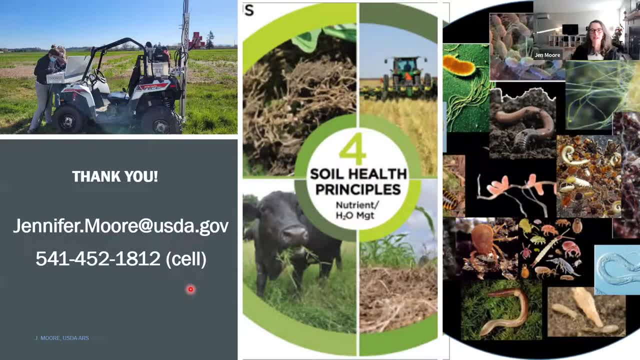 while we're kind of cycling. Okay, I'm going to try to combine some of these questions so we can get through the rest. Someone is asking about beneficial insects, and I'm going to actually refer them to our website for that one, because we have a beneficial insects webinar coming up actually very soon. 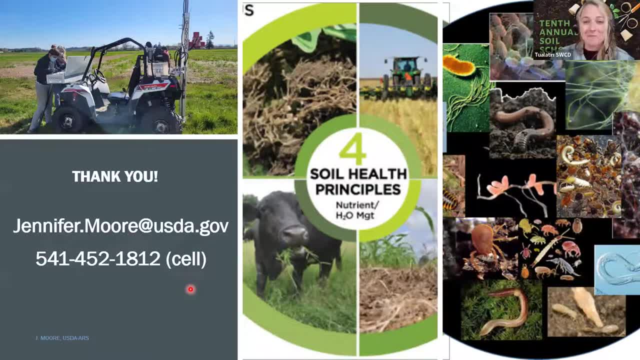 So go to our website and go to the same page that you found out about this. I can send the link in the chat, But definitely sign up for that. Thank you, Our beneficial insects workshop. we will teach you how to attract them to your property to take care. 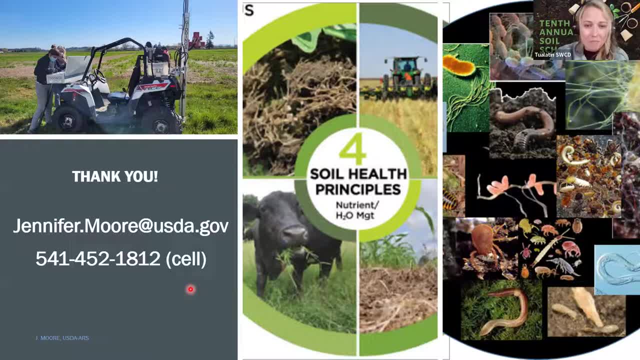 of pests. Okay, And then a quick. if you could give us a quick answer on this, although I'm sure you could go into more detail- How deep do you go into the soil to have that be considered tillage? So, if you're mixing your cover crops into the soil, is it just like a couple inches, Is it? 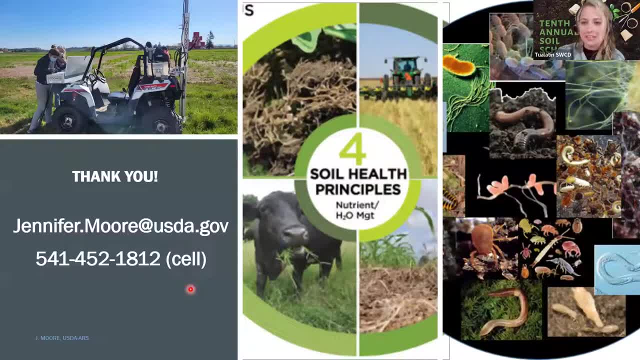 like six inches. How do you cross that threshold? Well, any tillage is tillage, but the impact of that tillage depends on how you do it. So, like a moldboard plow literally flips the soil upside down. It takes that, you know, six to eight inch chunk in it and it flips it. It's very disturbing. 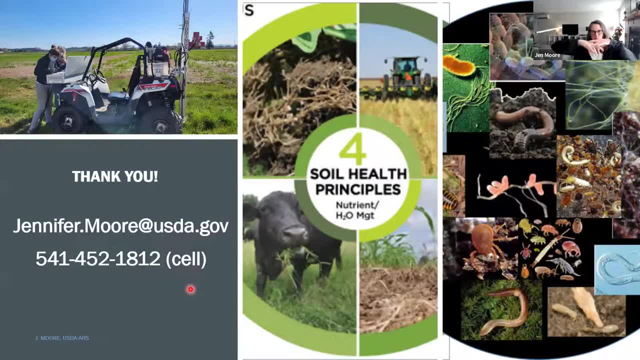 Whereas some of the more there's like for gardeners, there's like more of a rotary one that kind of does this action and it only goes a little bit To the surface. it's still disturbing, but it's not as disturbing as you know. it's like taking 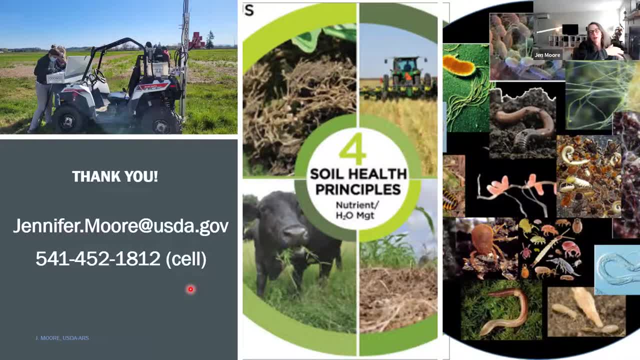 a bulldozer right And just demolishing your house, as opposed to like a tree falling on a little section of it that you can repair Right. And so if you think of the soil as like the foundation, you know how much you disturb it is gonna, you know, make an impact on how long and 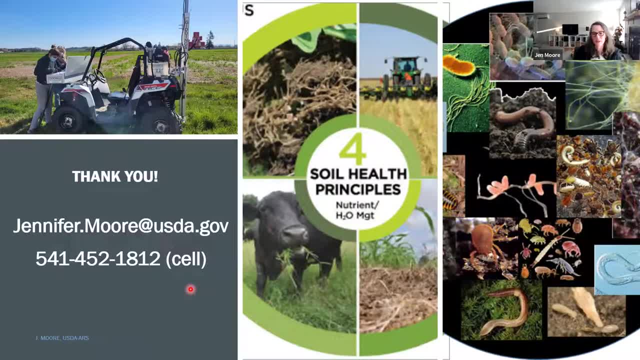 what's it going to take to rebuild it, kind of thing. Is that, is that quick enough? Yeah, I think that's great, All right. Last two questions- Both were upvoted, So important for folks. One: can you provide key elements at making? 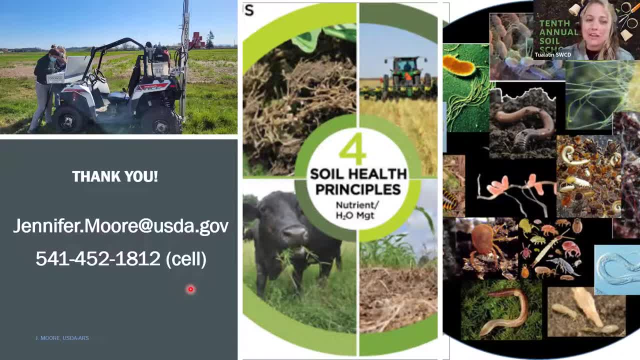 home compost and what is one item you would add to improve your soil? Organic matter compost is is is a great tool, but really you could do it through cover crop, Like it's a living cover, it's a living mulch, It's a living compost right. 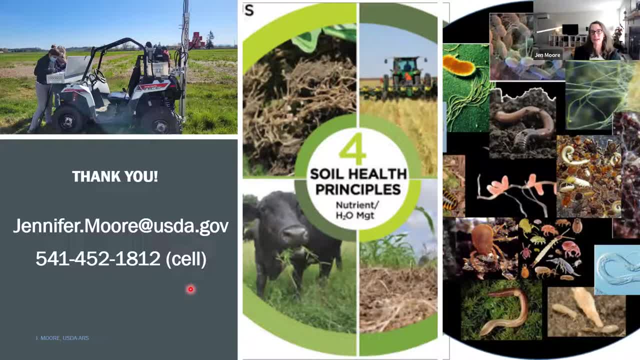 I can't tell you I'm actually a really horrible composter. I- our city, does you know municipal composting, and so I let the professionals do it. There's great resources out there. I could definitely provide some resources, if I'm sure you guys probably have some through the conservation. 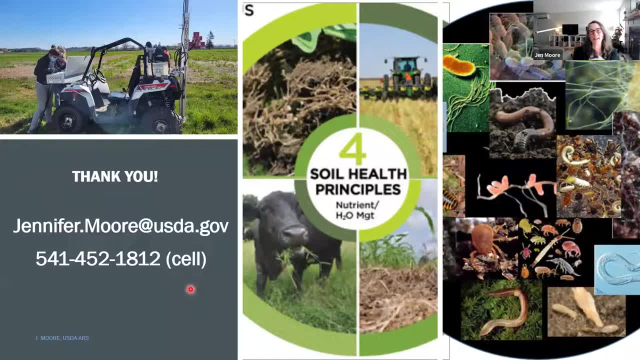 district. but yeah, I mean, it's all about. it's all about you know creating new things and you know bringing back the knowledge and knowledge that's given to the planet. you can, you can out, balance and, and you know you think i'm like a, i'm this awesome scientist. right, that should be. 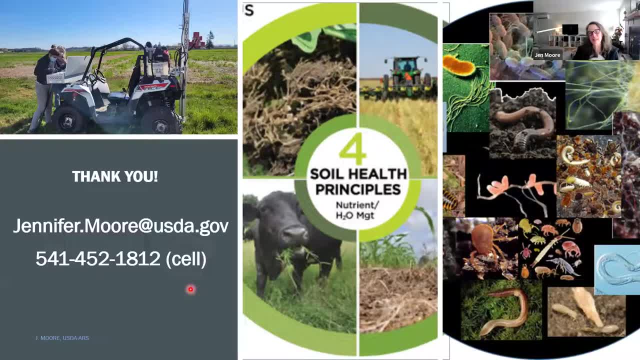 able to, and i could if i put the time into it. but, uh, between kids and work and everything you know, it's just not happening. so you are, you are a soil explorer. that's how i like to think of scientists. y'all are out there forging the way into the unknown. uh, yeah, i say, anytime you can, you can. 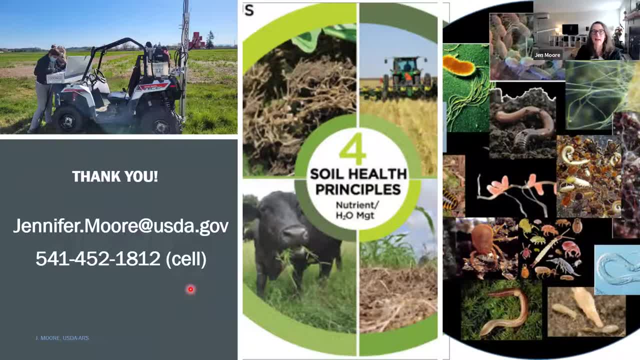 have it grown and done for you on site. it's one less step too. i'm also a little bit lazy when i garden, and so if i can grow it and then like, let it decompose naturally on the surface- um, that is the. it is compost in a sense, you know. um, that's a company. 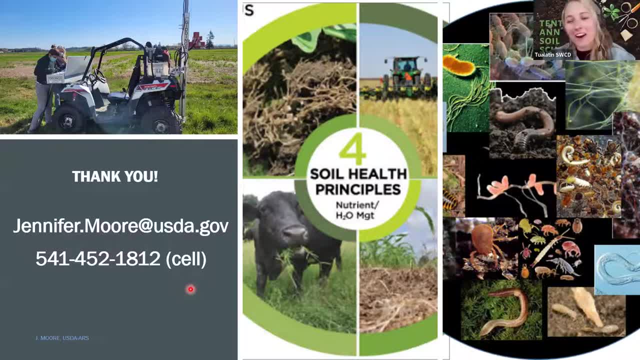 uh, so we are uh, just at seven o'clock. i want to thank you so much, jen, for joining us today. i'd also like to um thank everyone who tuned in Lots of great questions, Some of them it's hard to answer because it really depends, but I will follow up with the presentation and some other. 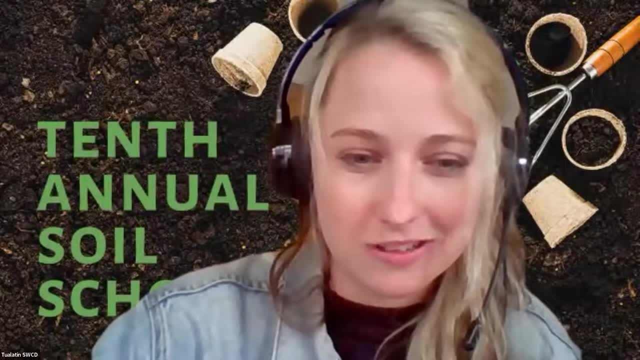 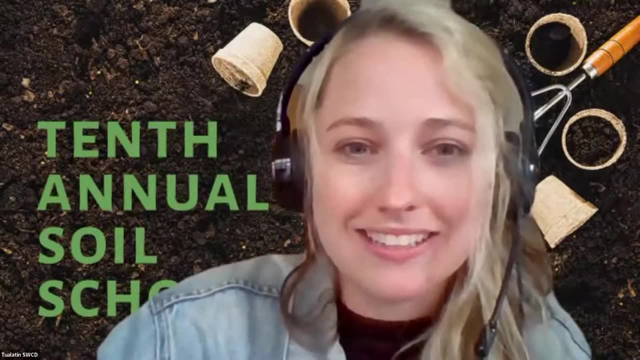 I've been taking down notes. Hopefully we can follow up with all sorts of resources that will help you guys, And in the meantime, please check out our website. In the chat there's a bunch of links to our website. We have all sorts of great resources, like how to make a compost bin and 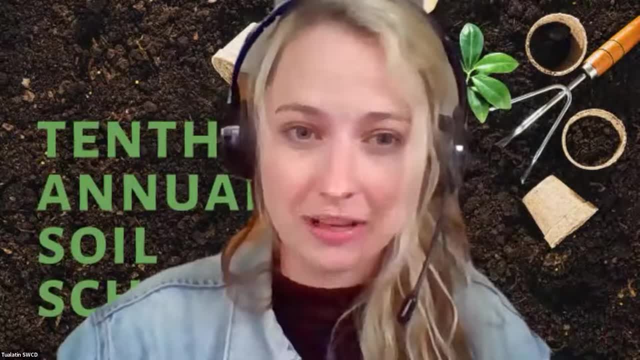 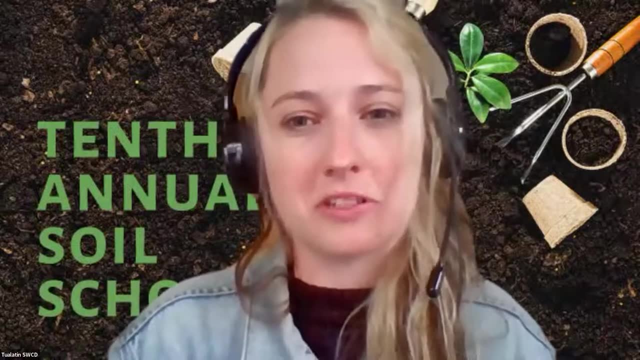 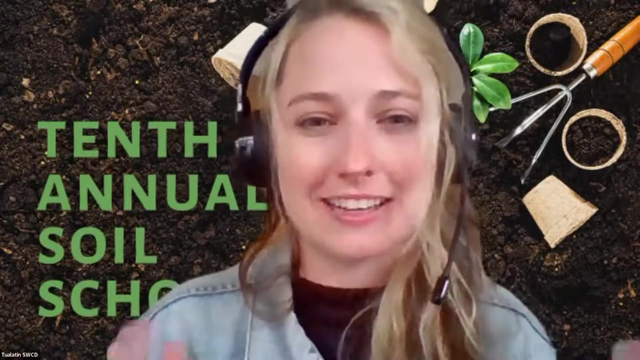 learning about soil. So if you have friends and family that just kind of want to get a little bit of an introduction to soil health, that's a really great place to go. And for your deeper soil questions, please contact Jen or contact us at Tualatin Soil and Water. We are here to help you. 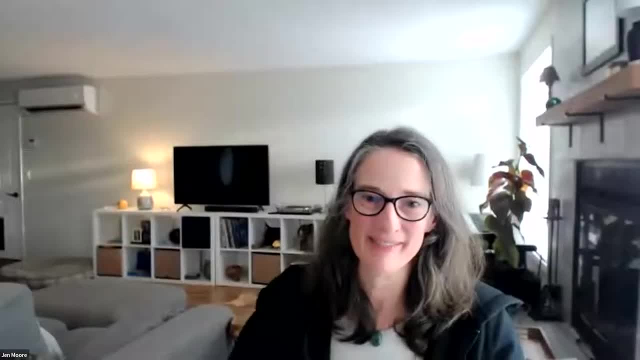 So thank you so much, everyone. Thank you, Have a good night. 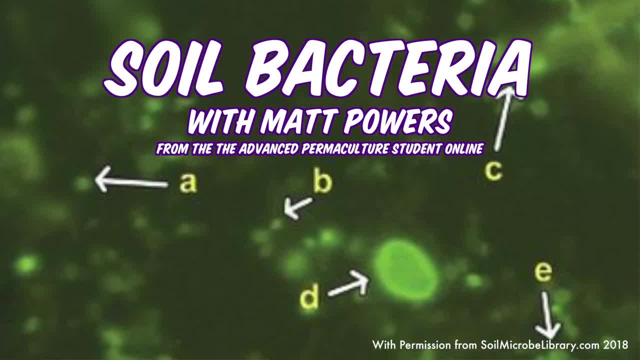 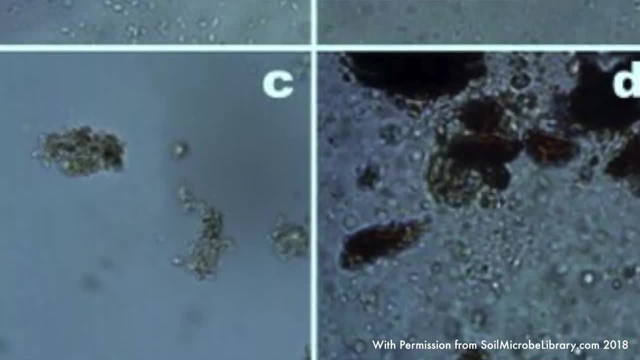 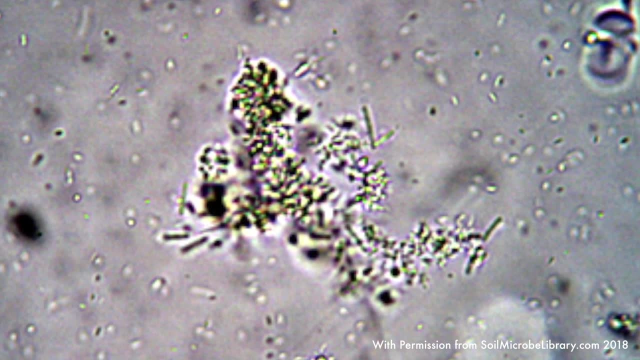 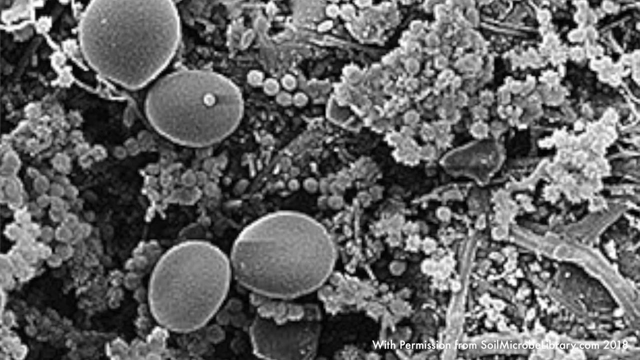 It begins with bacteria. Bacteria is really incredible because bacteria creates these glues that holds the soil particles together and these form the micro aggregates that later on fungi ties together and creates the macro aggregates, the structure of the soil. So first it's these bacterial glues. Bacteria are single-celled organisms. Bacteria is on everything. 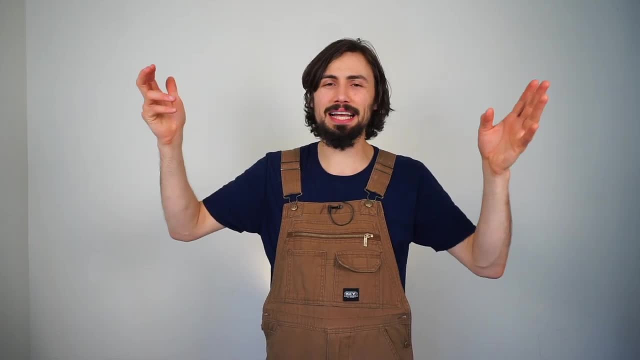 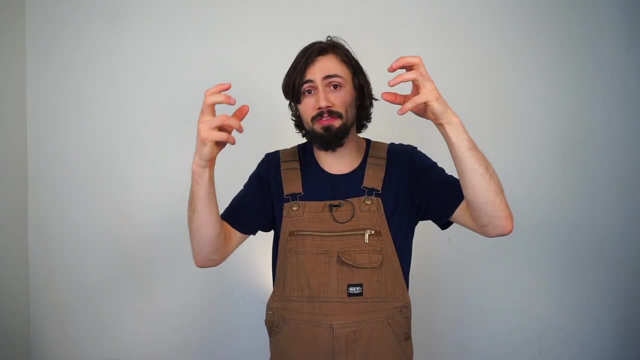 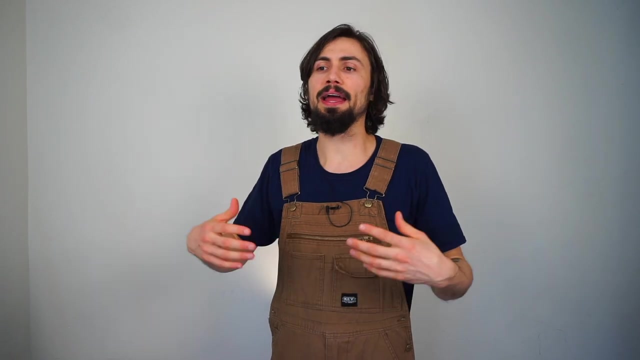 It's everywhere. It's all over the surfaces, all over our bodies. It is feeding on simple compounds, feeding on mostly simple sugars on the plant surfaces. They're feeding off of exudates and they're taking all of those exudates into their bodies and they're exchanging with all. 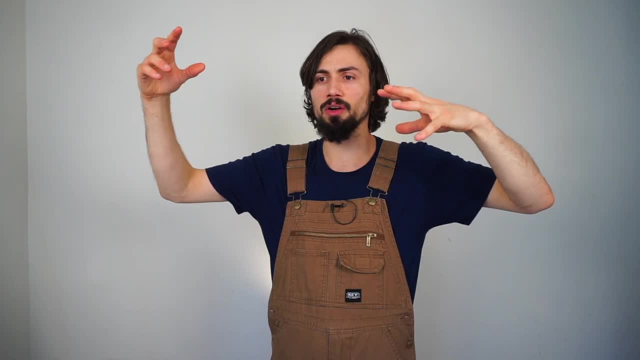 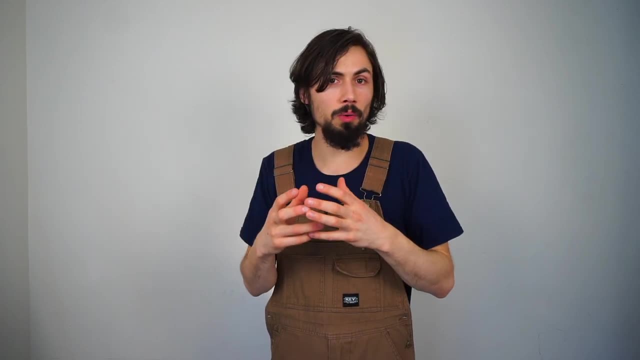 sorts of life They're consuming. consuming, They're taking it all in and then embodying it. Now they don't give it up. They're like this: you know the black box. They've got it all locked in. The bacteria is. 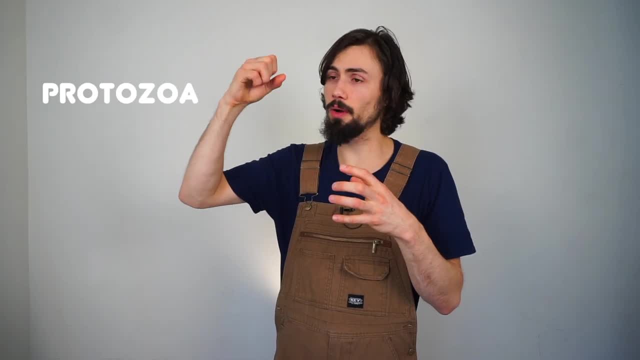 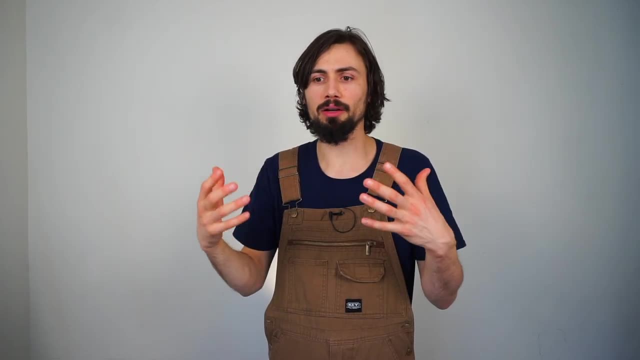 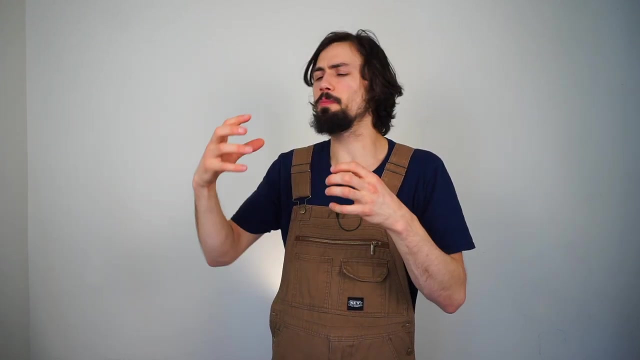 holding all those nutrients. Now protozoa comes and consumes them, because protozoas do not need all that NPK, micro, micro trace elements and nutrients that are inside. They release it in their waste. So protozoas are the first, And there's amoebas, flagellates and ciliates. 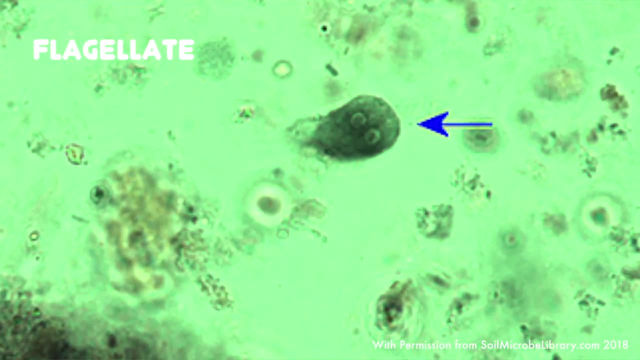 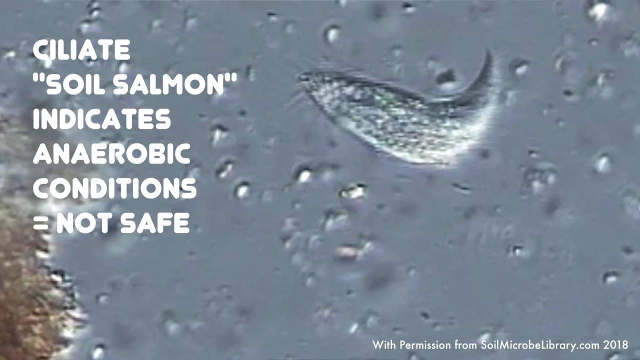 Ciliates are the bad ones. They're going to be consuming this and they're going to be releasing all these awesome nutrients- Macro, micro and trace elements- And then that can return to the plant. You need all the trophic layers because they've 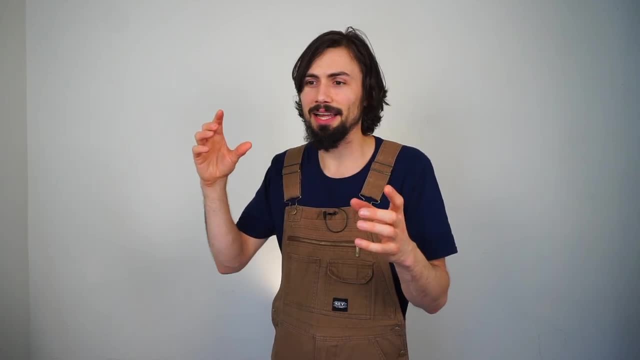 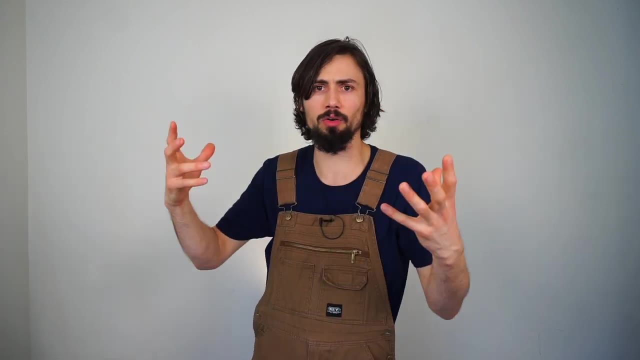 been tests done, Elaine's done- Where you just isolate these things and they either don't work or only half work if you just take out pieces. You need them all for it to be this symphony orchestration of amazingness, And so you want all the members in there, You want, you know, the